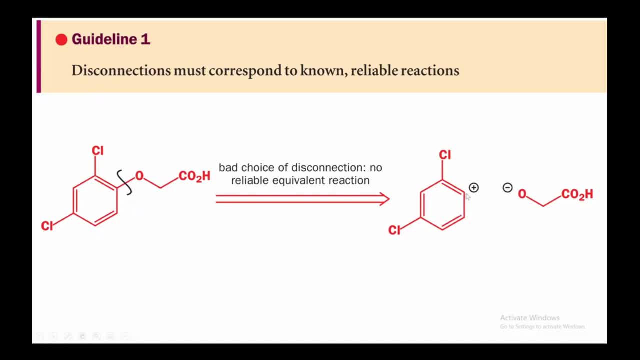 that will generate a positive charge on this benzene atom and a negative charge on oxygen. The negative charge on oxygen is perfectly fine, There is nothing wrong with it, But the positive charge on benzene is something unusual, right? Because then you have to have electron withdrawing groups strong. 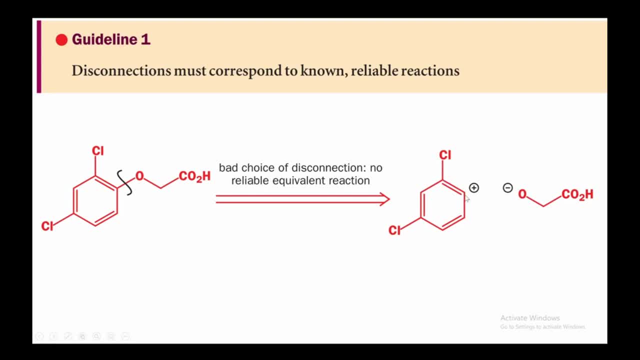 electron withdrawing group in order to put that leaving group on benzene then undergo a nucleophilic substitutions. But under normal conditions such as this, this is very bad choice of disconnection. not a reliable equivalent reaction. Alright, so you need to remember. 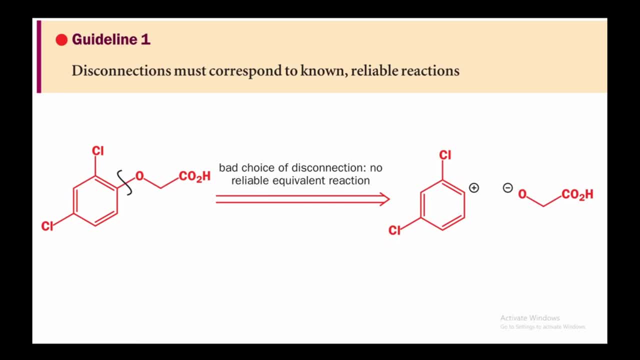 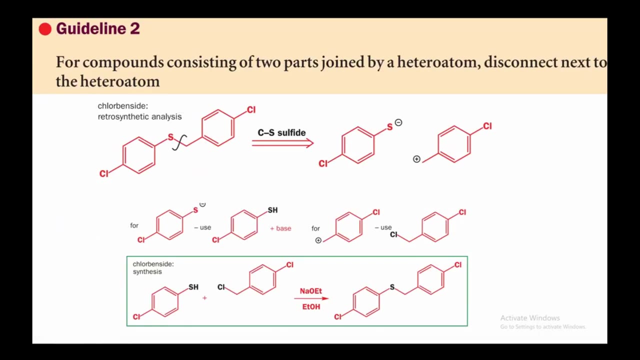 whenever you do retrosynthesis, you should disconnect from such a position where you end up with a known, reliable reaction. Okay, let's have a look at another example. So that is the guideline number two for compound consisting of two parts joined by a heteroatom. 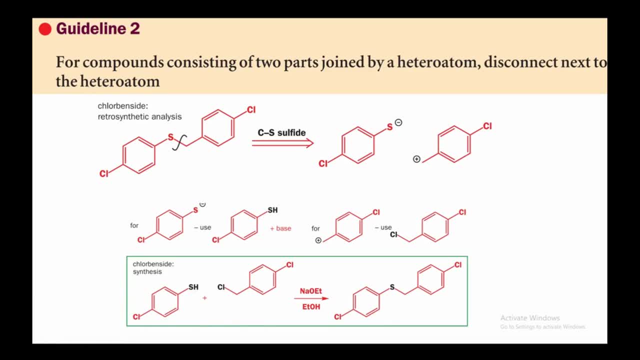 disconnect next to the heteroatom. So what is a heteroatom Other than carbon and hydrogen? all of the elements are heteroatom, For example, nitrogen, oxygen, sulfur. these are called heteroatom. So in this case, sulfur is a heteroatom. So you are disconnecting from the heteroatom. 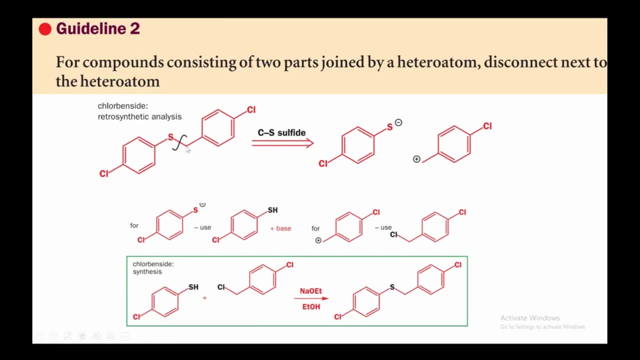 position so that sulfur is making bond with this carbon. This is a heteroatom, so you are disconnecting from this carbon, So what you need to do is to connect these two parts together and, of course, the disconnection of this position is called the CH sulfide, and the sulfur will get a negative charge. 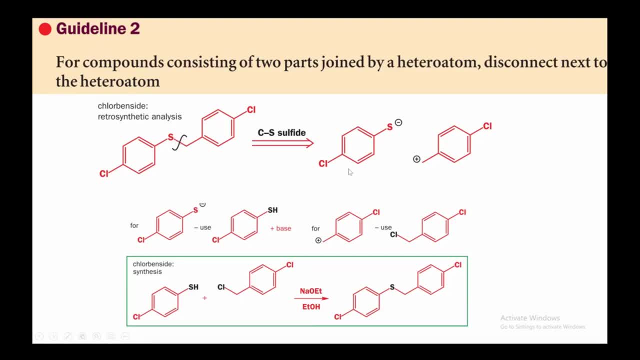 and this carbon will get a positive charge. So in this case these are called the centons and we need to find reagents or synthetic equivalents for these centons. So negative charge on carbon, which can be a equivalent to sulfur, thiol sh, and the positive charge. 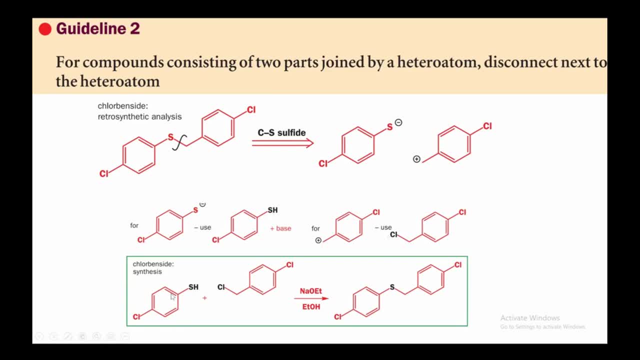 on this carbon is equivalent to this chlorine. So when you react with this, this compound, with this chlorine, you can use a base which will generate a negative charge by deprotonating the sulfur, and then this negative charge will attack on this carbon and you will get the product. so this is a forward reaction and this is a 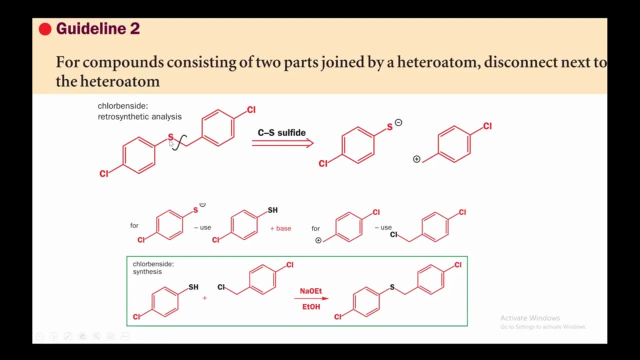 rate of synthesis. now, if you replace this sulfur with oxygen, you can use the same strategy. if you replace sulfur with nitrogen, you can use the same study. so you need to understand the concept. you cannot remember the molecules, the synthesis of molecules. you cannot remember the retrosynthesis of all the 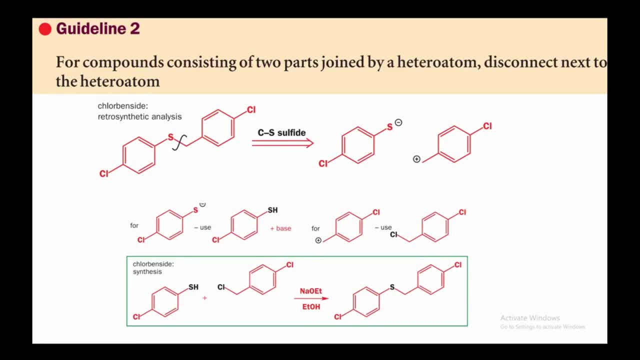 molecules that are being available in the literature. that's not how you learn organic chemistry. you need to have a method. you need to come up with a conceptual idea. it doesn't matter if you have this benzene or if you have two benzoins. it really doesn't matter. the conceptual point in this slide is that 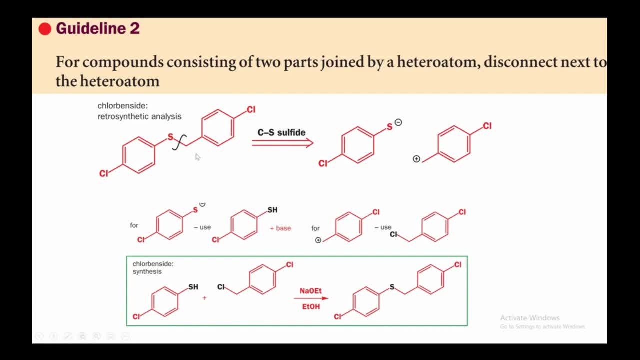 you need to understand the concept. you need to understand the concept, you need to disconnect from the hetero atom. so in this case you are disconnecting the bond between carbon and sulfur and that gives you the positive charge on carbon, because carbon is a less electronegative element and sulfur is more. 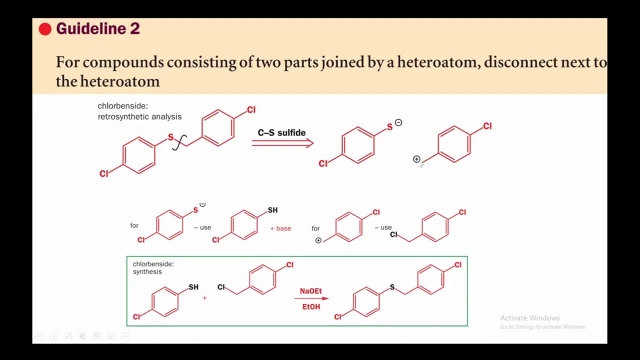 electronegative element and hence this sulfur gets a negative charge and carbon gets a positive charge. now try to find out the equivalence. how can you generate a positive charge on the carbon? put the leaving group, that's chlorine. how can you generate a negative charge on sulfur? put the hydrogen. that is the way of doing. 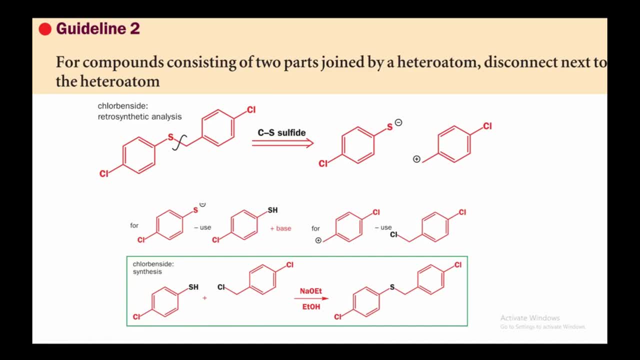 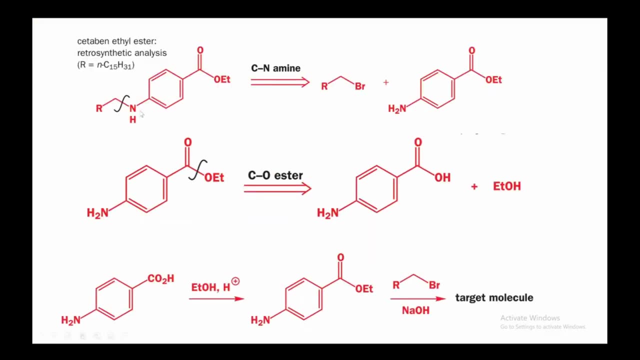 retrosynthesis. this is a simplest basic example. you need always need to do disconnection in this way. you disconnect the bond and put negative charge on one side and positive charge on one side, and then come up with the equivalence. all right, let's move on to the next slide. this is an example where you have a secondary amine on one. 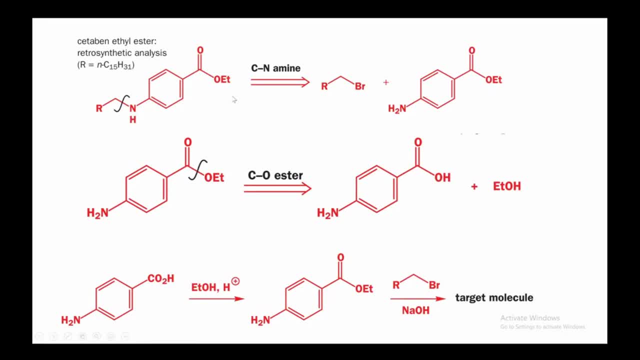 side and ester on other side. so the rule number one in retrosynthesis is always: recognize the functional groups, what kind of functional groups present in the compound. you need to target those functional groups and disconnect accordingly. so this is secondary, I mean you can disconnect the bond between 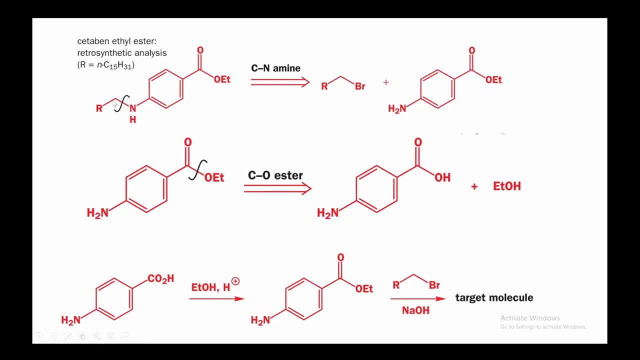 carbon and nitrogen. that is a heteroatom bond, and one side will become alkyl halide and another side will become NH2. all right, then you disconnect ester. so we have a simple CO ester disconnection. you disconnect this bond and then one side will become ethanol and other side will become carboxylic acid. how you can? 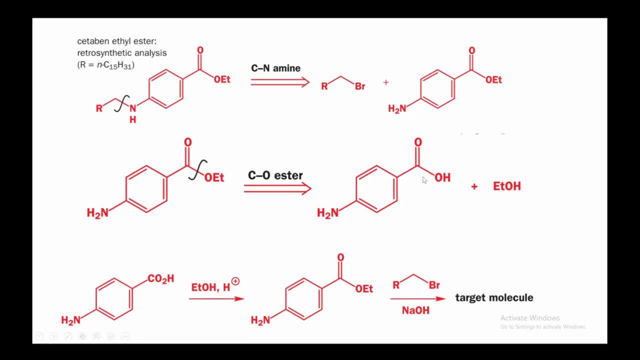 do this, but just remember how we can prepare esters. okay, esters can be prepared when carboxylic acid reacts with the ethanol. now think about forward direction reaction. we have NH2 and we have acid, so you react this acid with ethanol in an acidic 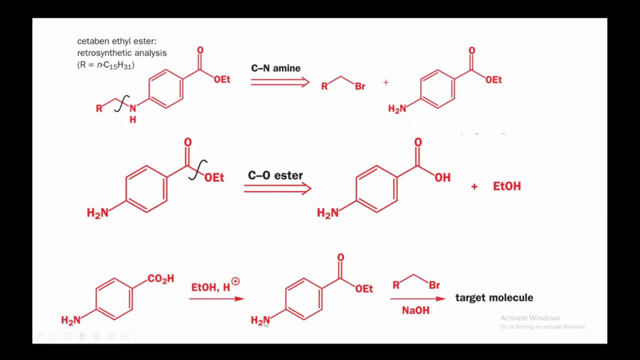 media. you get the ester and you have an NH2 group. now this is a nucleophilic position. you react this with alkyl halide in the presence of a base. you will get the target molecule all right. so this is the approach. this is the 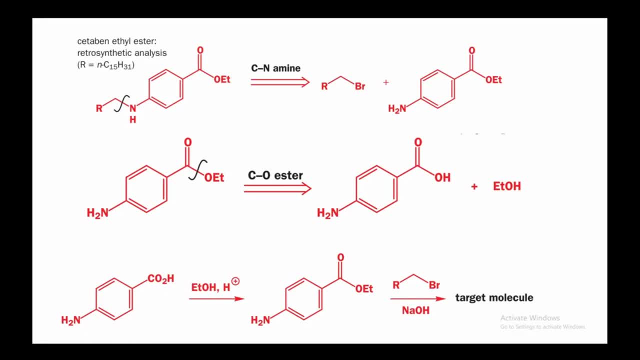 method. this is a strategy that you should follow when doing the retrosynthesis. now, whenever you see an ester bond anywhere in the questions given to you in the exam or entry test, you must- must- follow the strategy of disconnecting the ester. it doesn't matter how other groups are connected to. 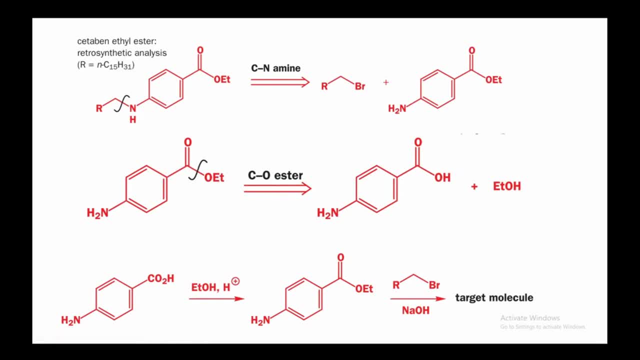 it. you should follow this pattern. you should follow the concepts, how you disconnect the secondary amines, how you can disconnect the ester functionality. in this slide you have learnt the of secondary amines and disconnection of ester. let's move on. okay, sometimes you are given a 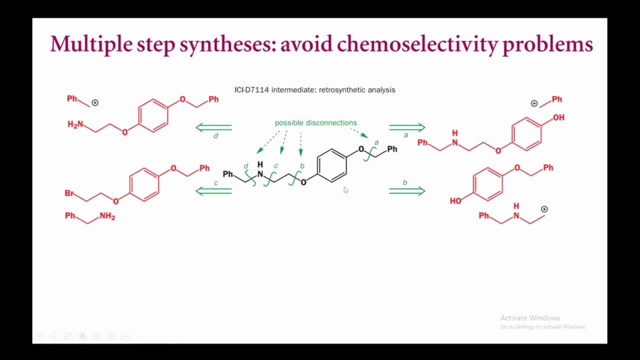 complex molecule and there can be multiple starting disconnections or possible disconnection, like a, b, c and d. now you have to pick which one will be better. so in this case, multi-step senses avoid chemoselectivity problems. what by chemoselectivity? so selectively reacting at the 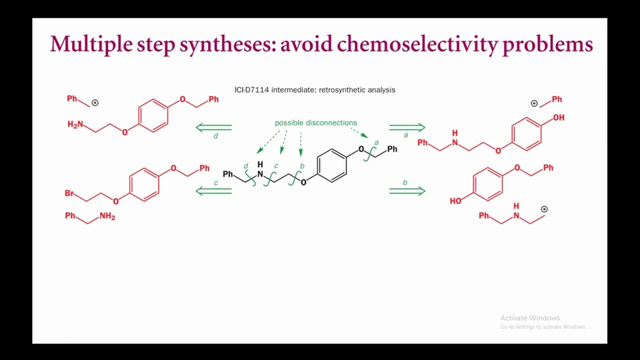 one functional group or one point and avoiding and not interfering other functionalities. so if you look at the disconnection a, that corresponds to the positive charge on this carbon and phenol on this benzene, if you see the disconnection b, that is phenol on the this benzene and the 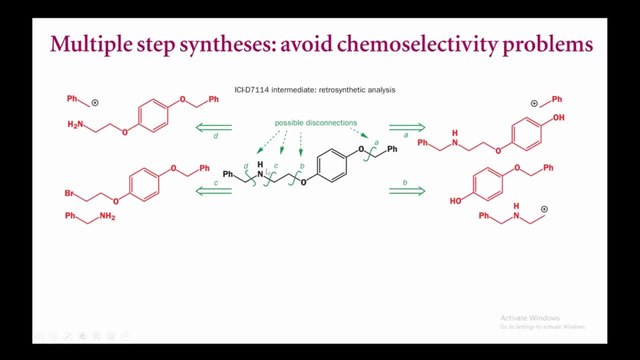 positive charge on this carbon, disconnection d, which disconnects from this carbon nitrogen bond and corresponds to this, and disconnection c, which corresponds to this one. now, the rule here is you should disconnect such a bond which is most reactive first. so there are four disconnection possible, but how can i proceed with which disconnection is correct or? 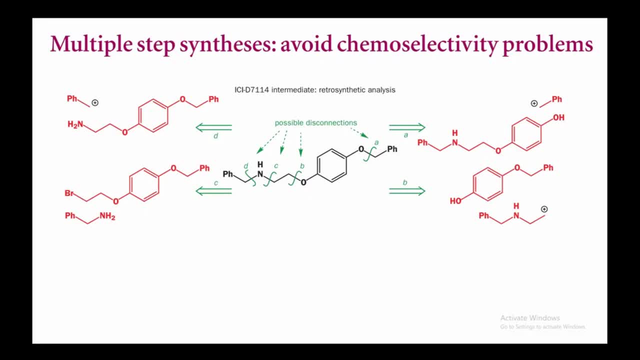 which disconnection is most suitable. according to the retrosynthetic strategies, disconnect that bond first, which is most reactive. so this one disconnection will be most plausible, one which gives you the this disconnection, that is, which gives you this one disconnection see it's most. 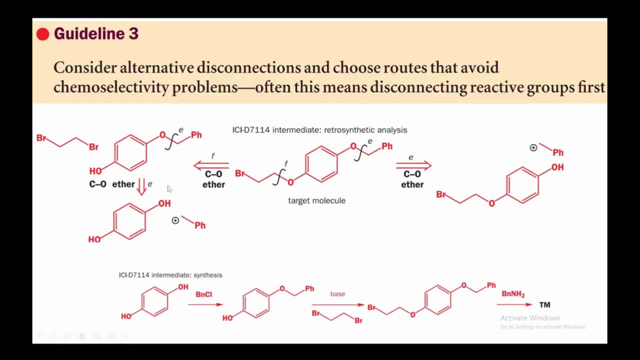 suitable one. now you can proceed either. II are in the F direction, so F direction is much more reliable. as you can see, in E we are disconnect the CO ether bond and you will get these syndhones. but if you disconnect from the position f you will get this time alkyl allied and ether and alcohol on. 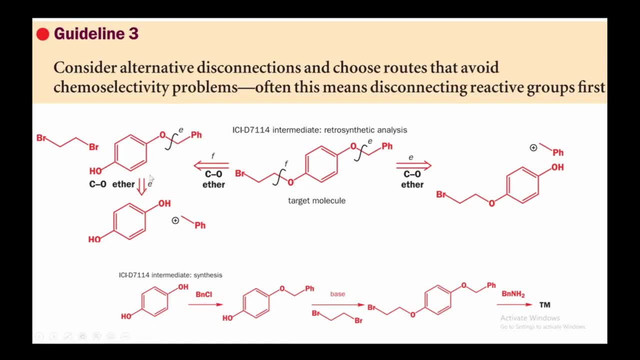 this side, then you can disconnect this position between carbon and oxygen. that will give, that will give you the phenol, di phenol 1, 4 by substituted, and this phenol the positive charge on this pencil position. now, if you look at the synthesis, the forward direction, retrosynthesis is a backward and 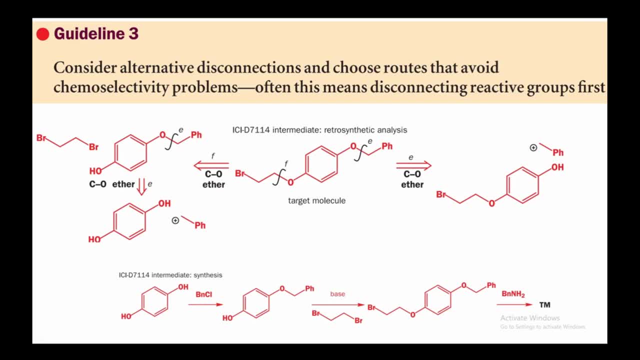 synthesis the forward. so you start from this easily cheap starting material: 1 4 di phenol, and then you react with BMC, lbm cell is final ring ch2 steel. okay, that's called benzoyl chloride. so this is a simple SN 2 type nucleophilic. 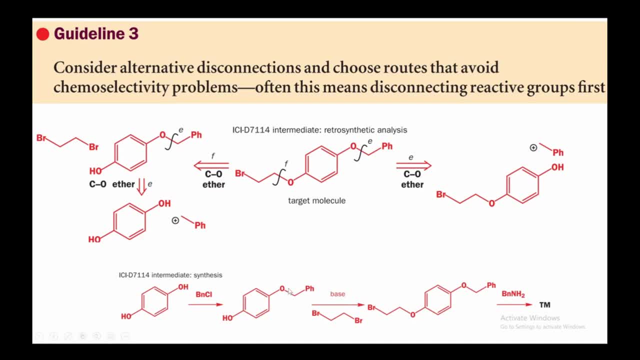 substitution, you get the formation of ethers and, in the next step, also based deprotonates, this phenolic hydrogen, and gets the negative charge there. this negative charge attacks on one of this carbon and gives you the ether again. and this next step is benzoyl amine, the NH 2 being nucleophilic and this carbon being 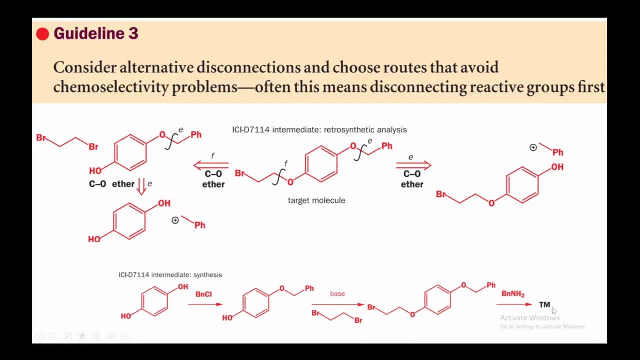 alkyl halide undergoes SM 2 reaction and which will give you the TM that is target molecule. so the point of this slide, the point of this showing the molecule, was that the consider alternative disconnections and choose the rules that avoid chemoselectivity problems. often this means disconnecting a 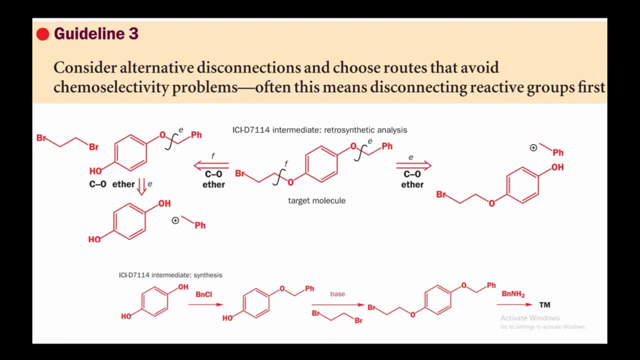 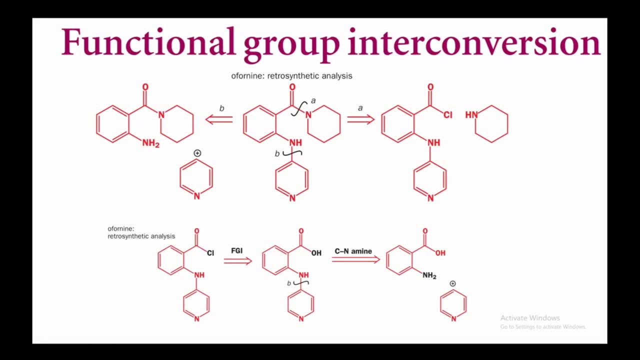 reactive group first. okay, I hope you got this concept. let's move on to the next slide. all right. next strategy in retrosynthesis is a functional group interconversion. okay, sometimes you cannot disconnect directly. you need to convert one functional group into another in order to reach towards the simple, reliable reagents. 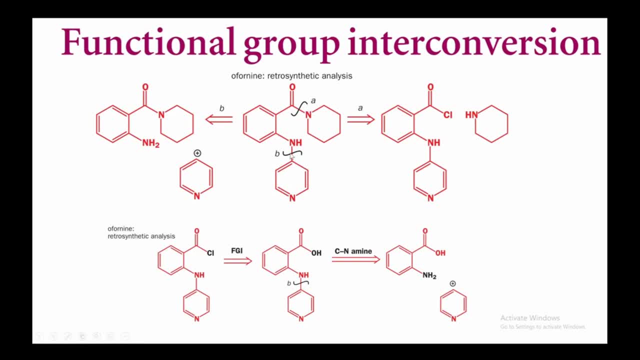 so disconnection a is possible, disconnection B is possible. disconnection b seems to be a bit difficult one, because you directly generating the positive charge and periodine. what you need to do is disconnect this amine functionality, so one side will become acid chloride and another will become the L mean. so it's a simple reaction of 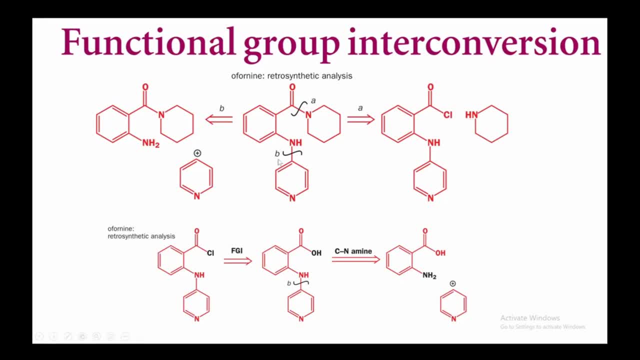 walking active charges, then we can disconnect. the amine functional group, then we can disconnect. need to have di. then what you can oder able to, if you can disconnect add示 connect. then you do FDI convert to ANZ and the same obligation organ, so whenб I n equal to sample ah. you can take these negative Clint from it and convert to another normal reviews you can be limited codes you will con previous, then you can disconnect. you to amine functional groups, then you can disconnect. then you do FDI convert into other normal Direction, then you can disconnect. then you D. 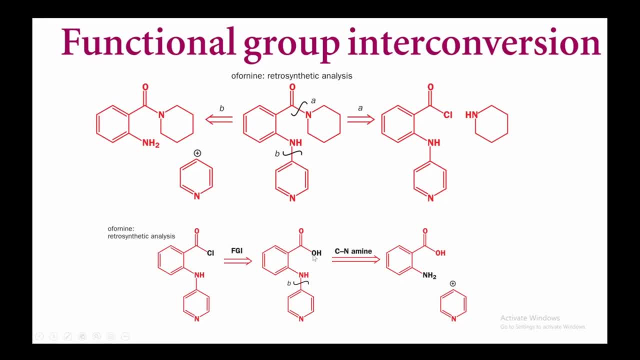 convert this acid chloride into acid carboxylic acid, as carboxylic acid and acid chloride are derivatives of each other, so they can be interconverted, they can be prepared from one one another. and then you disconnect this B, that is called a, C and amine disconnection. now you will get a positive charge on 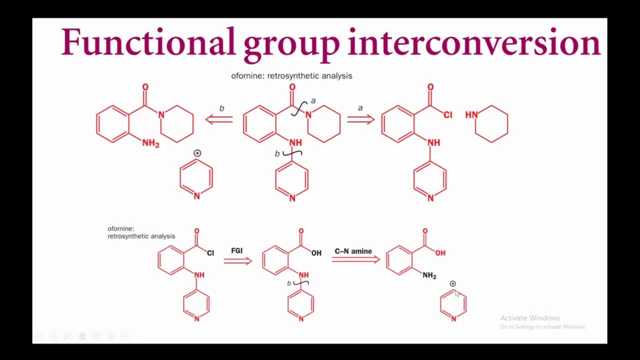 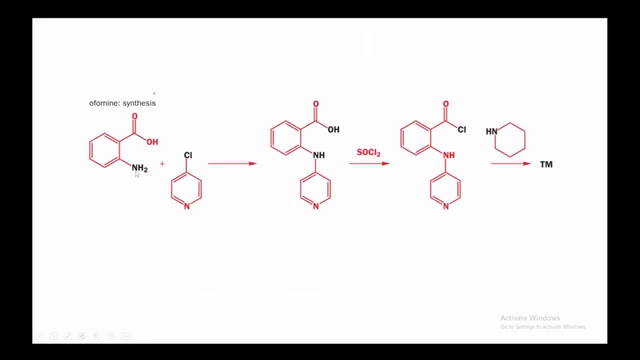 benzene, that where. that's where you can put the leaving group. that means that that's where you can put the chlorine or bromine. okay, let's have a look at the synthesis. so you start with this. this NH2 acts as a nucleophile, attacks on 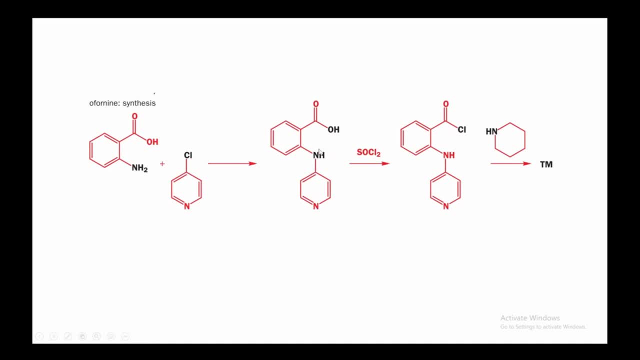 this carbon and chlorine leaves. then you have a formation of CN bond and converting of acid chloride with thionyl chloride into acid chlorides and this acid chloride rates with secondary amine to give you the target molecule. so in this strategy we learned how we can use the functional group interconversion. 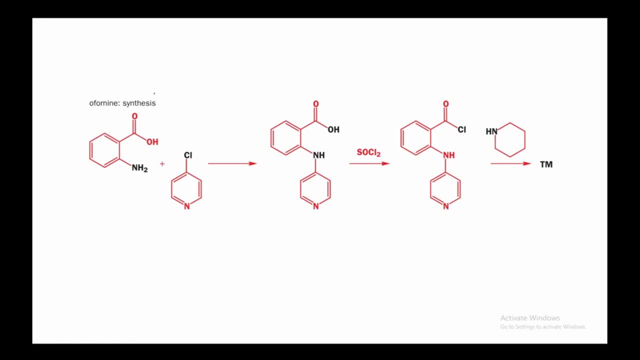 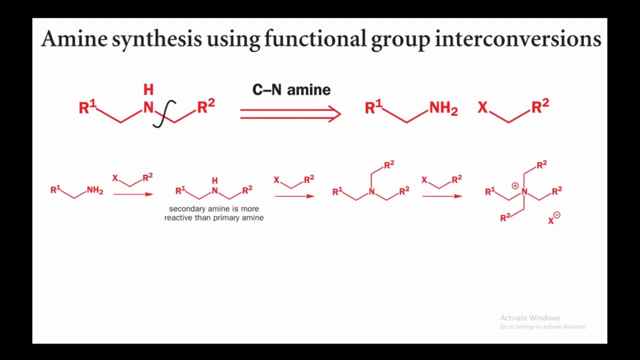 strategy in retrosynthesis in order to construct the synthetic strategy. okay, let's have a look at the functional group interconversion strategy in retrosynthesis in order to construct the synthetic strategy. okay, let's have a look at another example. this is a secondary amine: amine synthesis using functional 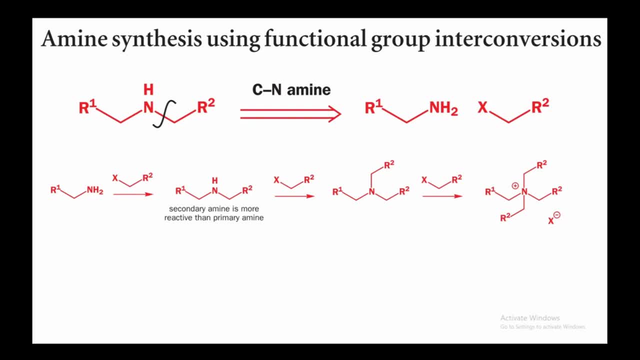 group interconversion so you can easily disconnect CN amine bond. but this is not a reliable or this is not a good disconnection. why? because this can cause several problems, such as over alkylation. what I mean by over alkylation is this nitrogen contains two hydrogens and this nitrogen is a nucleophilic in nature. if 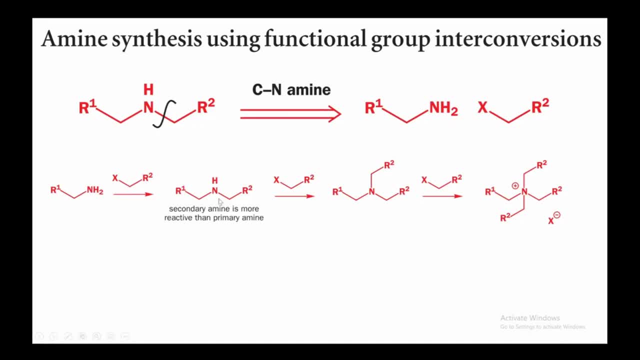 this attacks on this alkylite, you get double alkylation. I mean, and again this NH attacks on this alkyl halide, then you get a trial collated. I mean, and if this nitrogen again attacks on this alkylite, then you get a tetra alkylated. I mean, that's called quite a quaternary. I mean having 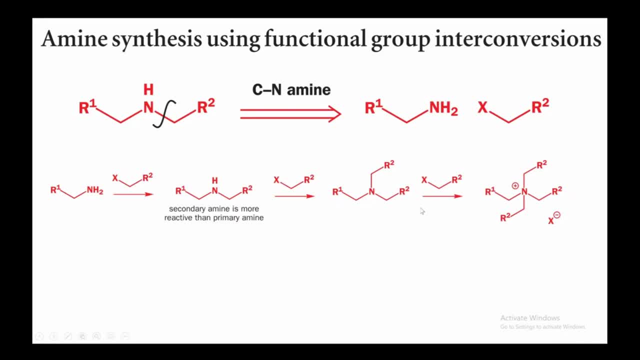 I mean having a positive charge. so this is the problem with this strategy. so avoid this strategy for amine synthesis. okay, this is not a good strategy. why? because you may end up with having more alkylated products. let's see what are the good strategies for amines. okay, this one is a better. 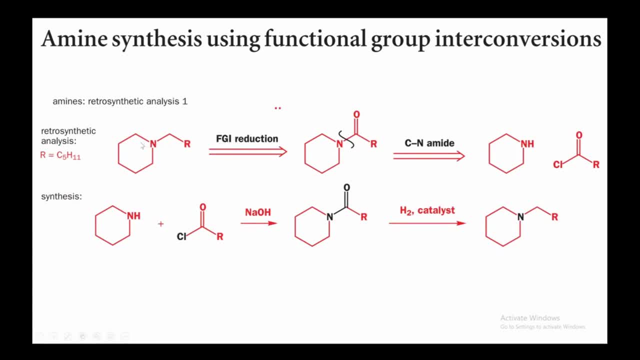 strategy, because you are doing FGI first. this is a tertiary. I mean you are converting amine into amide first and then you are disconnecting the amide bond, CN, to give you these starting materials. now this is a simple, well-known conventional reaction. secondary, I mean reacting with acid chloride. it will give. 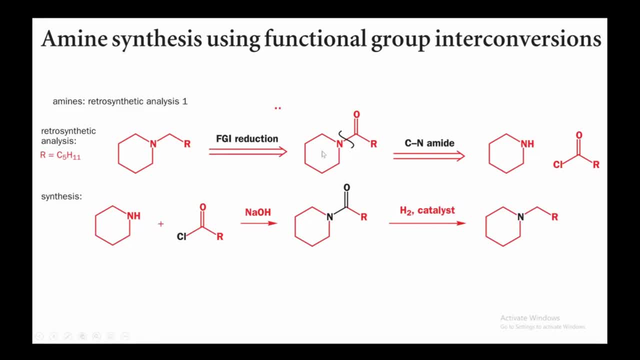 you amide and then you use any reducing agent, such as lithium, aluminum hydride, to reduce amide into amines. this is the forward direction of this data synthesis. so a mean is reacting with the acid. chloride gives you the amide bond and then you disconnect this amide bond with h2 and 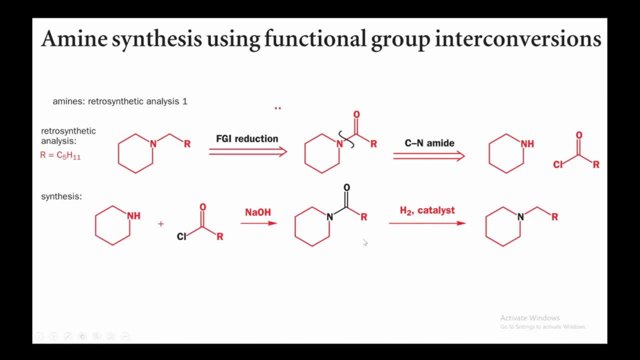 catalyst to give you the amine. so that's the good strategy for tertiary. I means, if you see it closely, this is a tertiary, I mean, so you can follow this approach now whenever you are given a big molecule or different functional deep but possessing different molecules. so you 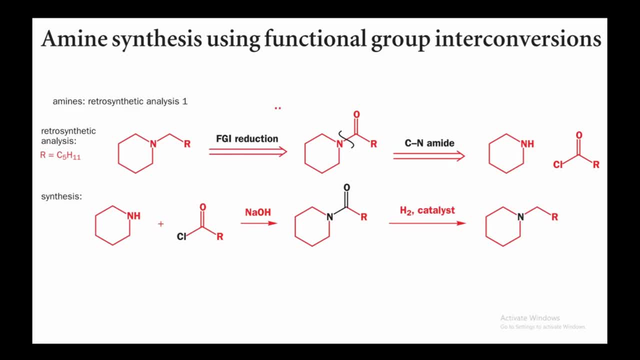 try to look out for the functional groups that are present in that molecule. so and remember these strategies you know. first you pick which functional group it is, then you try to use this approach. if it is tertiary amine, now try to use this approach using FGI: convert this tertiary amine to amide. then 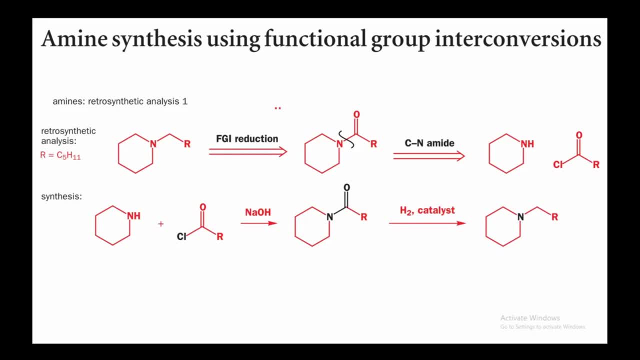 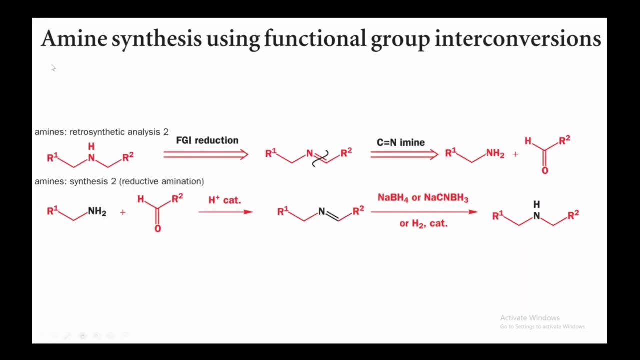 disconnect the amide bond to reach the simple starting materials. and then- this is a forward direction reaction: first reacting tertiary amine with acid chloride and then making amide, and then reducing amide with H2O catalyst. all right, let's move on to the next slide. this is again the same slide. all right, this one is. 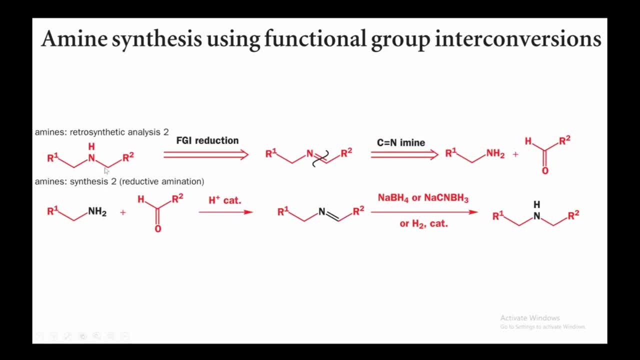 secondary amine. now this is a slightly different approach for secondary amines. what you do in this is you convert secondary amine into amines. all right, how you can convert amines into amines? just react amines with either aldehyde or ketone. then amines will be formed. that's called FGI reduction. then 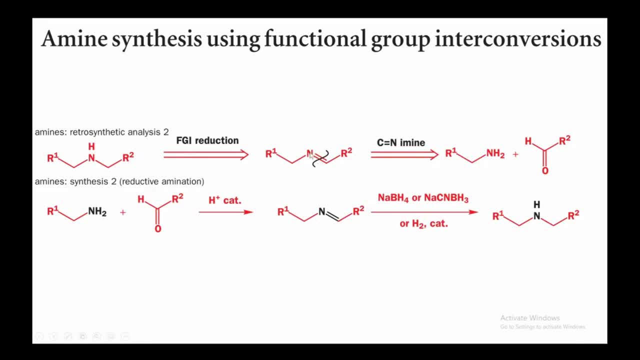 you delete or then you disconnect this bond between carbon and nitrogen, that is, CN amine disconnection, and this will. this can be disconnected into simple starting materials, amines and aldehydes. now you react this amine and aldehyde in the presence of an acidic catalyst to give you amine. then you react this amine in. 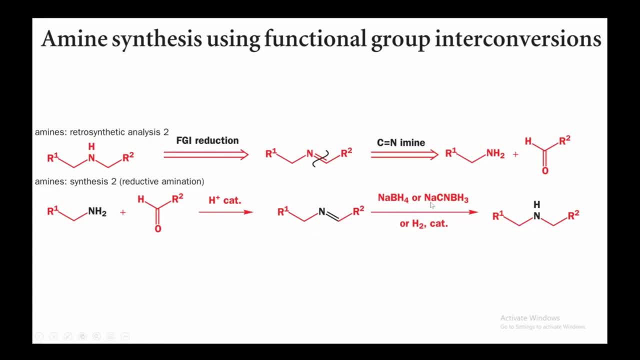 the using the reducing agent, such as sodium borohydride or sodium cyanoborohydride or H2 catalyst to give you the tertiary secondary amine. this is the approach that you can use in this case for that you can follow for this synthesis of secondary amines. so amine is a shift based formation. okay, let's go on. 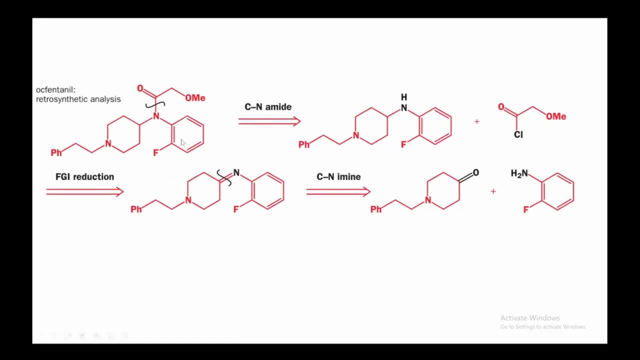 to the next slide. okay, now you have it's time to apply the concept. now you have a AMide functionality that you disconnect the AMide bond, CN. then you are ended up at secondary Pan-Amine and an acid chloride. now this is a secondary видеоonlite. you convert this into a FGI reduction. 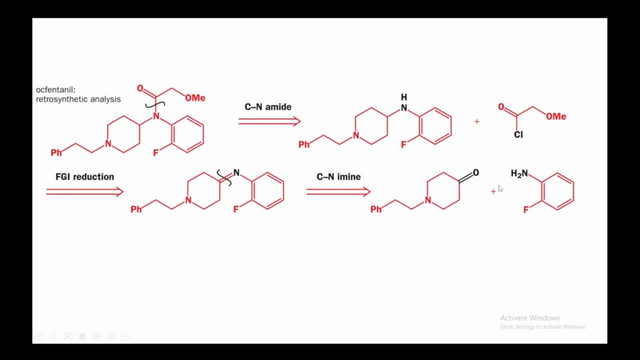 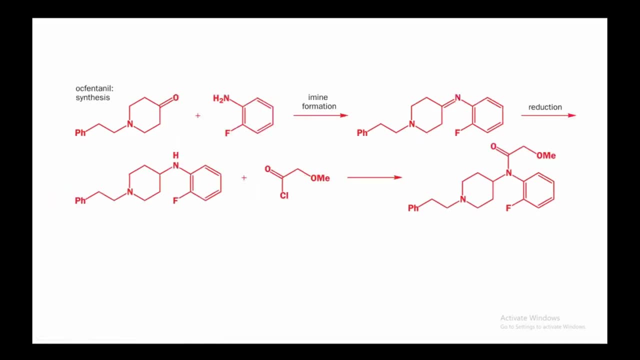 an imine, then you disconnect this bond and one side you will get a ketone and another side will you will get NH2. so let's look at the synthesis of this molecule. so this ketone reacts with this NH2. that is imine formation. that 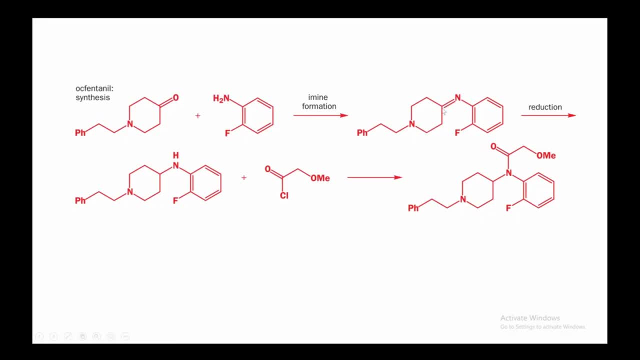 imine formation means carbon double bond nitrogen. then you reduce this double bond between carbon and nitrogen into NH and then you react this NH with this acid chloride and it will give you the desired product. so this was the applying the concept of imine formation into a real retrosynthesis. okay, let's move on. 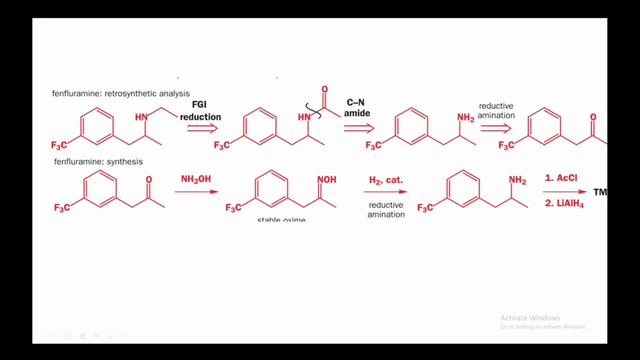 to the next slide. again. you start looking the molecule by first picking up what kind of functional group it is. it's a secondary. I mean straight away. you do FGI reduction. either go towards amide formation or go towards the amino acid imine formation. either is okay. so this is amide. now you disconnect it. you have. 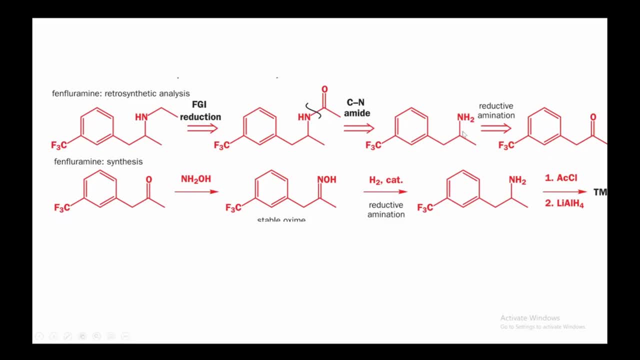 NH2. now you do reductive amination. what I mean by reductive amination is you delete this NH2 bond and put the ketone. let's have a look at the synthesis, then you will understand. so you start from this ketone, now reacting this ketone with. 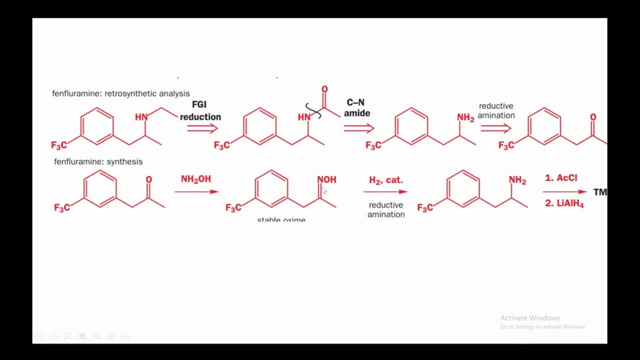 hydroxyl amine, it will give you the stable oxime. now you do reduction of this double bond- nitrogen with carbon- in a catalytic way that you'll get the NH2 that's called reductive amination. and now you are reacting this NH2 with. 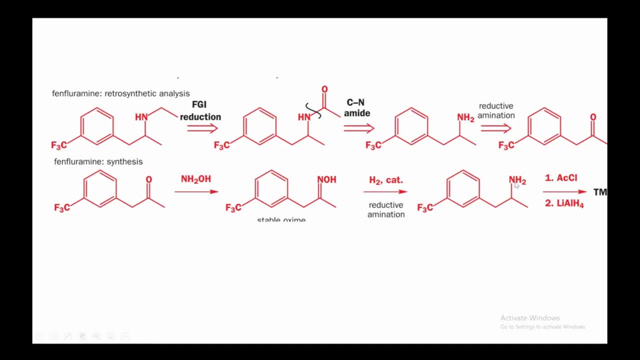 acetyl chloride, acid chloride. basically, you are converting amines into amides: number one, then in the number two you are reducing the amide to get your target compound. I hope you understood it. if you don't understand any of the slide, please drop your comments below in this video and let me know what you think of this, and see you in the next part. 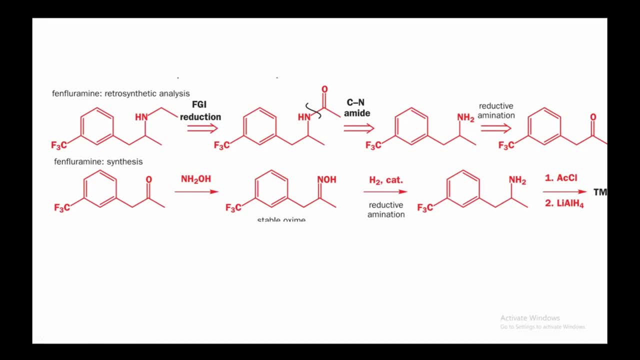 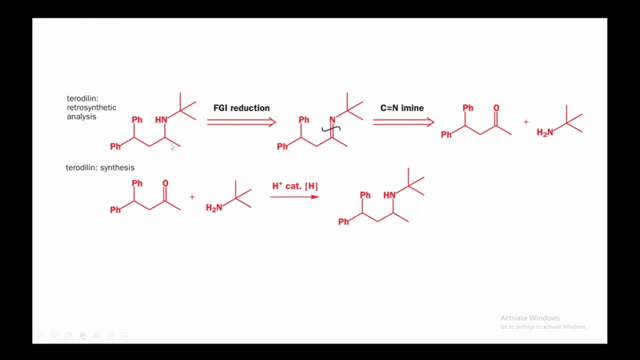 video. i will try to make video on particularly that slide. okay, thanks, let's move on to the next slide. again, you have been given this molecule. how will you do retro sensors of this compound? what you need to do is to recognize functional group. that is secondary. i mean, do you? you need 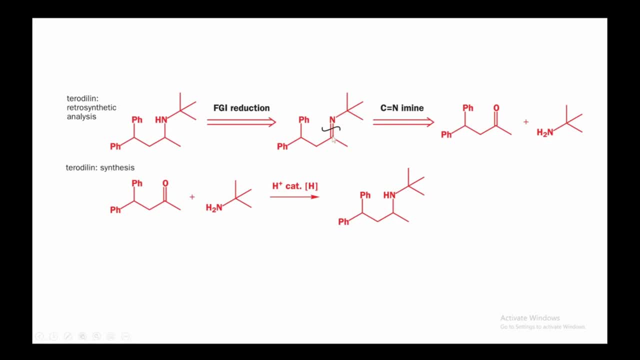 to do fgi reduction. now carbon double bond, uh nitrogen- that is immune. now you disconnect this. one part will become ketone and other part will become nh2. now nh2 and ketone react together in the presence of acid catalyzed media. they give you a immune formation. and this h in brackets. 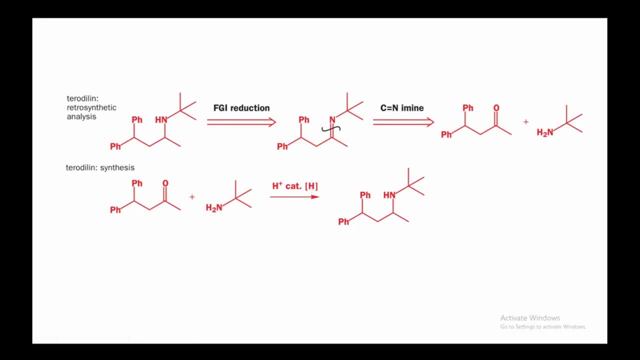 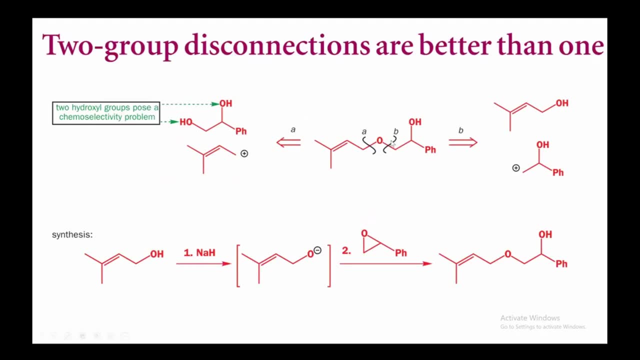 shows the reduction, and this will give you your target molecule. now let's move on to the two group disconnections are better than one. if you are given this molecule, you can either disconnect it by root b or root a, so root a will give you the down. 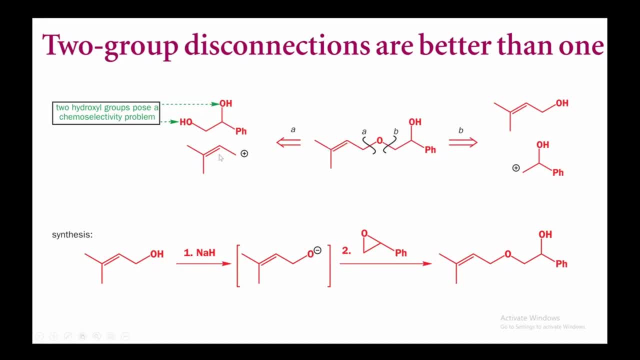 diodes like one, two functionalized and a positive charge on this one and root b will give you the alcohol on this side and this one here. you can see this is a same tone that can be used, this reagent, epoxide, because this lone pair of oxygen can attack on this carbon and it can give you the 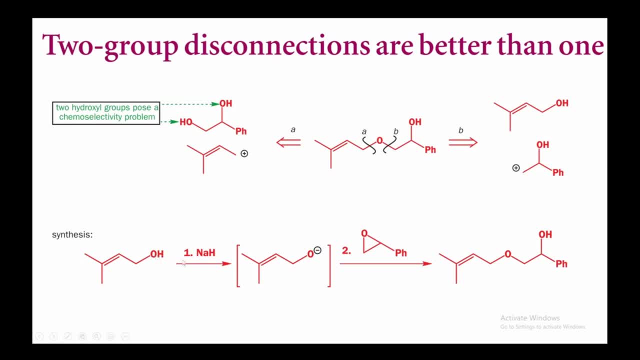 epoxide. all right, now this is alcohol. you react with a base like sodium hydride. you generate a negative charge on this oxygen. now this negative charge acts as a nucleophile and it attacks on the epoxide ring and the ring opening reaction takes place. hence you get the alcohol formation. so this: 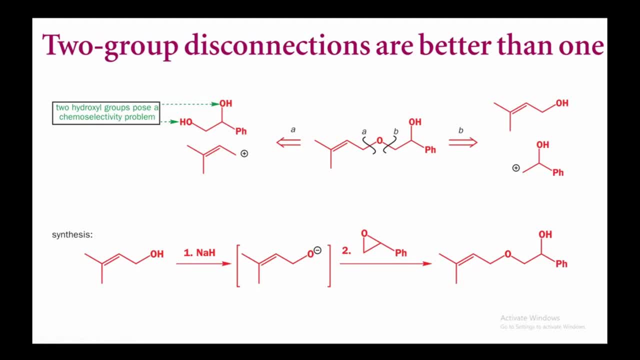 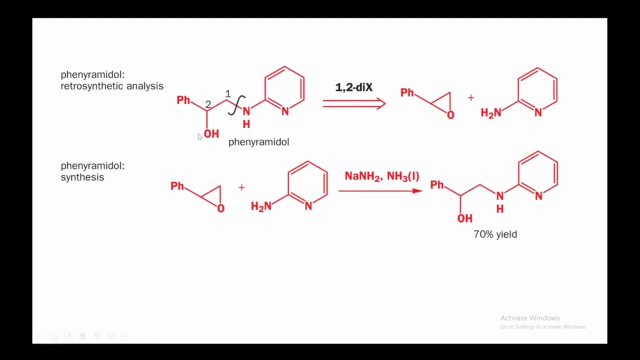 is how you can use the two, two group disconnections. what were the two groups here? one was ether and one was alcohol. so this is how we can use this approach. okay, let's move on towards more examples now. this is another example of two groups where you have a secondary amine and alcohol and the 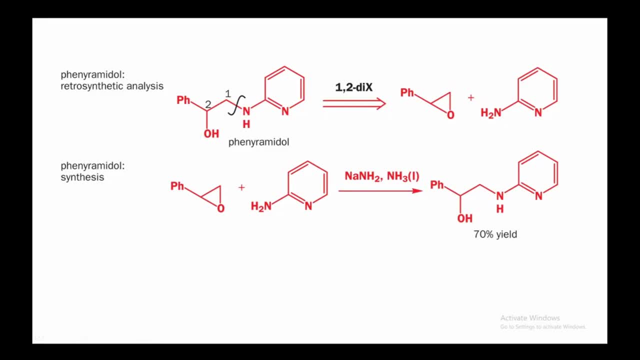 two functional groups is one, two are the two groups. two functional groups are separated by one two disconnection or one two distance. now you disconnect the cn bond and get epoxide on one side and nh2 on the other. now, in the forward direction you react this nh2 with epoxide. 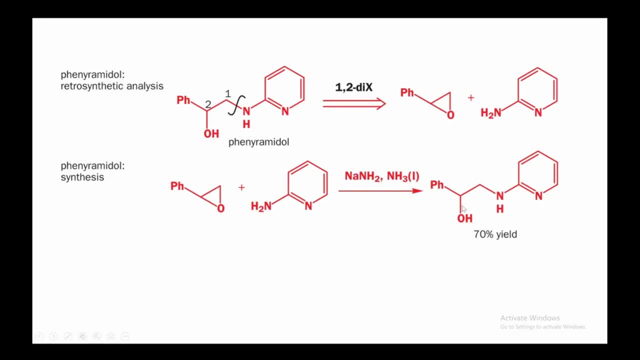 in the sodium amide ammonia, you will get this product. the ring opening reaction takes place. so that's how you can approach the two group disconnections. okay, let's say, all right, let's look at another example now. again, if you see the target compound, it contains two group 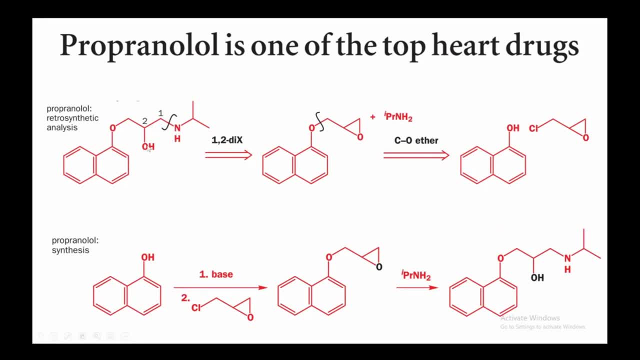 functionalities. one is secondary amine, another is alcohol. so you count the relationship between two functional groups and then disconnect the cn bond and the other side will give you the epoxide. and then you disconnect this oxygen bond between carbon that will give you alcohol on this neptune. 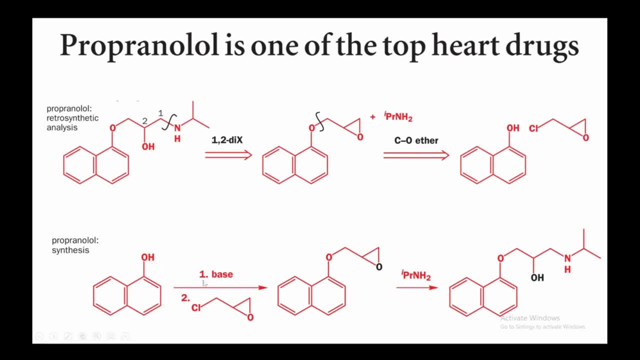 and this is the epoxide. now you react this neptole using a base to generate a negative charge on the carbon and then this will take on this carbon and the chlorine group will leave and in the next step, the second primary amine will attack on this epoxide, which is electrophilic in nature, and the 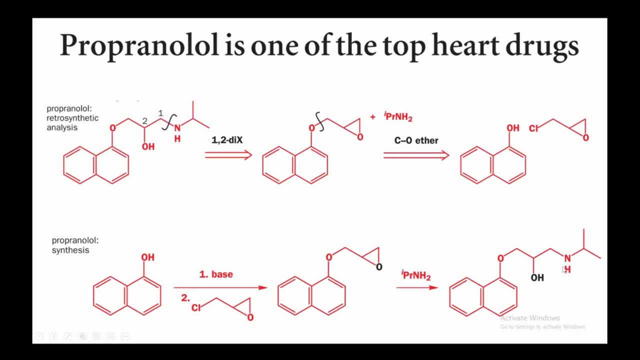 ring opening, reaction will take place, and hence you will generate a one, two die or that functionalized compound. so this is how you can recognize functional groups and the relationship between them, and then that's how you can disconnect them. all right, let's move on to the next strategy. 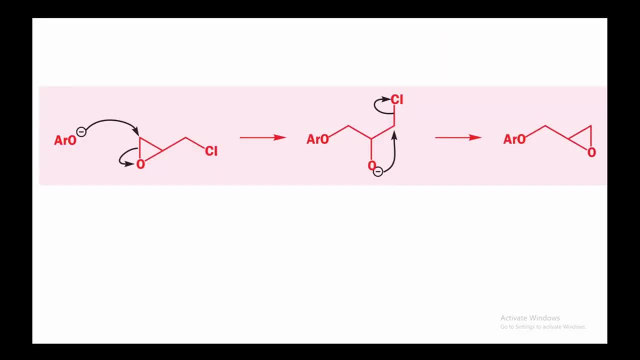 this is a very good example of how you can open the ring of epoxide and then make a ring. so this is opening and closing of epoxide ring. so you are generating a negative charge on oxygen. let's say, suppose a phenolic oxygen or alcoholic oxygen. this attacks on the 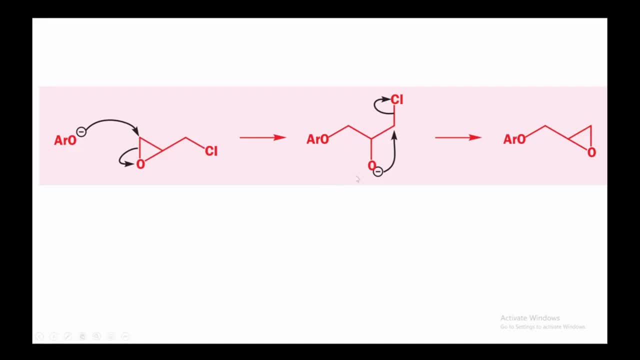 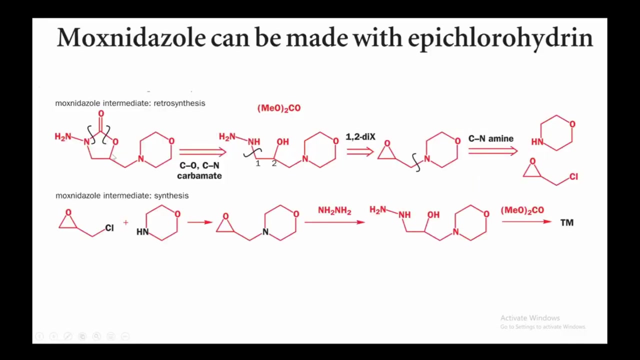 less substituted side of the epoxide and ring opening takes place. now you have a one two relationship between this oxygen and this chlorine, and this negative charge attacks on this carbon and you are generating the epoxide. let's move on to the next example, where you have a masked 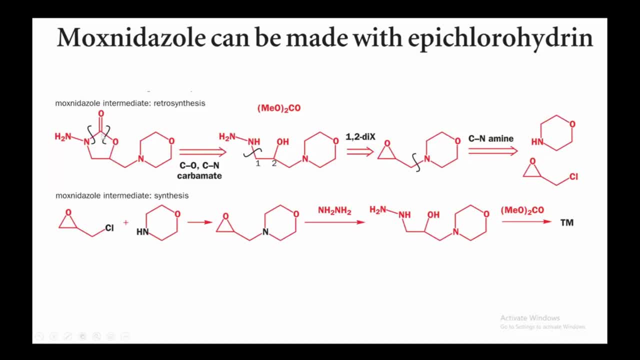 difunctional compound. so this is ester from this angle and this is amide from this angle and it's a cyclic compound. so we cannot call it ester now. we can call it amide, but we can see clearly what functionalities they are. so we disconnect this co bond and we can disconnect this. 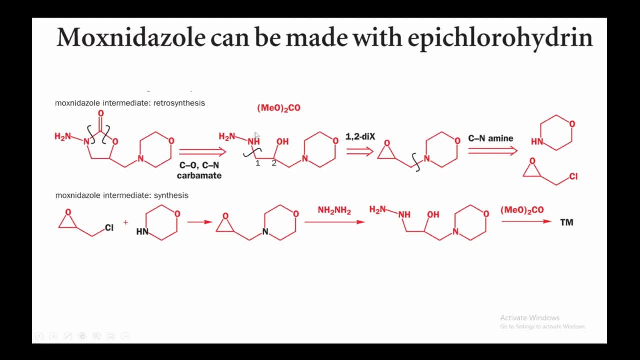 cn bond and we can see the relationship after that. so if you disconnect this one, then you will get a carbonyl group, this one wiped off, and this will be connected with the esters methoxy. now the relationship between this nh and oh is one two, so you can disconnect the bond between carbon and 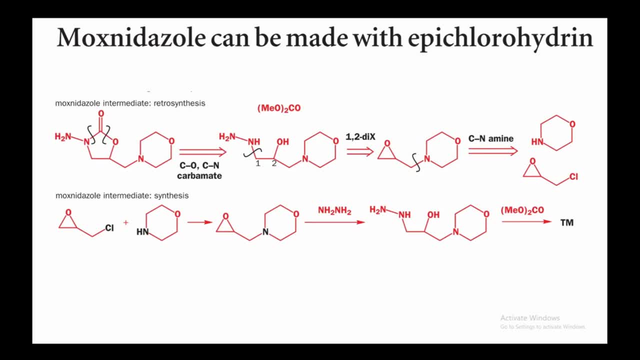 nitrogen and then, as a result, you get the epoxide formation and the next step again is the cn amine group disconnection. so you disconnect between carbon and nitrogen bond and, as a result, you get the epoxide, having the alpha carbon with halogen atom, and this is a secondary amine. now what happens? 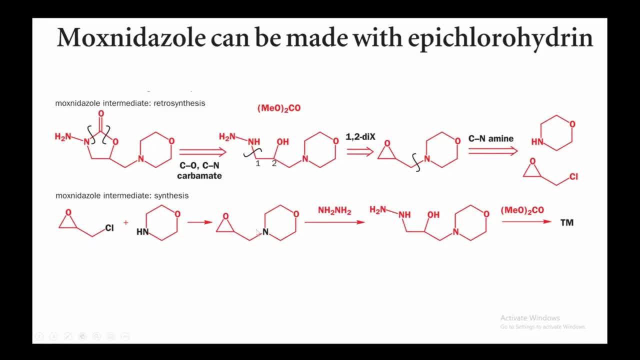 is the primary amine attacks on this carbon in sn2 fashion to give you this compound and in the next step, the primary amine attacks on the less substituted side of this epoxide ring and the ring opening takes place and you get this functionality. and in this case, 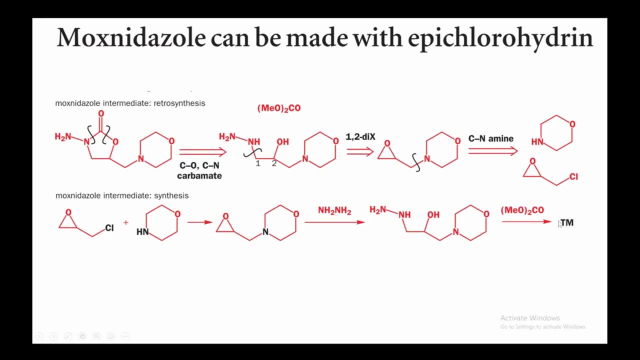 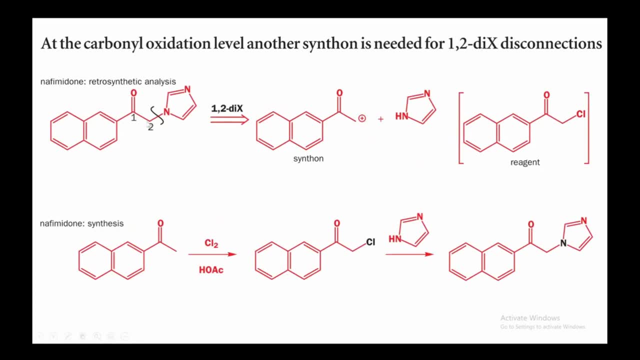 you are reacting this with this ester to get you the target compound. okay, so let's move on to the next example. if you see, here again, this is a one, two functionality. one is ketone, second is having a heterocyclic ring. it doesn't matter, you need to figure out the relationship between the 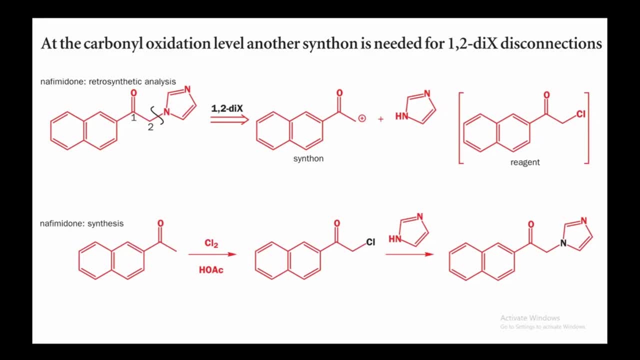 function. you don't need to panic by looking at the different functionalities. or you don't need to panic by looking at the big molecules or different structures. focus, be calm. just figure out what kind of relationship, what kind of functional groups they are. so you disconnect from one to disconnection- that is, c and disconnection- and you generate a positive. 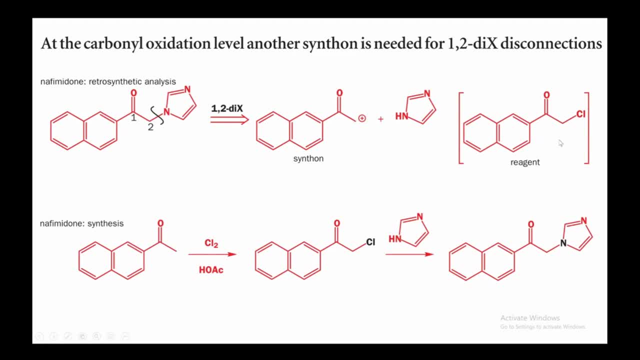 charge on carbon. number two, and that is equivalent to this reagent, that is alpha halogenation, that is alpha chlorination of the carbonyl compounds, and this is the second element. so what happens? you have alpha carbon here or alpha hydrogen, so these are replaced with one chlorine. 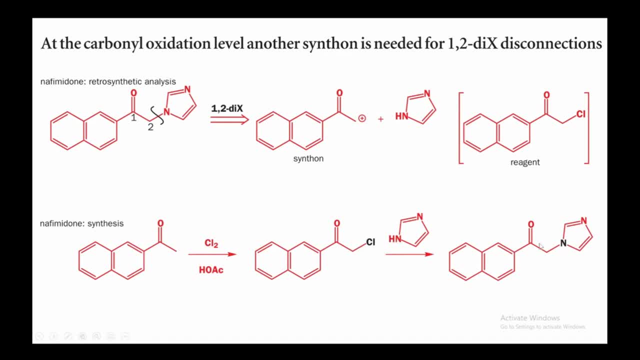 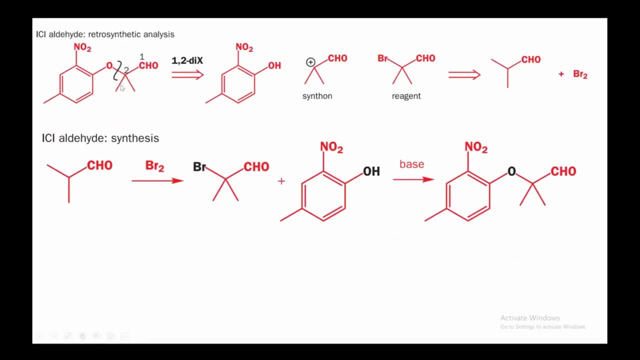 and then this nh attacks on this carbon and then you get the product. okay, let's move on to the next example. so this is the next example where you have aldehyde and ether functionalities. so the relationship between aldehyde and ether is one- two. so you disconnection. 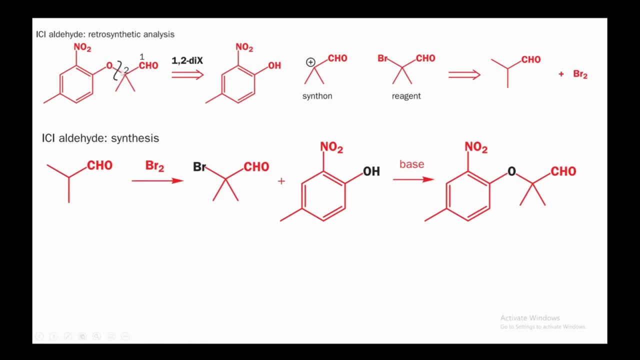 the co bond and then you get alcohol or phenol on this benzene and the positive charge. positive charge on this aldehyde side, which is equivalent to this reagent, that is alpha bromination on the alpha carbon of aldehyde, and you can disconnect this bromine to start from simply. 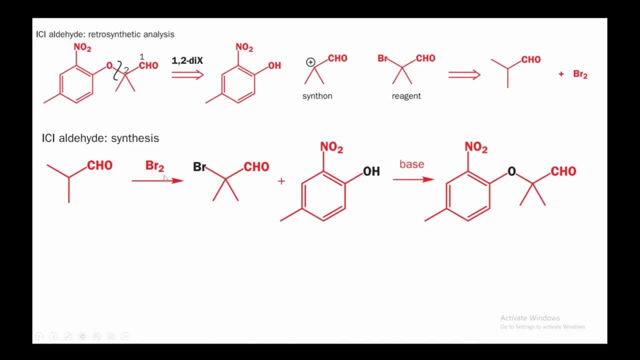 starting aldehyde. now this aldehyde reacts with br2 to give you the alpha brominated product, and then this react with this phenol in the presence of paste to give you the desired product. so this is how you can use the one, two group disconnections to generate the simple starting materials, and this is a very 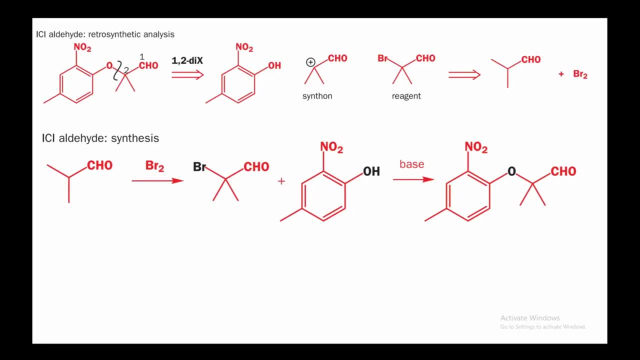 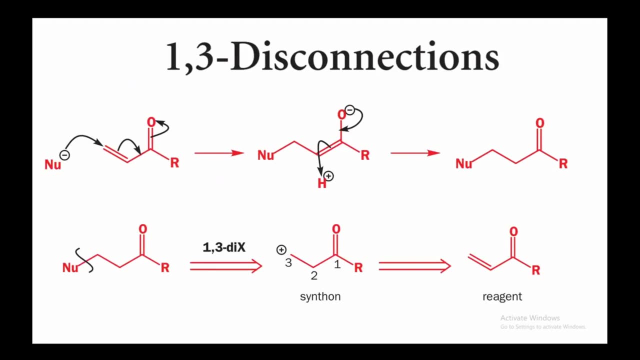 good way to use these strategies for retrosynthesis. okay, let's further move on to one three disconnections. now in one three disconnections, there are different possibilities. either you get this double bond- this is a michael acceptor, a nucleophile attacks on this position- and the bond. 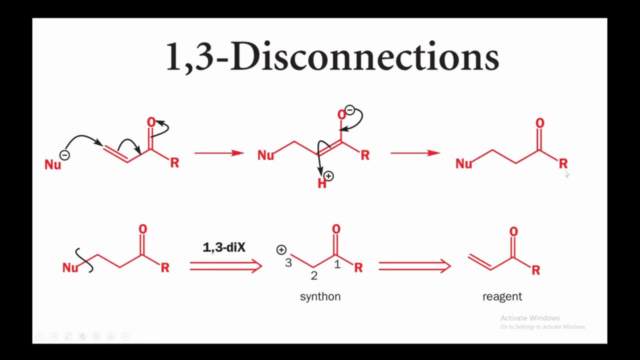 formation between this carbon nucleophile takes place in. this is a mechanism. now, if you are given such kind of a situation where you have a carbonyl compound in a nucleophile at position three, that is called one three disconnection. so you disconnect the nucleophilic position, generate a positive charge on carbon number three, which is equivalent. 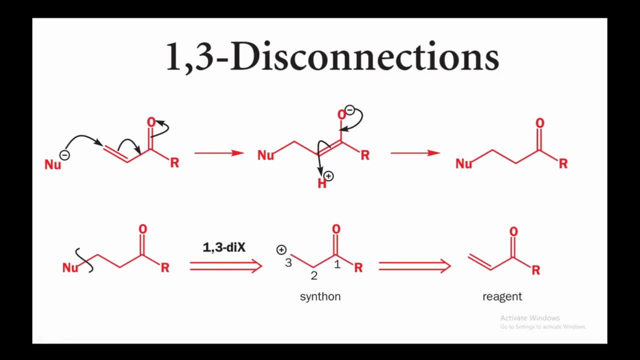 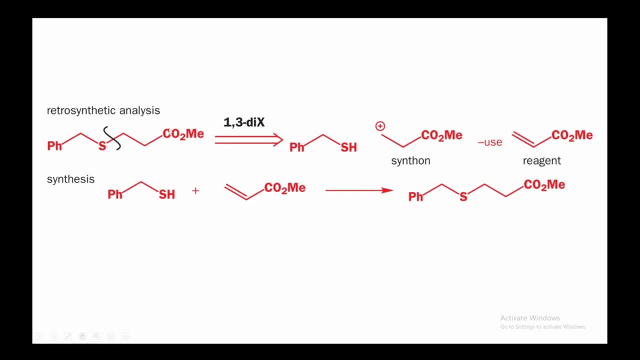 to this reagent. okay, now let's apply this concept to the molecule. you have this situation where this side is a nucleophilic and the other side is a nucleophilic and the other side is a nucleophilic, and this is your carbonyl compound: one, two and three. so you disconnect this cs bond. 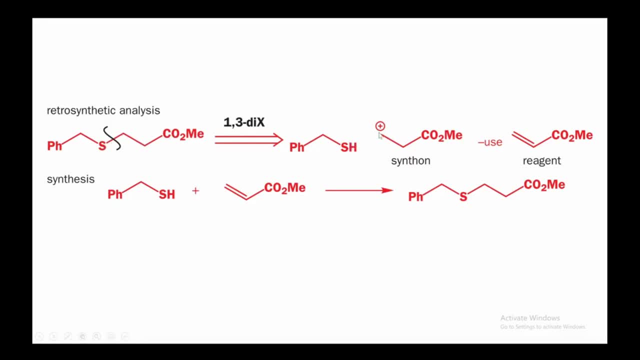 that is called one three: disconnection. this becomes sh and this side contains a positive charge. it's a centon. there's a reagent for this centon is this michael acceptor. so you react this nucleophilic style with this michael acceptor and you will get the product. so this is how we 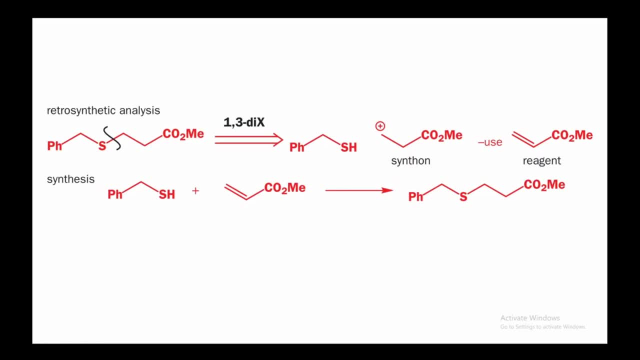 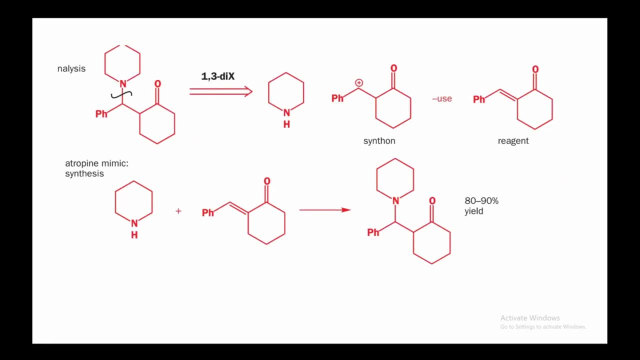 can apply this one three disconnection concept to the organic molecules for retrosynthesis. all right, let's move on to the next concept, which is the organic molecules for retrosynthesis. on to the next example. again, this is a one three relationship between this tertiary amine and this. 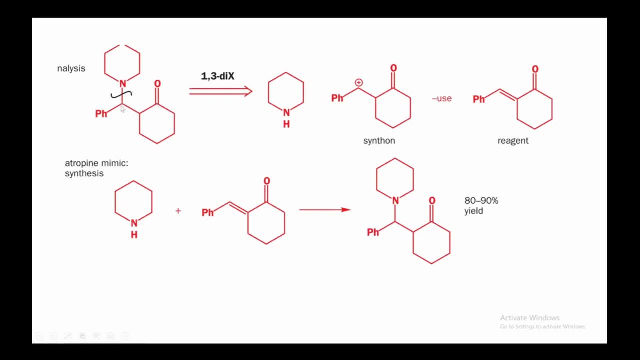 ketone. so if you count one, two and three, so you disconnect the cn bond, you will get a secondary amine and a positive charge here. this is a centon, which can, which is equivalent to this reagent. now you react this paper, yeah, piperidine, i think. then with this, uh, michael acceptor. 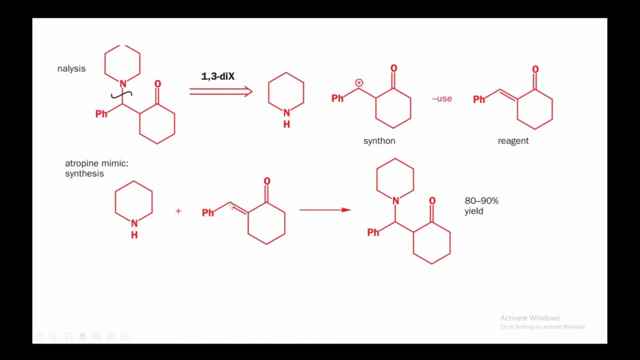 this nh attacks on this double bond and then you have one formation between this three and a nitrogen and an excellent yield. you don't need to write yields when you are writing the synthesis in the exam, because you don't know, you are not sure this is a 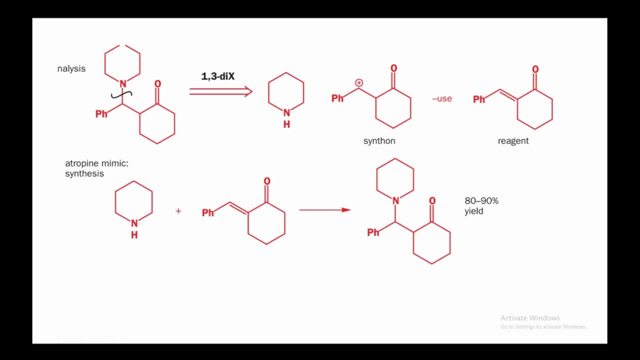 snapshot from a book. this is a well-known or reported reaction in the literature. that's why the authors reported here. but you are not supposed to write yields in the reaction. okay, make sure you don't confuse yourself with this. all right, let's move on to the next example. 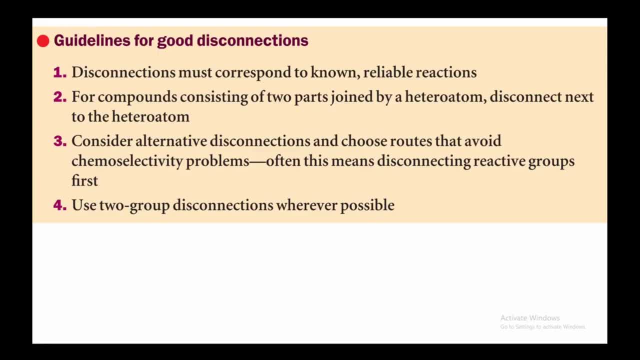 and furthermore, if we go down, we need to follow the guidelines for good disconnections. what are good, does disconnections, which disconnections are pretty good or which disconnections are reliable? number one: disconnections must correspond to known reliable reactions. number two: for compounds consisting of two parts joined by a heteroatom, disconnect next to the heteroatom. 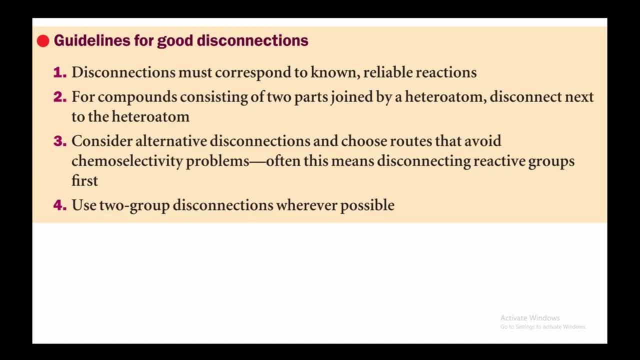 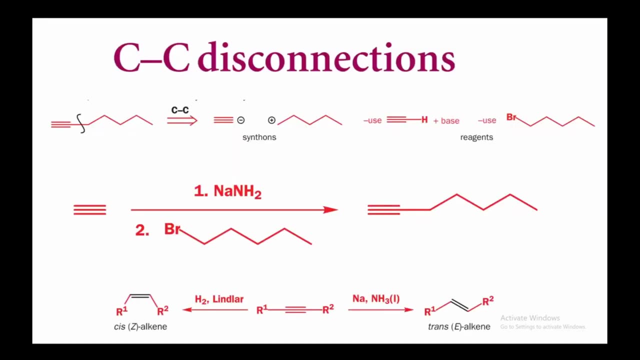 number three: consider alternative disconnections and choose rules that avoid chemoselectivity. often this means disconnecting reactive groups. first. number four: use two group disconnections where possible. all right, let's discuss the cc disconnections. you you have alkyne and alkyl chain, so you disconnect from this cc bond. 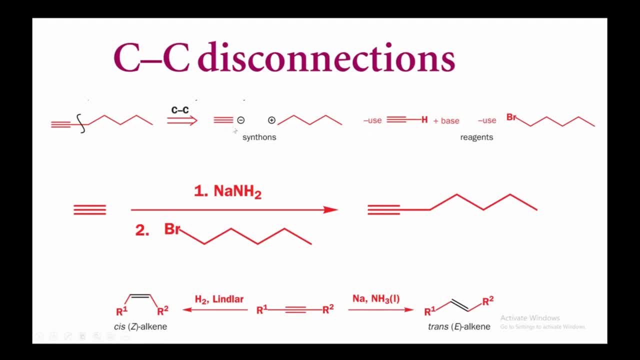 and you generate a simple ethane molecule and a positive charge on this. so ethane is a well-known nucleophilic must compound which can be used as a nucleophilic, and this positive charge on this carbon anion is a very important reaction to the response to this alkylonite. what happens is there is a acidic 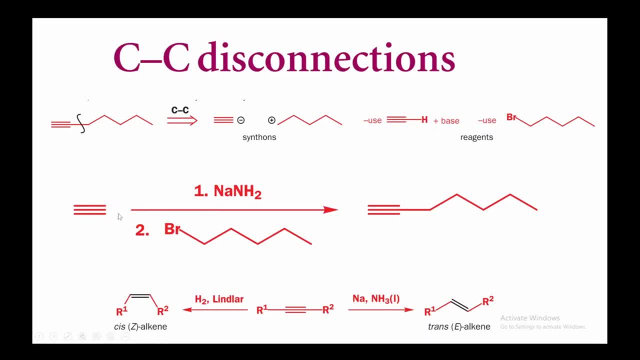 hydrogen on this ethane. so sodium amide is a base which deprotonates this acidic hydrogen and then generates a negative charge, which negative charge attacks on this carbon in an sn2 fashion to give you this product. this is a very important reaction: the conversion of alkynes into alkenes. but there's 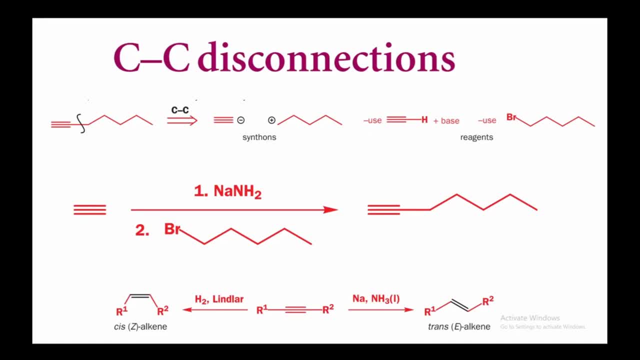 a steroselectivity problem. so if you want to achieve a cis alkene or z alkene, you must use at least h2pd. if you want to convert alkyne into e or trans alkene, you must use sodium and liquid ammonia. that's how you approach it. okay, i? this is how you can generate trans alkene or cis alkene. 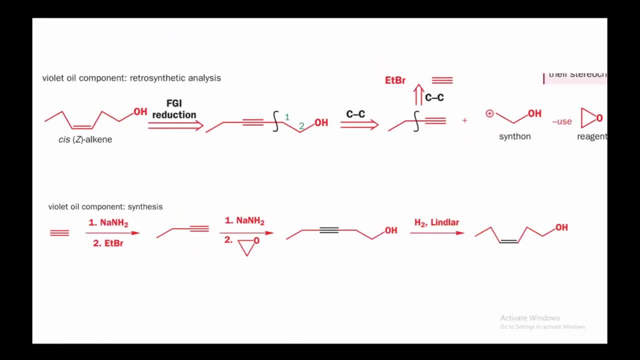 from all kinds. okay, let's move on to follow this strategy, or follow that concept to the real, apply this concept to the real example. so you have this example. what you do is you add to fgi reduction. basically you're converting alkene into alkynes and then you are generating a some sort of relationship between two functional 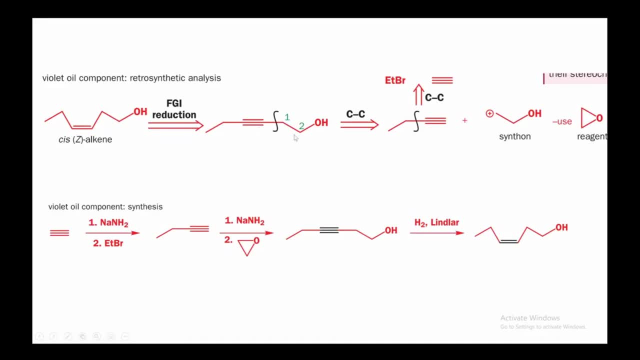 groups? what are the two functional groups here? one is alkyne and another is alcohol. so you are disconnecting alkyne from one position, that is cc bond disconnection- and the one side becomes this one and another side becomes this positive charge and this carbon, which is equivalent to this. 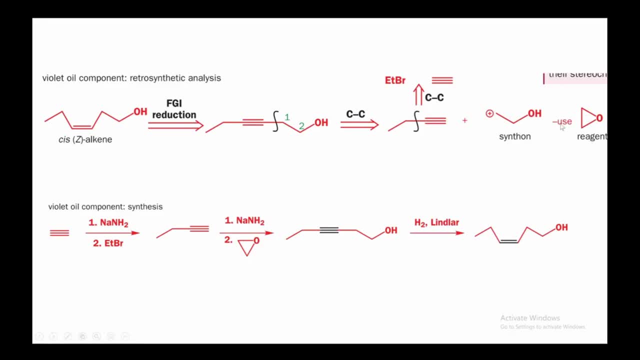 epoxide ring. we have seen this situation so many times in this series of lectures, like in this series of slides. now you can disconnect this ethyl group ethyl, make it ethyl bromide and start from a simple ethyne, and this ethyne contains hydrogens on both the sides, and now you are reacting this. 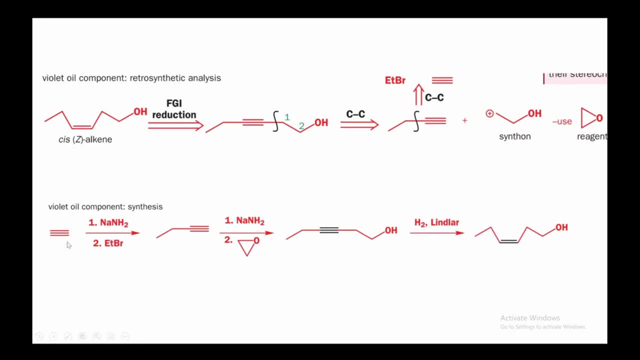 ethyne with sodium amide base, which generates a negative charge on this side of the ethyne and it attacks on the ethyl bromide gives you this, then you are reacting this sodium amide again and you are deprotonating this side and you are generating a negative charge which attacks on this. 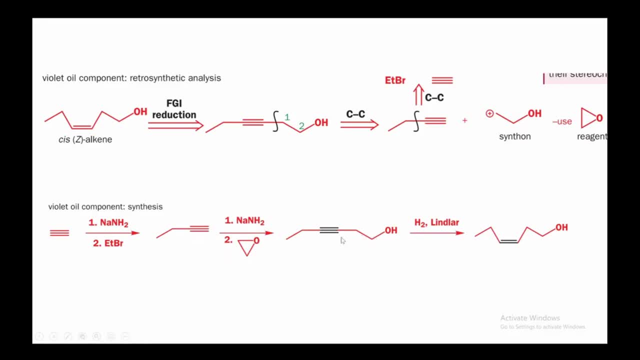 epoxide and it gives you this, then you are reacting this alkyne with h2 lindox catalyst, because you are, you need a cis or z alkene. hence that's it. so this was a strategy that we followed for generating the cis alkene from the by using the alkyne strategy, and it's a good example to have. so you should. 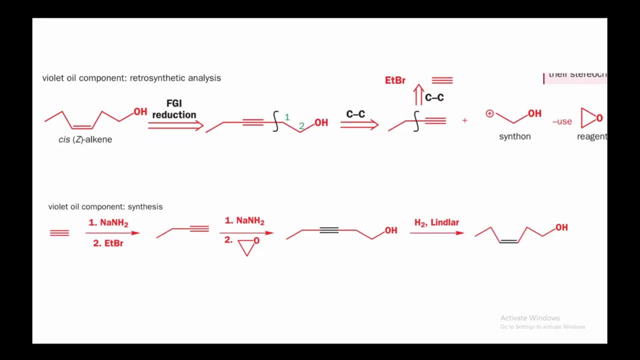 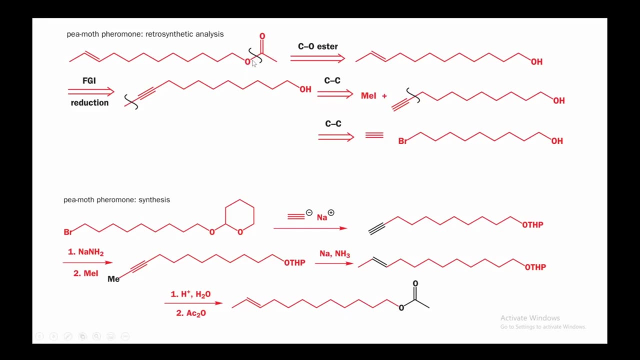 understand these simple tricks in order to apply them whenever you can in any complex or different a difficult molecule. okay, let's move on to the next example now. this is ester and this is alkene. so you already know how we can disconnect esters. so you disconnect esters by co ester linkage. 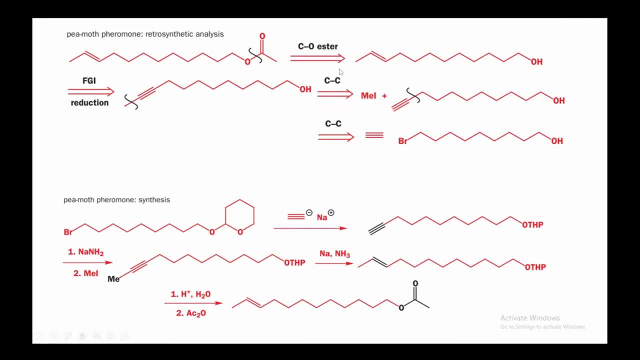 and one side becomes alcohol and another side becomes carboxylic acid. and the next step is converting alkene into alkynes, and then you are disconnecting this side becomes methyl iodide, this alkyl halide part, and this is a ethylene similar to ethylene containing a one acid hydrogen, and then you are disconnecting this. 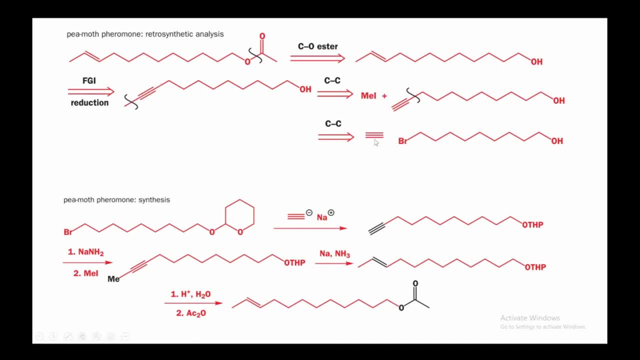 big alkyl chain and you can start the synthesis from simple ethylene compound. but here is the issue of alcohol. so you first protect the alcohol, otherwise you can generate a intramolecular reaction between alcohol and bromine. so you first protect alcohol, then you start with this. now this negative charge on ethylene. 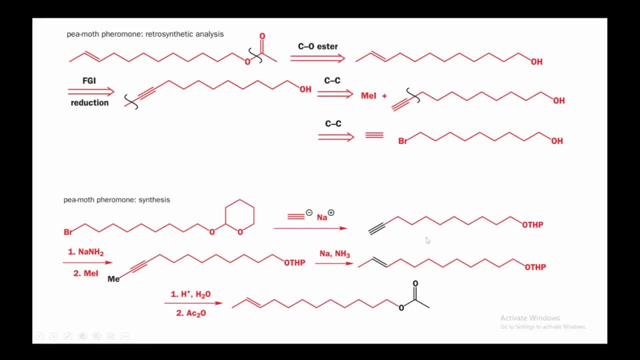 generated with a base sodium amide. it takes on this carbon and bromine leaves and you get a protected alkyne. and the next step? you again use a base sodium amide and methyl iodide to generate this functionality. and in the next step, you are converting this alkyne into a trans alkene using 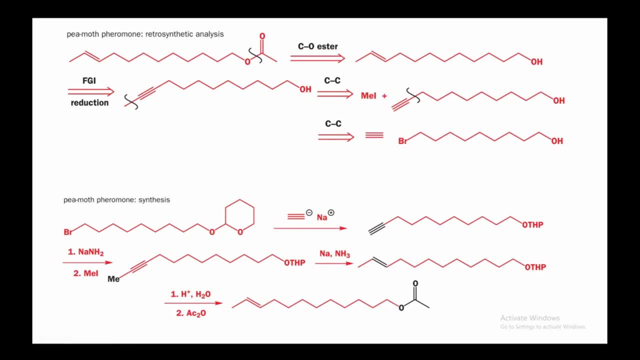 sodium and liquid ammonia rather than linlots catalyst. if you use linlots catalyst, you will get a cis alkene, but if you are using sodium and liquid ammonia, you will get a trans alkene and in the next step you can convert this protected alcohol by deprotection into the 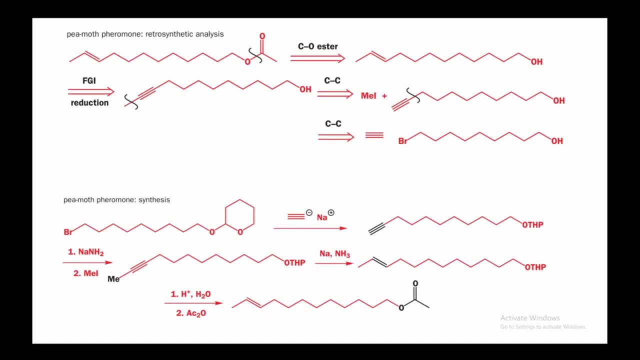 alcohol and then using acetic anhydride to generate, give you the product that is ester, containing functionality. okay, that's the way, that's the method that's you can apply it and generate the desired functional groups for applying this kind of a strategy. okay, let's move on. 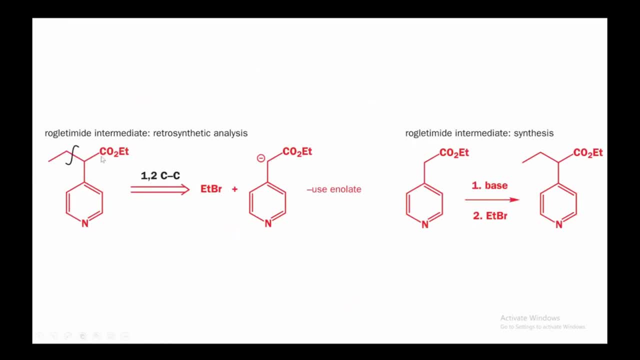 to the next example. now, this is a different approach. this is a ester functionality and this is the carbon and this is alkyl chain. you disconnect this chain. that becomes ethyl bromide and you generate a negative charge there. okay, now how you can? you can do the synthesis of this. 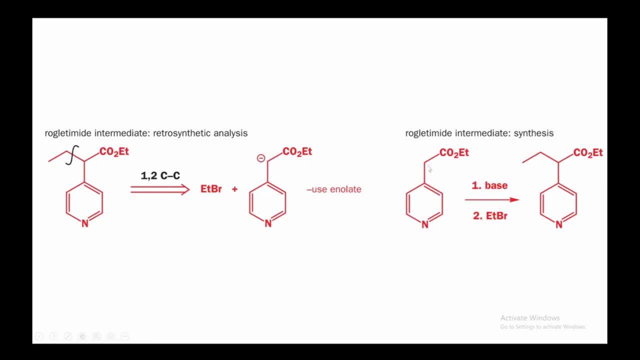 this is the compound which contains alpha carbon and its acidic position, and you can use the base, which generates a negative charge on this position, and the ethyl bromide as the alkylating agent to generate this compound. so this is a very simple way to alkylate the alpha position of carbonyl compounds. okay, let's move on to the next example. 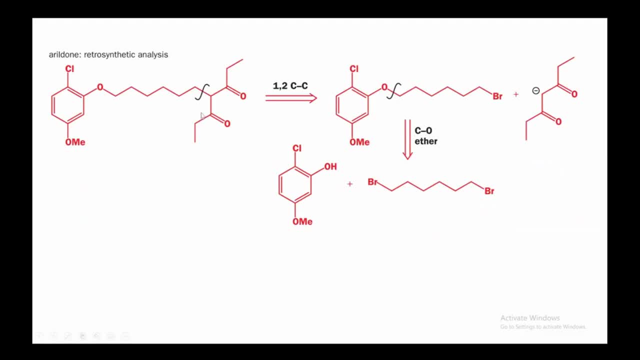 so this is again uh example of alkylation on the acidic position of carbonyl compound. so you disconnect it from this position and you generate a bromine on one side of the compound and negative charge on the other side and you generate an ethyl bromide on the other side and you generate a. 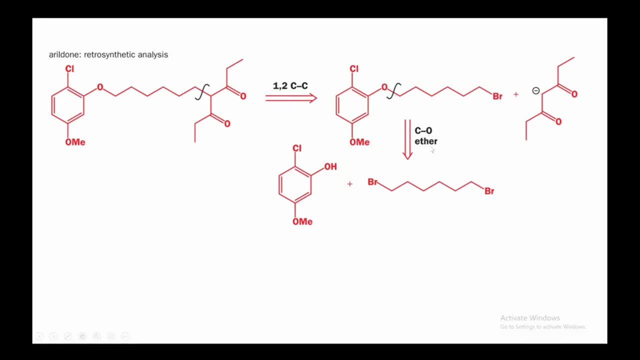 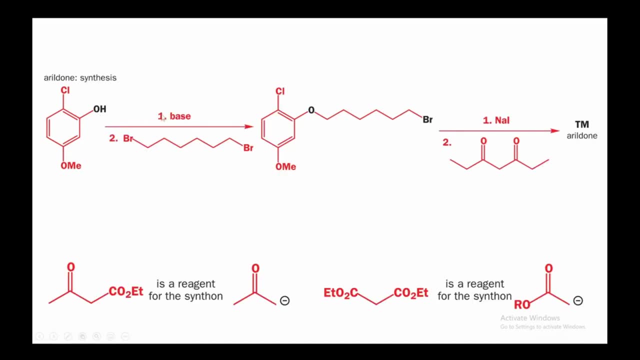 carbon bond and then you disconnect from co bond- that's a ether bond- into alcohol and this is dialkyl halide. now you do the synthesis, so you have a phenol, you generate a negative charge at phenolic oxygen and then this negative charge attacks on this bromine and it gives you this. 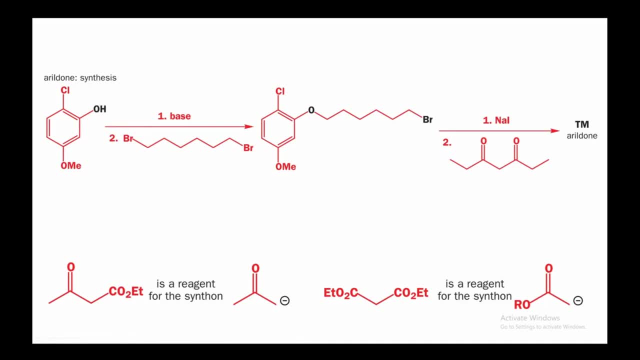 compound having ether linkage and then you are reacting this with carbon compound and then you get the target compound. so that's the method for generating this functionality and this is the approach for alkylating carbonyl compounds at the alpha position. now, if you have to do this strategy, like this compound, 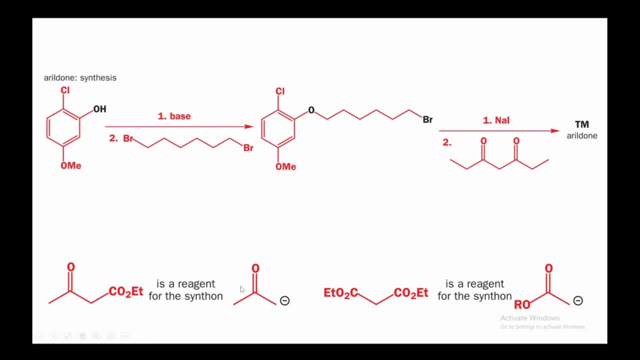 having ketone and ester, so it's a reagent for centon and this one. you are generating a negative charge, so there's, this is the reagent for this, and if you are generating this negative charge here, then the reagent should be this one. so this: 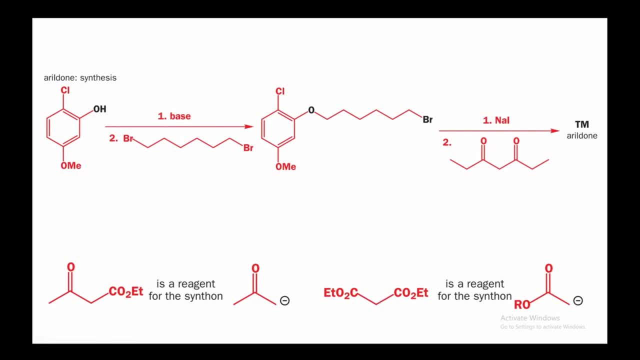 is a very good concept, very small thing, but it's applied in so many different complex molecules so you need to understand this. so if you are generating negative charge here, then your reagent for this centon it should be this: if you are generating negative charge on this position. 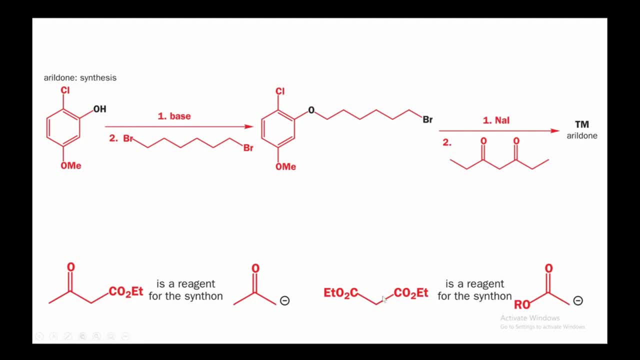 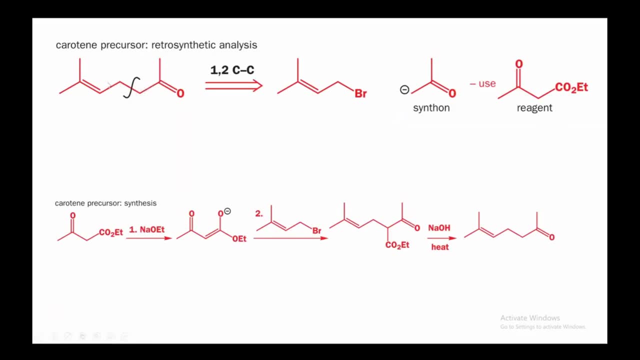 then the reagent for this centon is this one. okay, now let's apply this strategy to this compound. so this is a carbon compound and having alkyl chain containing double bond, so you can disconnect this position from the alpha carbon. this is alpha carbon, the carbon next to carbon carbon, that is. 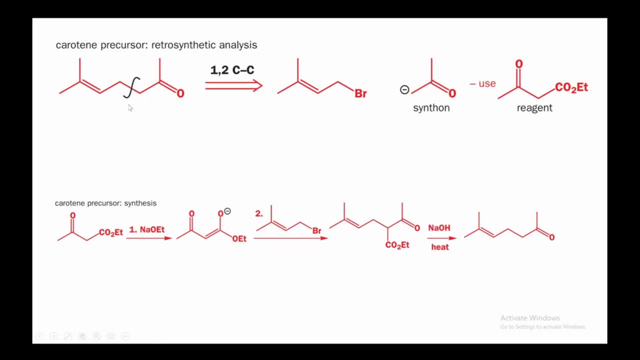 next to carbon. carbon is called alpha carbon, so you are disconnecting one to cc. one side becomes alkyl light and another side you get a negative charge which is equivalent to this reagent. now you are reacting with base to this region, generating a negative charge here, and this is a enolate. 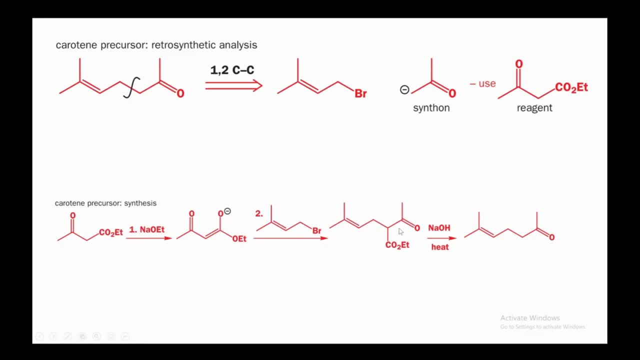 which will attack on this alkyl halide to give you this product and in the last, you can remove the unnecessary ester which was introduced for the increasing the reactivity of the alpha hydrogens, making them more acidic. so this is the approach that you can use for alkylation. 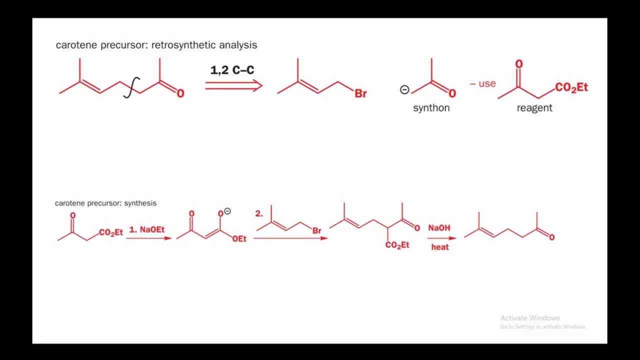 of the alkylation of these compounds. for this purpose, you can use these compounds and like introduce the ester functionalities into it so that you can generate the negative charge on the alpha carbon, and then you can proceed it for the alkylation at the alpha position. okay, let's move on to the next example. 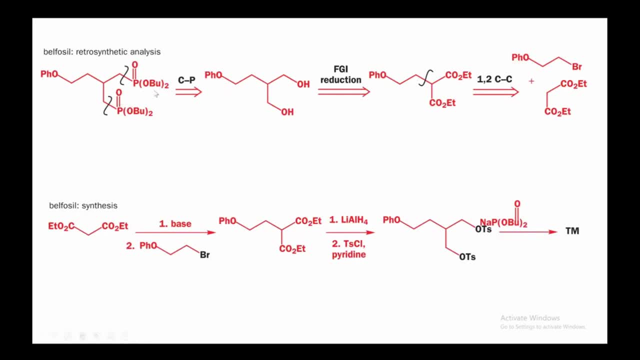 now you have a phosphorus containing compound here, so you don't need to worry about you. just disconnect the cp bond, just follow the simple hetero atom instead. you disconnect from the hetero atom, then you get alcohols, then you do the fgi reduction, then alcohol is converted into esters. 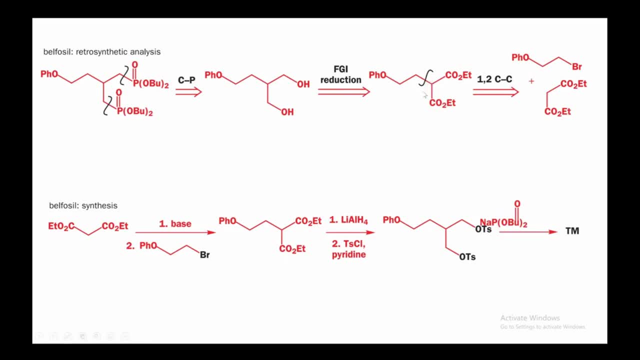 now you have alkyl part and alpha carbon, you disconnect this alkyl part and then you can start from this 1- 3 diester functionality. what happens? you react with it, with a base, generate a negative charge and then use this negative charge to attack on this carbon to generate this alkylated product. 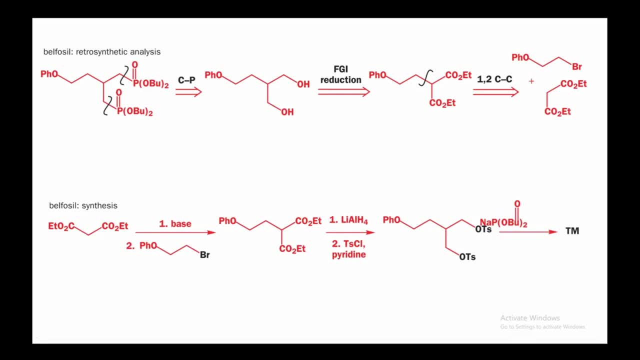 and in the next step you use the reducing agent to first convert esters into st effing compounds. this is the best way to get the buffers from the are expressed in caroxylic box, and once it is done, then you will need to resor any savory component of the protein. 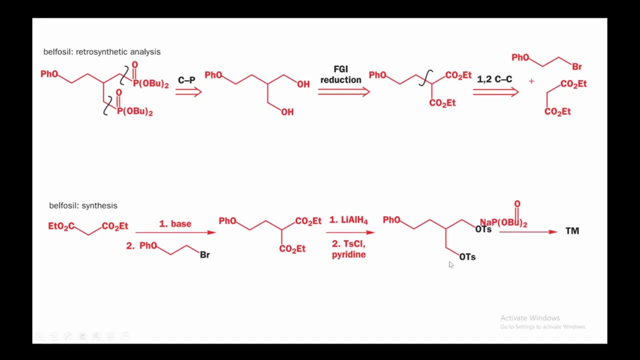 and in the next step you can use the alcohols. then you can use the totally chloride and prediene to convert alcohols into tosylates and, in the last step, Toxyl. why we are doing until s, in which we use the alkylation at the alpha position of the carbon compounds. 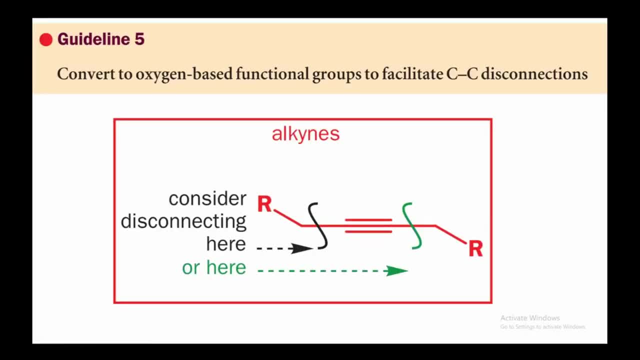 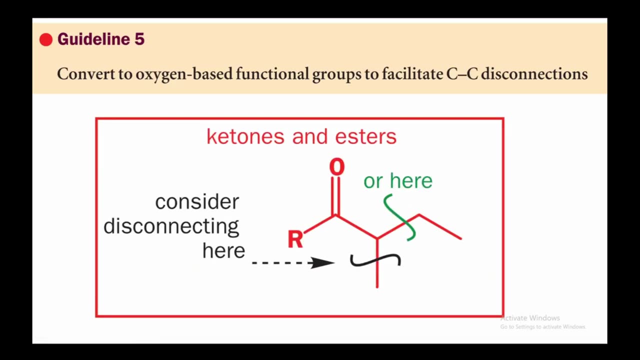 let's move on to the next example. this is a guideline. five convert to oxygen based functional groups to facilitate cc disconnection. so if you have all kinds you can either disconnection from left side or from the right side. either is fine. if you have these ketones and esters, you can disconnect it from top or bottom. this is called alkylation of. 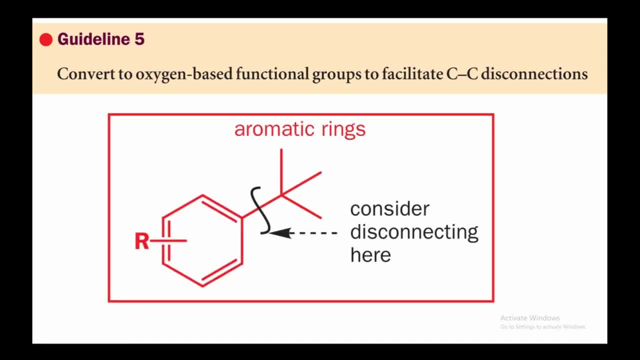 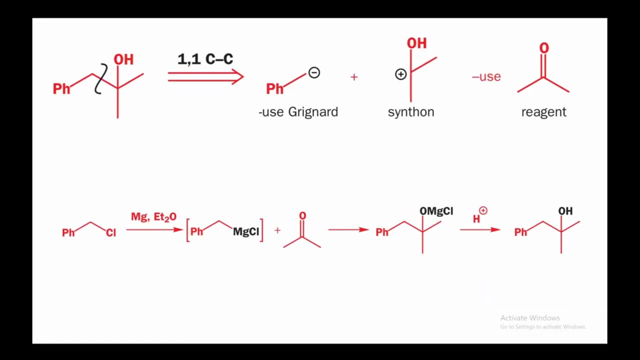 alpha carbon, so you can disconnect it from both ways. if you have aromatic ring alkylated, you can disconnect it from this position and then you can make it by friedcoll craft alkylation. ok, let's go to find out how we can do disconnection of alcohols. this is a tertiary alcohol, so you 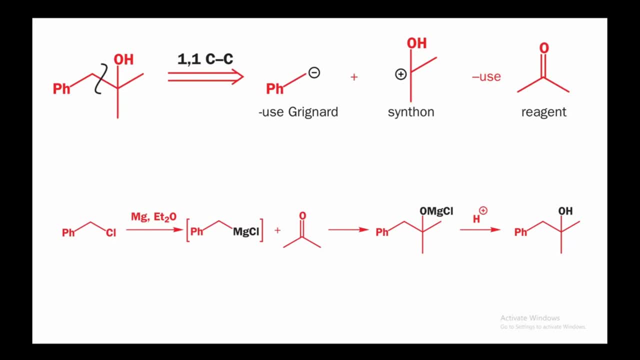 disconnect it from one side and you generate a negative charge on this carbon and a positive charge on the central atom. so the positive charge equivalent for this carbon is acetone and the negative charge equivalent for användure carbon is CDP. so this carbon, if highly strongly oxidizing co Aaron, is event to avantic ab acid tä Ridgewell. 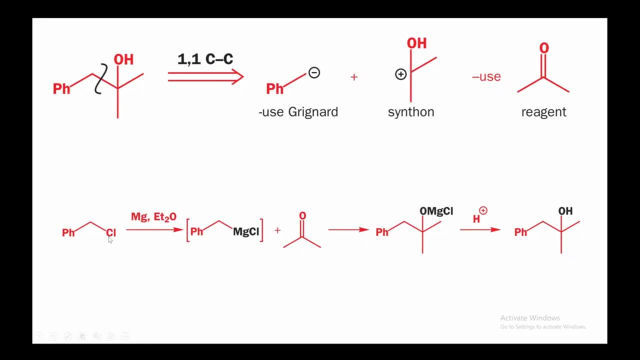 is Grignard region. so you react this alkyl halide first with magnesium, in the presence of diethyl ether, to generate a Grignard region. now this Grignard region reacts with this acetone to give you this intermediate, and then you hydrolyze this intermediate into alcohol. okay, now let's proceed further to use. 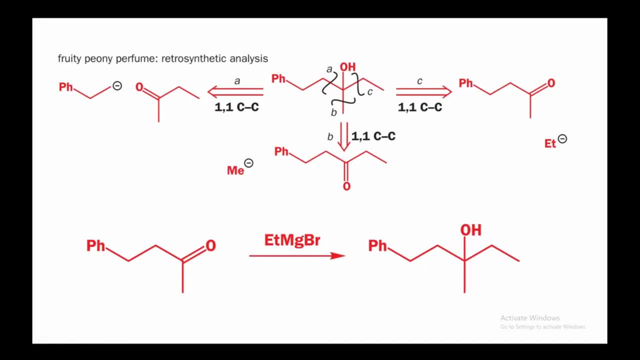 this strategy of Grignard region for formation of alcohols. now you have this unsymmetrical tertiary alcohol. there are three disconnection possible: A, B and C. so we will go through the C route that you disconnect from this side and you generate a ketone and then you react this with this ethyl magnesium bromide. 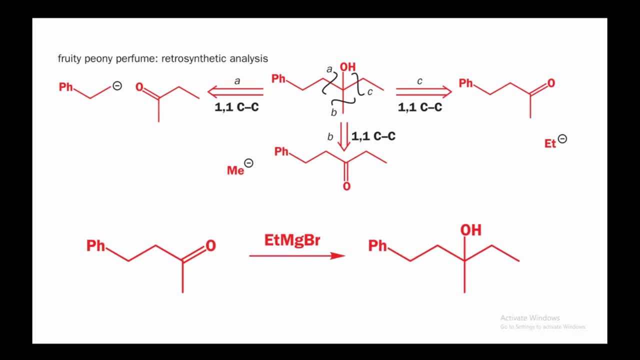 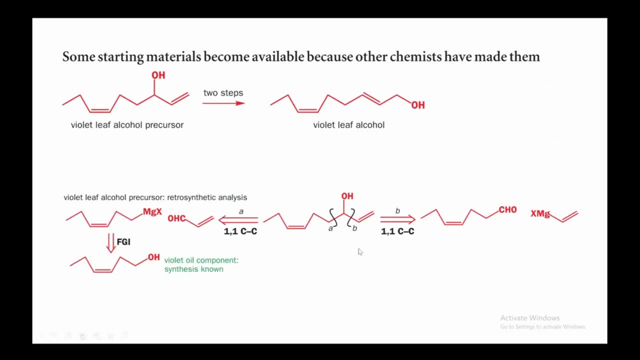 so the concept here is, when you react ketones with Grignard regions, you get the tertiary alcohols. okay, let's do this next example, where you have a- again secondary alcohol, you can either disconnect through alcohol or you can either disconnect through tertiary alcohol or you can either. 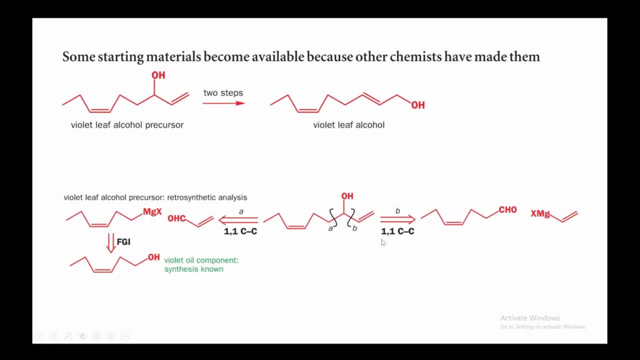 disconnect through A and B. so the B approach is slightly less favorable because generating a Grignard region on venal position is really hard task but generating on this sp3 carbonyl and Grignard region is relatively easier. so you disconnect from this position and you will get aldehyde on the one side and Grignard region on the. 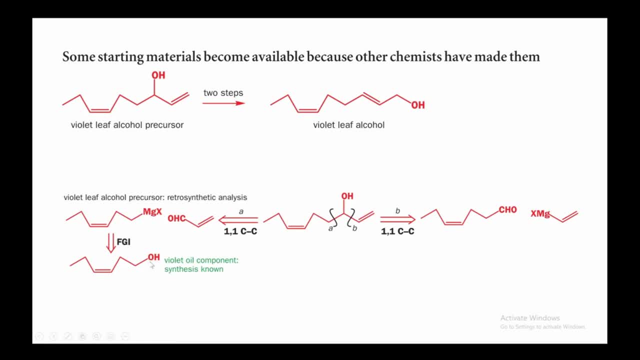 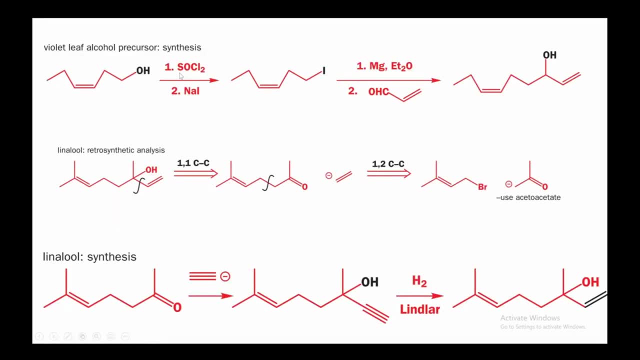 other. and then you convert this grignard region into alcohol by using FGIS strategy. let's have a sense. look at the. so you first have alcohol, you convert it into iodine by using sodium chloride, first converting alcohol into chlorine and then using sodium iodide to convert chlorine into iodine. 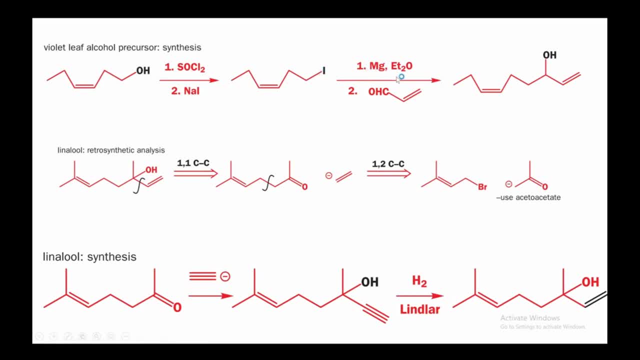 and then reacting this iodine with magnesium and diethyl ether using this aldehyde, and then you will get this secondary alcohol. that's how you use this approach. next example is again tertiary alcohol. so you disconnect from this position and you get a negative charge on this carbon. now you 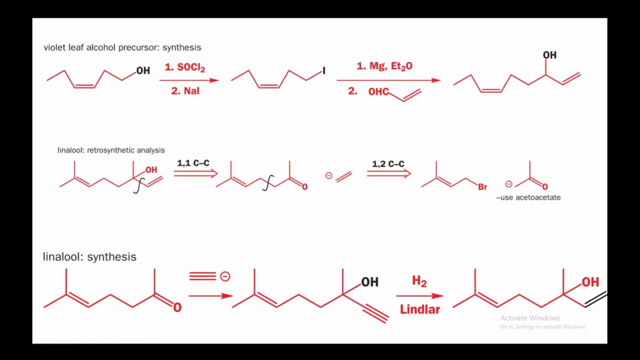 cannot choose the Gjetner region, but you can use alkyne in the state of that. then this is alkylation, escape, alpha alkylation of this carbon. will you disconnect it from this position and you get alkyl on one side and inolate on the another side. what happens? you can react these two together. 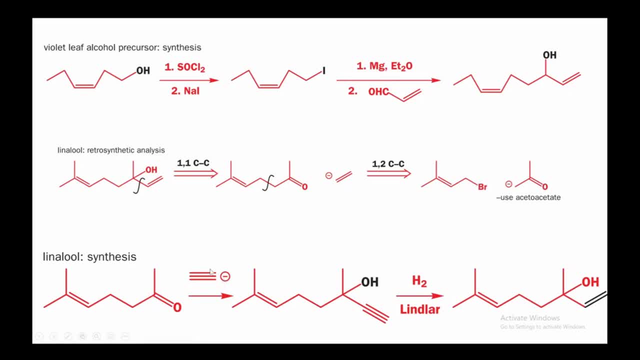 to give you this compound. and now you are reacting ketones with alkynes. they give you the tertiary alcohols. and then next step: by disconnecting now by doing reduction with lindart's catalyst, you can generate cis alkynes. that's how you can replace get, not regions, with alkynes. also, that's another way. 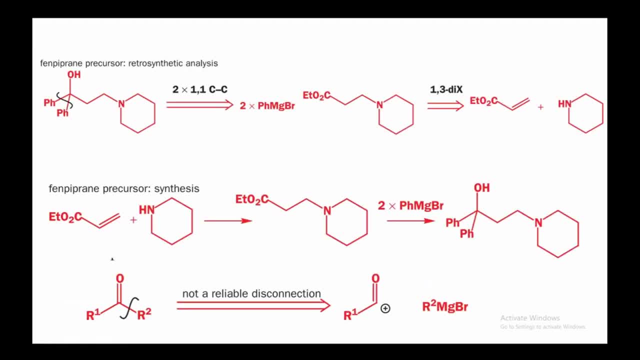 good clever strategy. okay, let's move on to the next example. this is a little bit different, but it's still a tertiary alcohol. but it's substituted with symmetrical uh substituent, that is, two diaphenyl groups. so you disconnect diaphenyl groups and make the rest compound as diaphenyl. 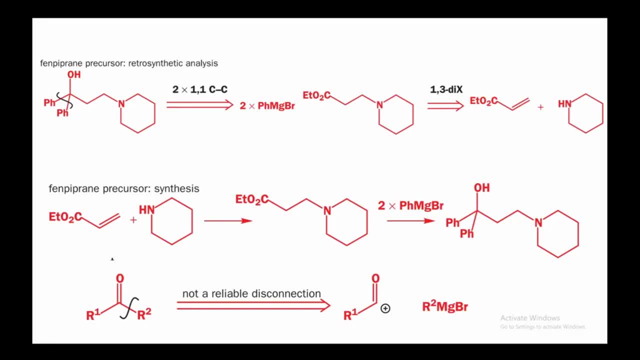 magnesium bromide and other side becomes the ester. now you disconnect this. this is a 1: 3 disconnection which we already discussed. so you disconnected from this position. one side becomes michael acceptor and the another side becomes the secondary amine. now you react this: michael acceptor with the 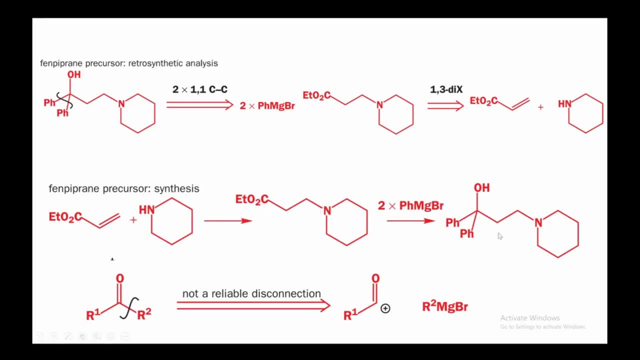 secondary amine to generate this, then you are reacting this ester with phenol magnesium bromide to generate the tertiary alcohol. okay, now you are familiar with the disconnection of alcohols and this is a 1: 3 strategy. but if you are, if you want to disconnect from this position, then these are not the reliable. 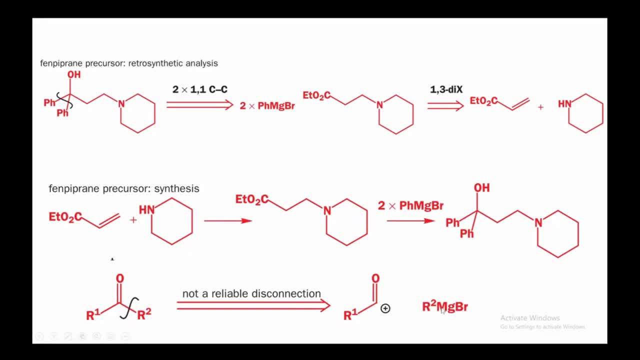 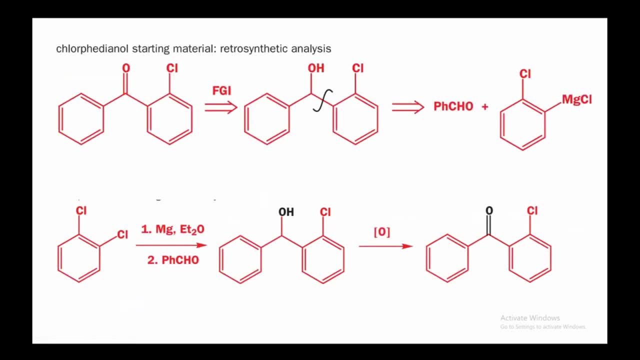 reagents, because if you react this aldehyde with this magnesium bromide, it will give you alcohol, not this one. so you need a relatively different approach. what you can do instead: you convert this ketone by using fgi strategy into alcohol. you can use fgi strategy to generate this alcohol and then disconnect it to get the aldehyde on one. 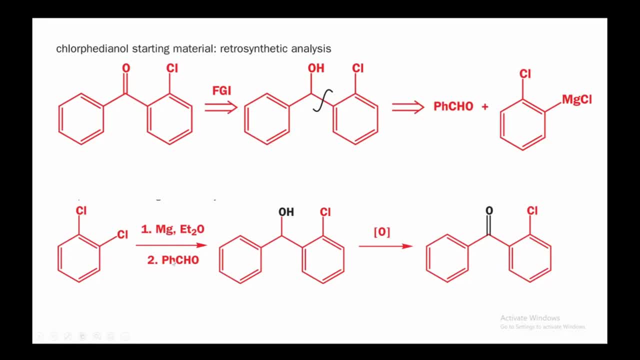 side and then get nitrogen on the other side. so, for example, now you have a chlorine. now you are reacting this chlorine with magnesium, diethyl ether and benzaldehyde. then you are reacting these together. you are generating alcohol. now you are doing oxidation of this, oh, to generate the 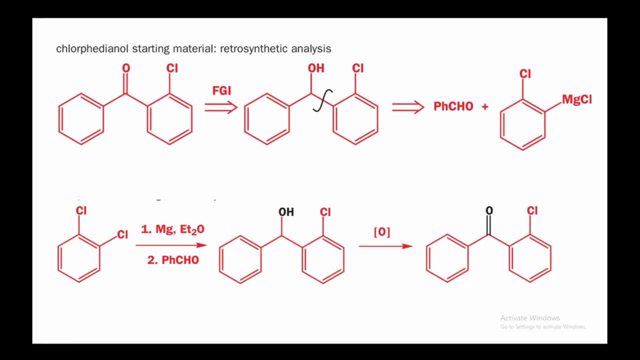 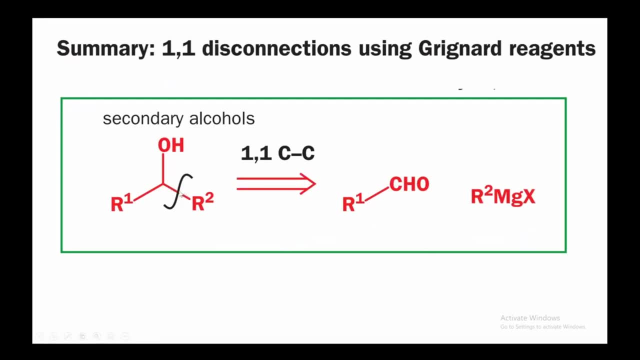 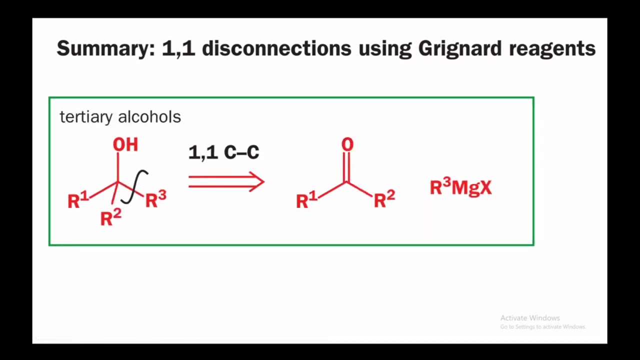 ketone. okay, this is another way of achieving your target: compound alcohols. you disconnect it from this position. one side will become aldehyde and another side will become Grignard reagent. if you have tertiary alcohols, they are unsemitical. they are containing three different functional groups, so you 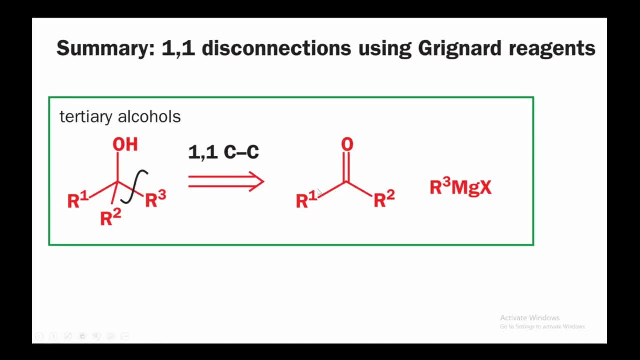 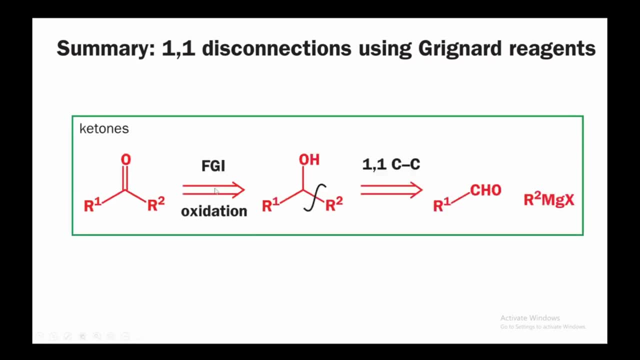 can disconnect either of these. R group and the rest of the become will be ketone and then you have a Grignard reagent reacting with ketones to give you the tertiary alcohols. if you have ketones, then you first do FGI and then 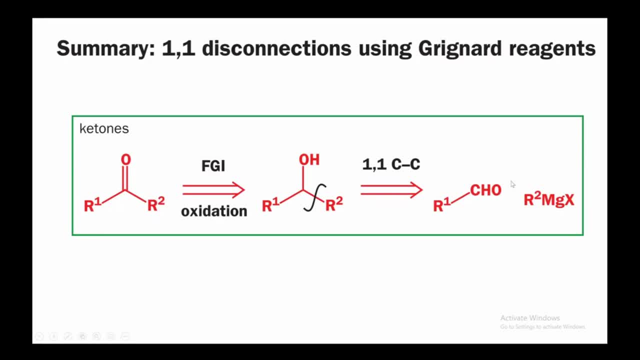 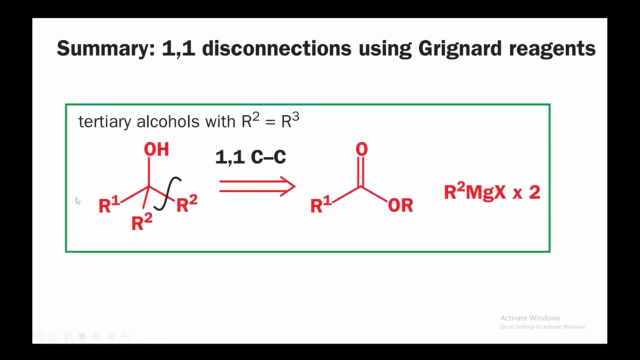 you do the Grignard type strategy, the corresponding reagents will become aldehyde and Grignard reagent. now, in the forward direction, you react this aldehyde with Grignard reagent to give you this alcohol and then you oxidize this alcohol into ketone. if you have two similar R groups, like 2R or similar R2, 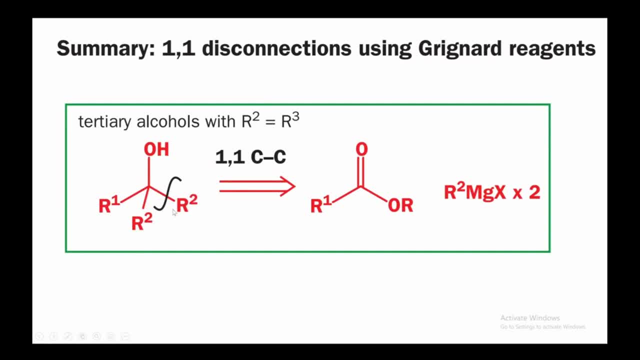 R2 means two methyl or two phenyls, then you can disconnect those two groups simultaneously at the same position, same point, and then you can disconnect these two groups simultaneously at the same point, and then you will get ester functionality with Grignard agent now. 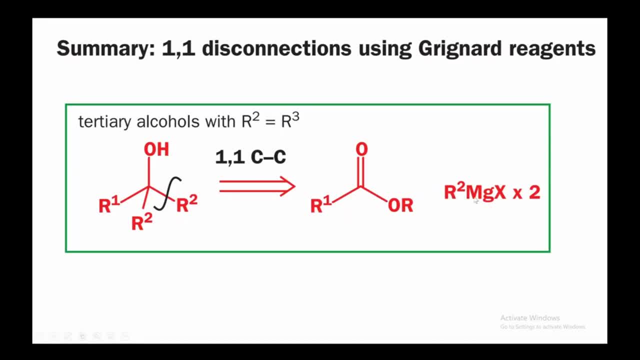 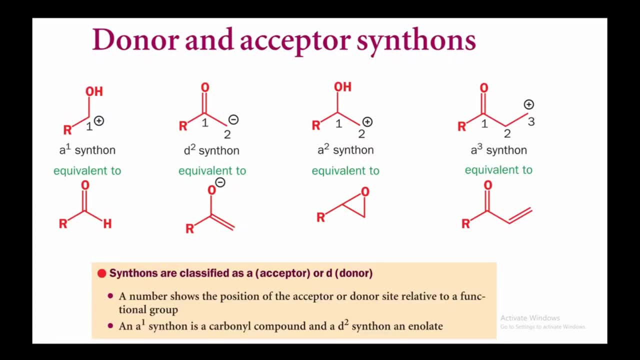 you'll react this ester with Grignard to generate this tertiary alcohol. now another concept: engratosanthes is a donor and acceptor senton. so donor is denoted with D and acceptor is denoted with a, and the number denotes the distance. so A1 means having positive charge on carbon 1. 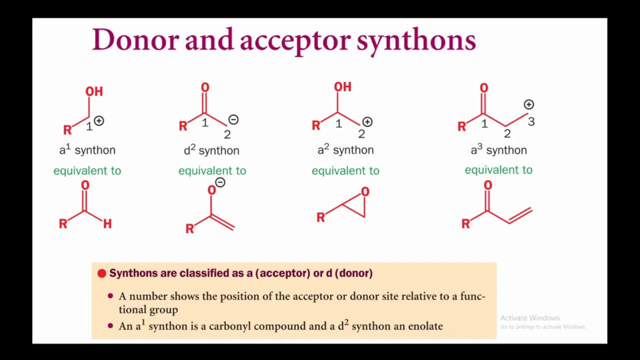 And A2 means positive charge of carbon 2 and A3 means positive charge on carbon three, so that's called a 1, a 2 and a 3 and the d 1 means negative charge on carbon 1 and d 2 means negative charge on carbon 2 and d 3 means negative charge. 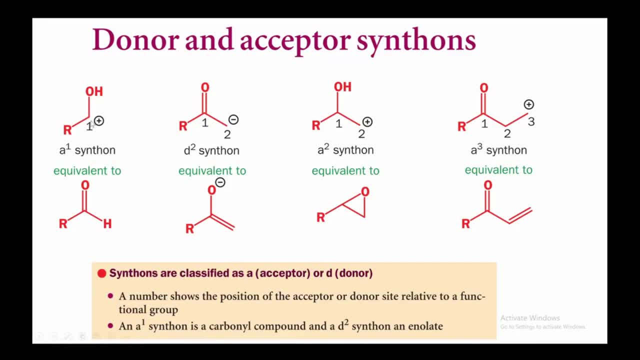 on carbon 3. so in this case, this is a 1 centone because it contains positive charge. on carbon number 1, this is d 2 centone because this contains a negative charge. on carbon number 2, this is a 2 centone because this contains a positive. 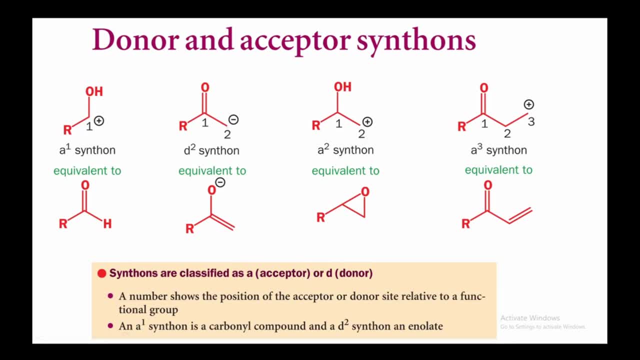 charge on heat, carbon number 2, and this is a 3 centone because it contains positive charge on carbon. number 3 and the equivalent to these centones are these compounds. so you can use a 1 aldehyde, d 2 enolate, a 2 epoxide and a. 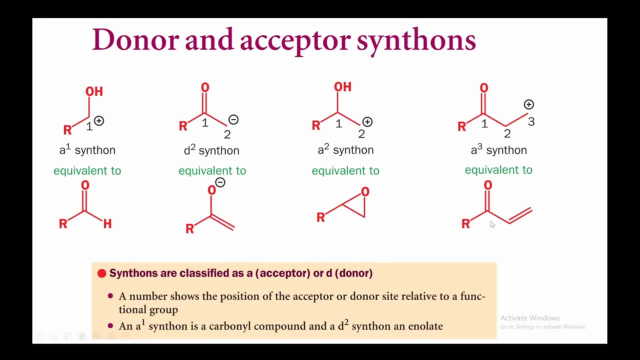 3, Michael acceptor. so if you remember this, if you understand this concept, you can do so many examples of retrosynthetics. you can do so many examples of retrosynthetics without anyone. okay, let's apply this donor acceptor concept and sometimes in exams you are being asked to provide what is type of this centon. it is either: 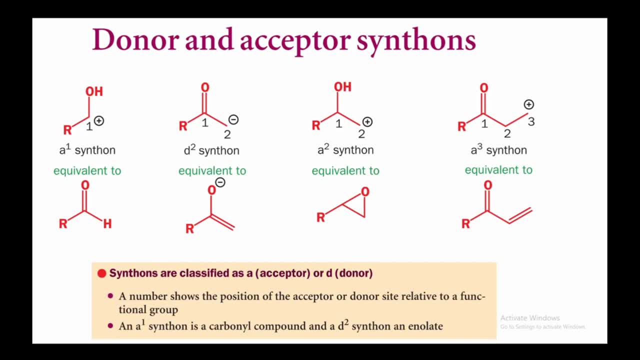 a or D. so it's quick way to identify a and D. if it is a positive charge, that's a means acceptor. if it is a negative charge, that means it's donor. and now you different. you count the numbering. so one, two, three, if it the positive charge is, 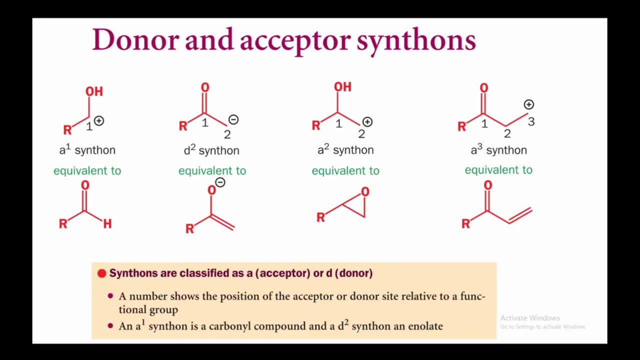 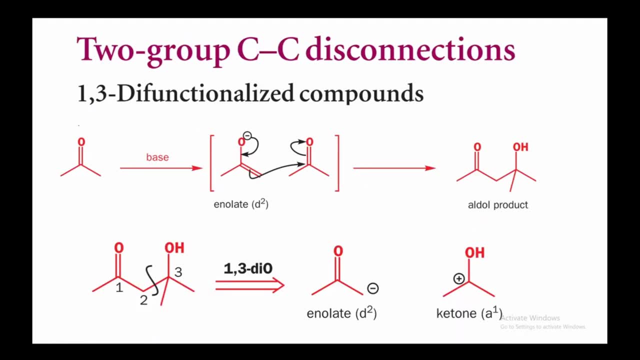 eight, carbon number three, that is called a three. if the negative charge is a carbon, number two, that is called d2. okay, let's move on. so this is important thing. that is one three di functionalized compound. so you have a acetone reacting with acetone. this is a self condensation. 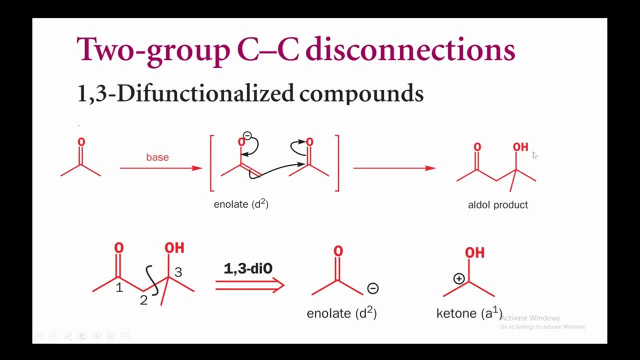 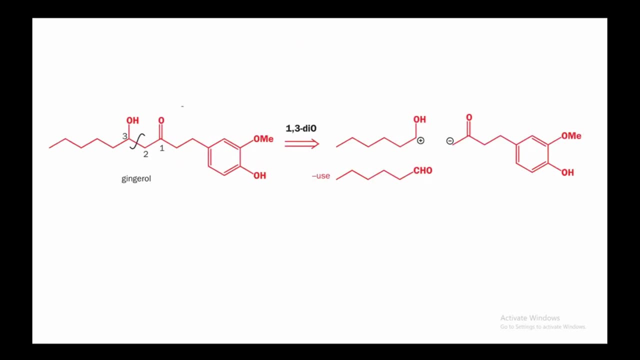 reaction and it gives you the aldol product, that is, carbon group and alcohol. now you react this aldol group. disconnect with this from position two, between two and three to generate a negative charge on the two position and a positive charge on a1. so this is a aldol product, one, two, three. so you disconnect from two and 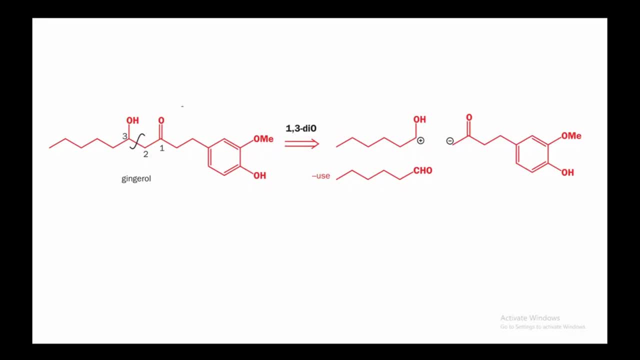 three: this is one three: di carbonyl compound disconnections and one side becomes aldehyde and other side becomes enolate. then you can construct this functional group. this is similar to the one three, the aldol products. this is alpha beta unsaturated. so what you do, first, dehydrate FGR, dehydrate, convert it. 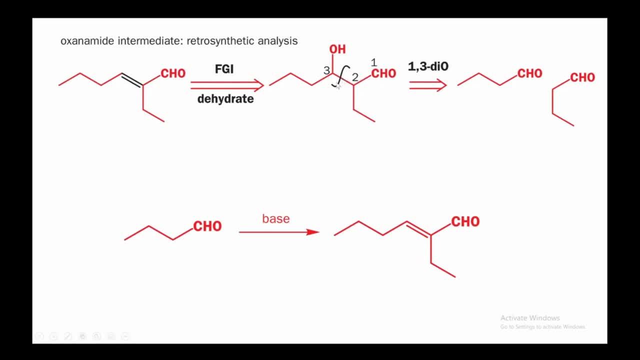 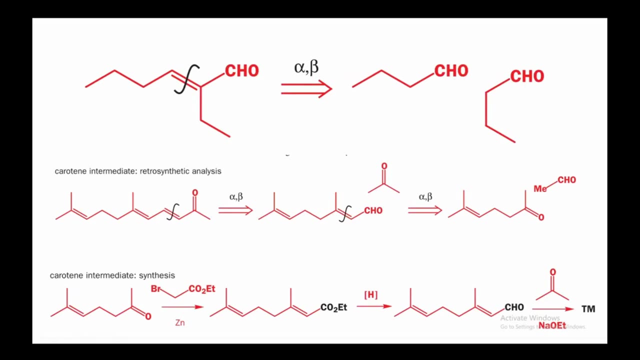 into alcohol and then you'll want disconnect from bond two and three into down three different form and this is how you can make the forward direction. so again, this is a similar to one, three diols like one, three, sorry, one three di carbonyl compounds. this is alpha beta unsaturated compound, so you 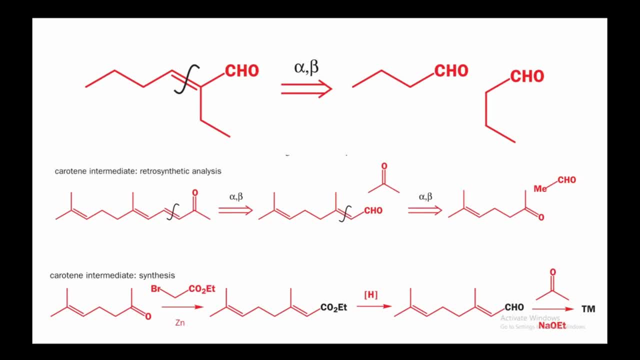 disconnect from the double bond and one side becomes aldehyde and other is aldehyde. it can be ketone as well, but in the next example we will see. so this is alpha beta unsaturated linkage. so you disconnect from this position and the one side becomes aldehyde and another becomes the acetone. now again we 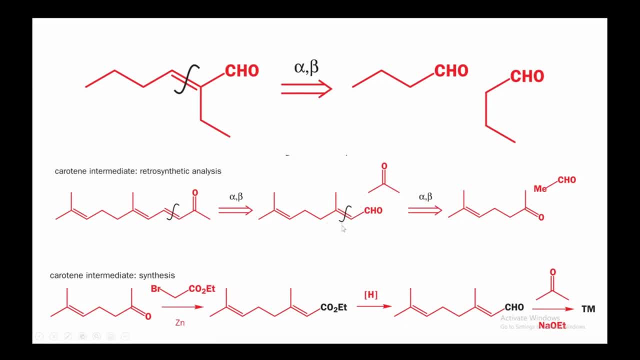 have a double alpha beta unsaturated. so you disconnect it again. now this side becomes ketone and the other side becomes aldehyde, so it's a double alpha beta unsaturated disconnection in this example. now what happens? you are reacting this with alkylating agent, you generating this ester, you are reducing. 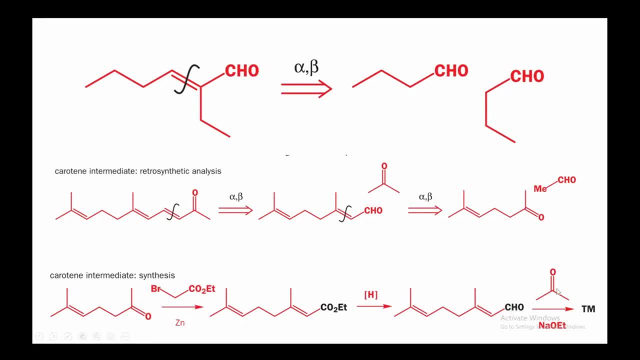 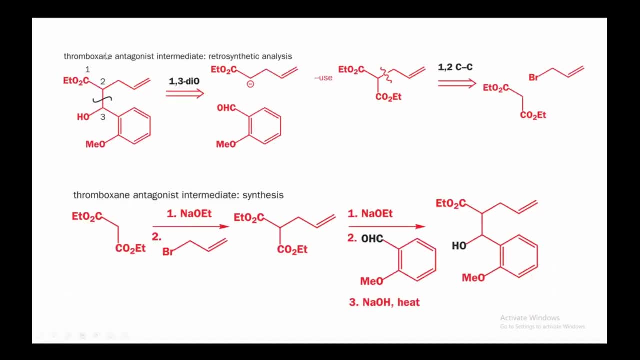 this ester into aldehyde, and then you are reacting this aldehyde with this acetone to generate the target molecule. okay, now let's move on. so this is a one three di oxygen containing carbonyl group. so this is a one ester, and three is old. 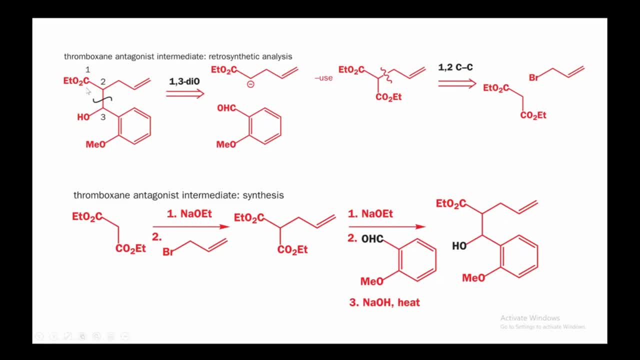 so what happens here? you disconnect the bond between two and three. so the disconnection gives you the negative charge on the carbon number two and the aldehyde carbon number three will become aldehyde. and now you are reacting this, attaching another ester group, and then this is a simple alkylation reaction. and then this is a simple alkylation reaction, and then this is a simple alkylation reaction. 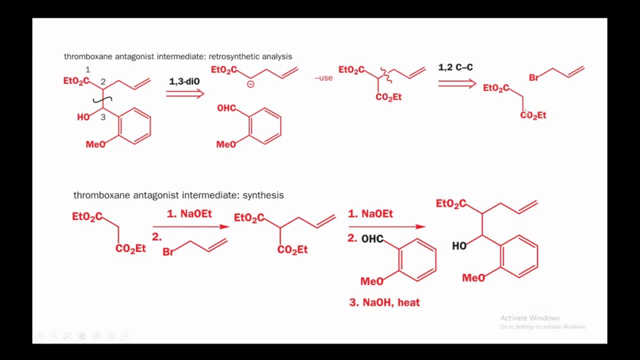 reaction. so you delete this alkyl reaction and then you have a one three ester linkage. now you are reacting this one three ester linkage with this and sodium ethoxide will generate a negative charge here and this negative charge will take on this carbon and then bromine will leave. you will get this. 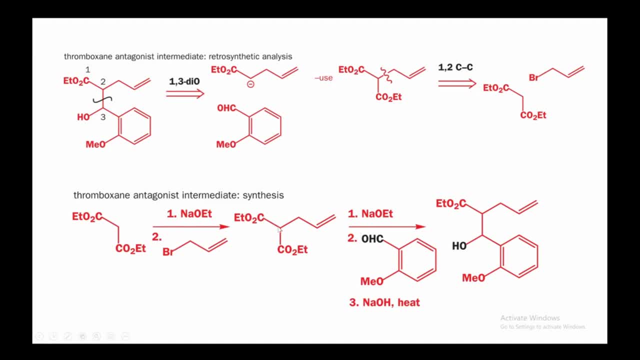 compound. now, sodium ethoxide will generate a negative charge at this position which will react with this aldehyde to give you the one three di carbonyl compounds and you can remove the extra ester group by using sodium hydroxide and heating. that's how you can prepare this compound. another example: 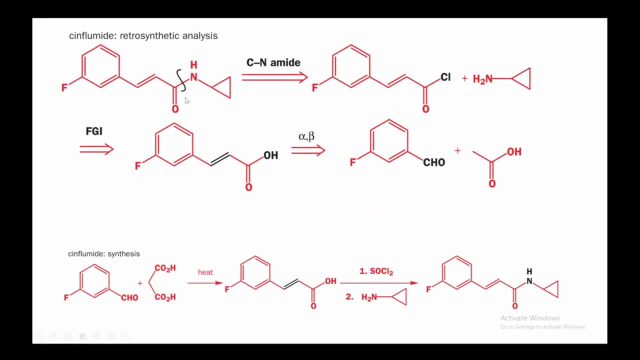 of alpha beta unsaturated compounds. but this time we have to first convert amide into your. this is amide functionality will disconnect between C and bond. you get the acid chloride and in the next step we convert acid chloride into carboxylic acids. now you have a carbonyl alpha beta unsaturated. you disconnect. 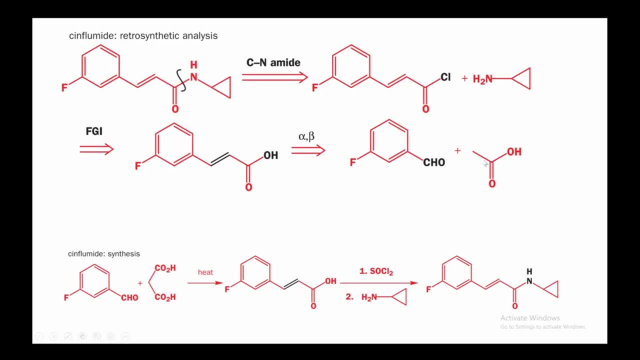 one side becomes aldehyde, another side becomes acetate. so in order to activate this acid, will add another acid to make it active with lean compound. then generate a negative charge here and this aldehyde to give you this linkage and heat the compound to remove extra acid. then in the next step you are converting acid using 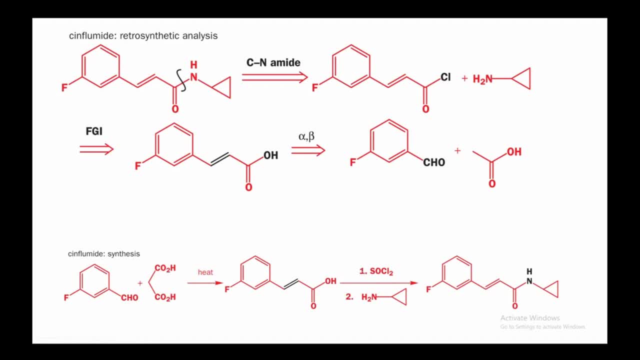 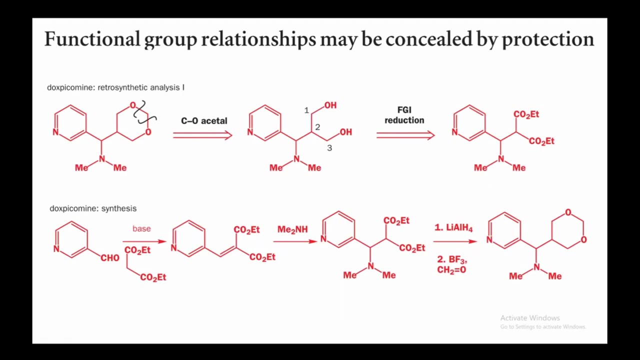 pinocloid into chlorine and then you have acid chloride. now you are reacting this acid chloride with this primary. I mean to give you the desired target molecule example. this is a functional group relationship may be concealed by protection, so sometimes we have a protection in such as in this case. so 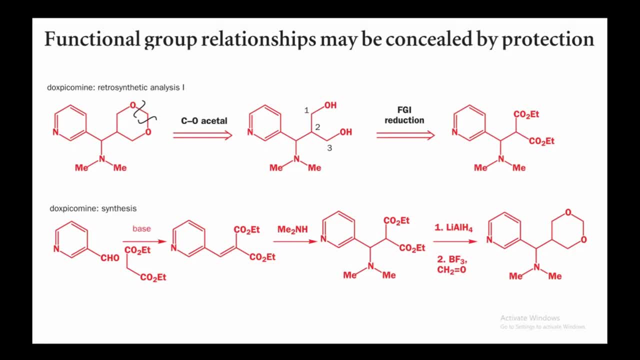 that you can have this, the ester linkage of this compound, and sometimes then you disconnect the CO acetol linkage, then you generate diodes. that is one, two, three functionalities and now you can do FDI reduction, you convert alcohols into esters and then you can convert this compound into the simple starting. 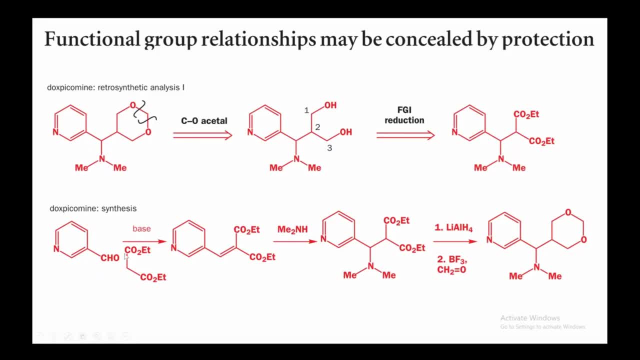 materials by disconnecting from this position. so you react this compound with aldehyde, and this in the presence of base to generate positive charge. then this primary is a secondary, direct with this Michael acceptor to give you this, and in the next step you reduce esters into alcohol. 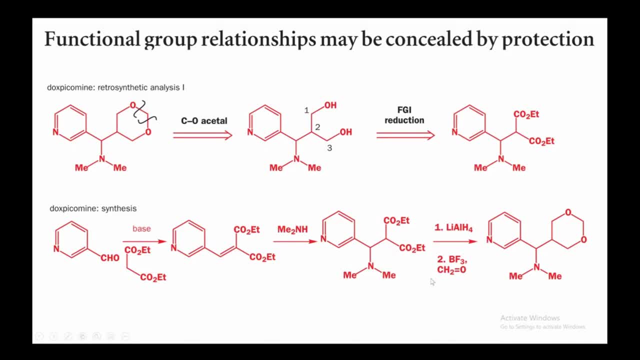 then you protect those alcohols with acetols using formaldehyde. so this, how you can use a protecting group is 30 D for this sort of functional groups. okay, let's have a look at the next example. so this is 1, 2, 3 relationship. so you 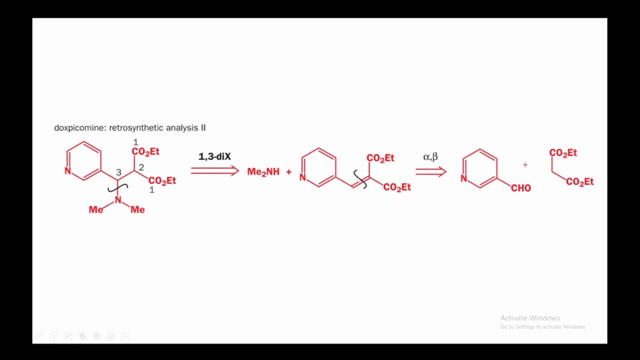 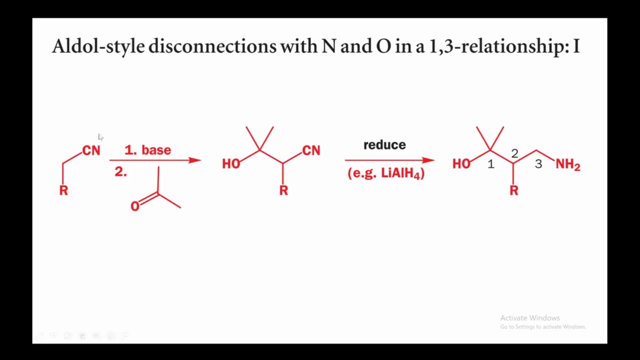 disconnected from here, you get the positive charge here and then you generate a alpha beta unsaturated situation and the one side becomes aldehyde and another is actinicline. okay, let's go on to the aldol disconnections with N and O in a 1-3 relationship. so you react with alpha. 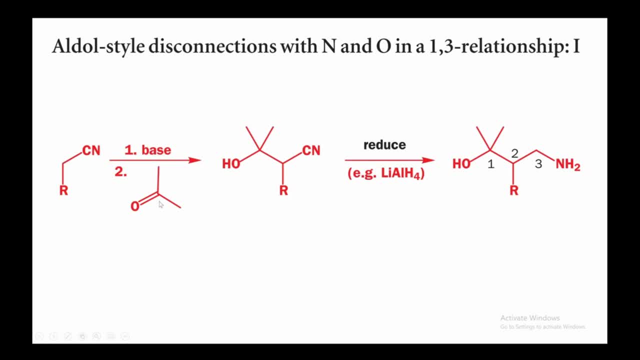 cyano compounds in the presence of base. with acetone or aldehyde or ketone, you generate a cyano alcohol compounds. then you reduce cyanide into NH2. now you have a relationship between amine and alcohol that is a parted by three functional groups. now next we will apply this concept into the molecules. before that, 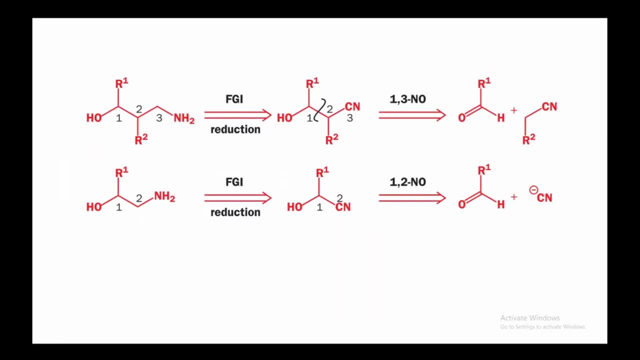 we need to understand more strategies. so this is a 1- 2- 3 relationship between amine and alcohol. so what you need to do is FGI reduction to make them closer. so you convert NH2 into cyanide and then you disconnect the bond between 1 and 2. 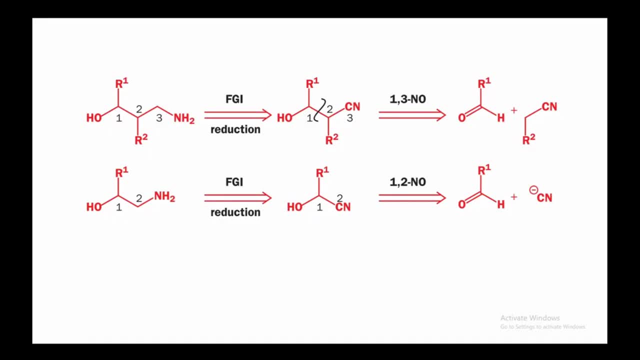 then you will, sorry, sorry, aldehyde and cyano compound. now in the next step you do the FGI reduction. then you have cyanide at the position 2. now you are doing disconnection, that is, from between 1 and 2, and the cyanide gets the negative. 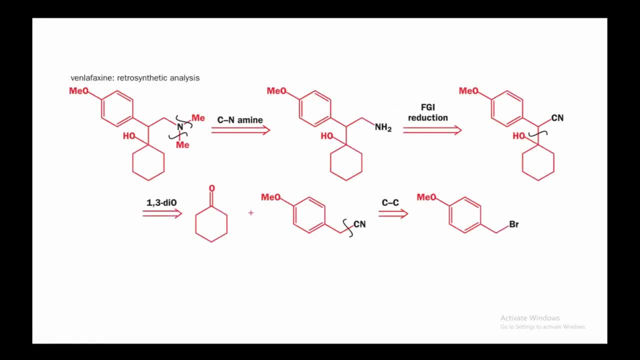 charge in the aldehyde. so then you have at this example where you are disconnecting the two methyl groups attached with this nitrogen, that becomes NH2, that is C and amine disconnection, and next step is FGI reduction, that is, you are converting NH2 into cyanide and then you have a 1, 2, 3 relationship between cyanide and alcohol. 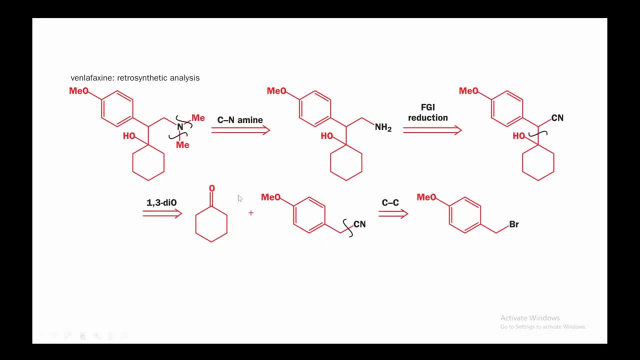 you are disconnecting the bond between carbon and carbon. that is called 1: 3 disconnection- and you have a simple cyclohexanone and this is a cyanide. further, you can using disconnection, you are converting cyanide into alkyl halide or a benzoyl halide. 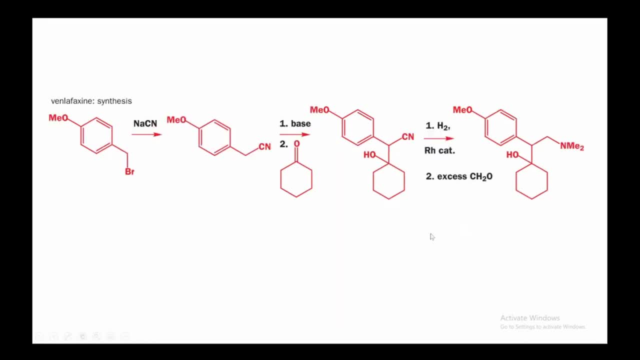 you simply do do the SN2 reaction, sodium C will stay in the Ronnie Integrosur and C will stay in N2. the sodium C will stay in the Viel attacks on this carbon and SN2 are generating this compound and, in the presence of base, you are. 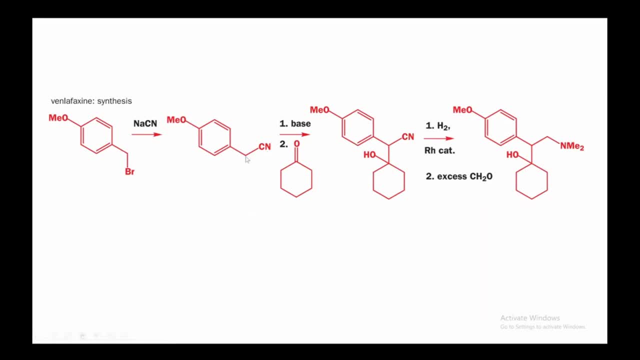 generating the negative charge on the alpha carbon of cyanide, and this negative charge attacks on this ketone to give you this functionality and in this you can reduce the cyanide into this compound and by reacting further with excess of formaldehyde you can generate the methyls on the 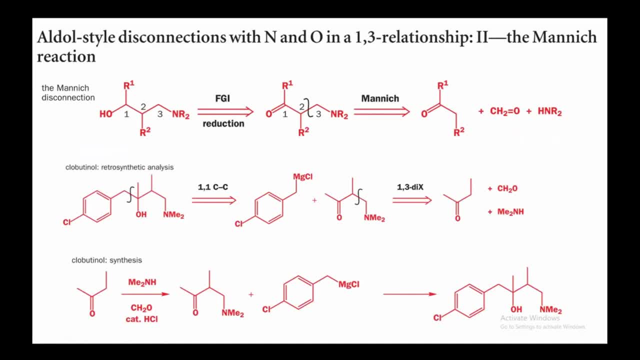 nitrogen. okay, let's do another manic type study, that's aldolio style disconnections with nitrogen and oxygen in a 1-3 relationship, type 2. the manic reaction, so that's a relationship of amine and alcohol, that is, distance between two functional group, is 1-3. so you do fgi reduction and then you 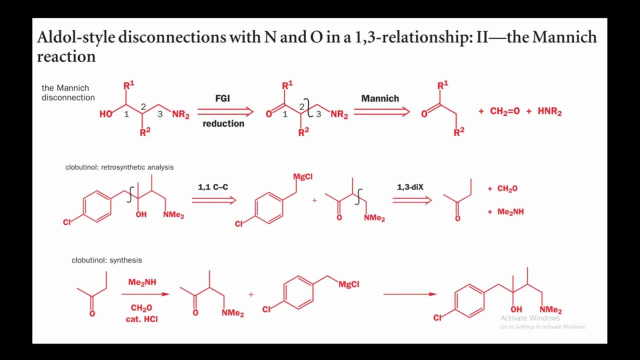 convert and this alcohol into ketone. then you disconnect the bond between 2 and 3 so that you can mix all of these reagents like ketone formic acid. and then you can mix all of these reagents like ketone formic acid and then you 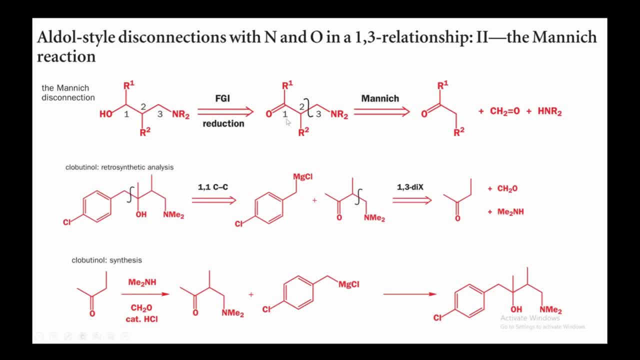 formaldehyde and this amine to give you this compound. and then you do reduction of this ketone to give you the alcohol. so apply this strategy to this compound so you have this 1-2-3 relationship between amine and alcohol. so you disconnect this alkyl chain- 1cc disconnection- this alcohol is 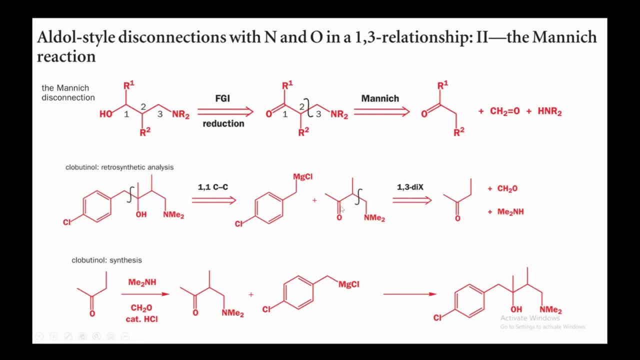 magnesium chloride, ketone reagent. this becomes ketone. now you can disconnect from this position. that is carbon, carbon bond disconnection and the relationship is 1-3 disconnection and it's a manic type reaction. so you react this ketone with this secondary amine, formaldehyde, in the 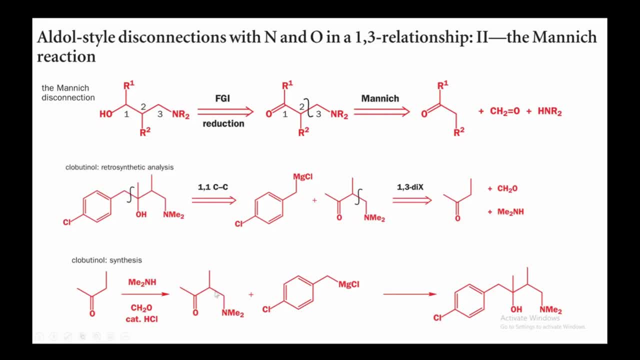 presence of hcl to generate this manic reagent that contains ketone, and then you react this ketone with magnesium chloride containing grignard reagent to give you this alcohol. so that's how you can prepare this compound, using manic type reaction. this is a strategy that you need to follow in big 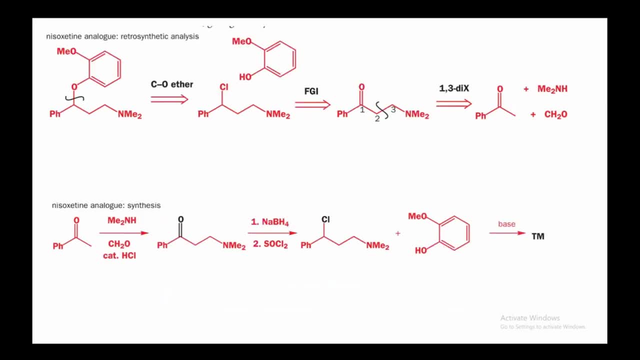 molecules at different artificial compounds. okay, let's again follow the strategy. this is a ether linkage, so we are disconnecting co ether bond and one side you are getting alcohol, like phenol in this case, and another side you are getting alkyl halide. so what you do is do fgi, so you convert. 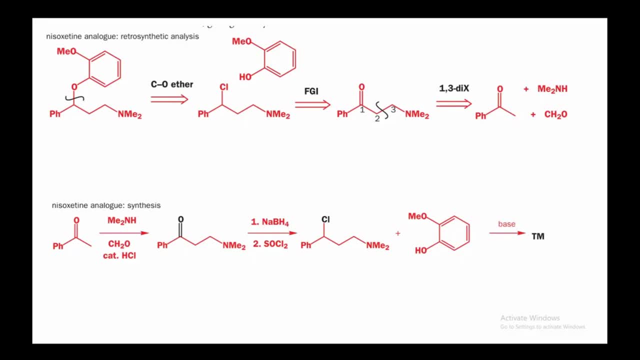 chlorine into oh and then you do oxidation of oh to convert it into ketone. that's called fgi. now you are disconnecting between these two compounds and then you are getting alcohol like two and three by manic type reaction. then you mix up these things to give you 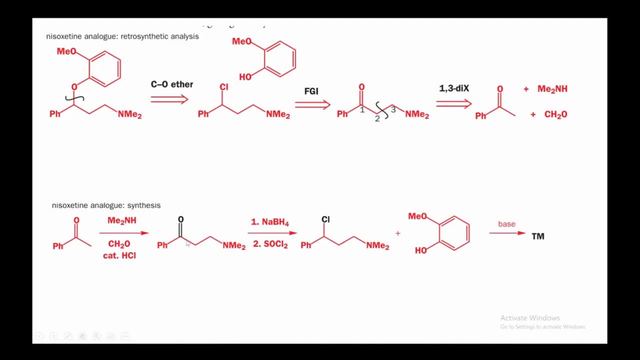 this compound. then you reduce this ketone into alcohol, then react it with hyaluronide. it gives you the chlorine. now you are reacting this chlorine with this OH of phenol in the presence of base to give you the target molecule. so that's the story, how you can follow this approach for generating the target. 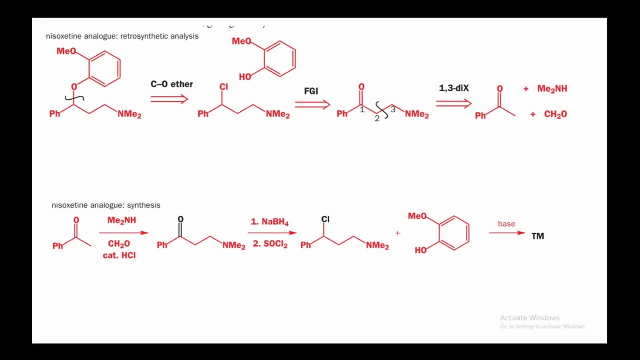 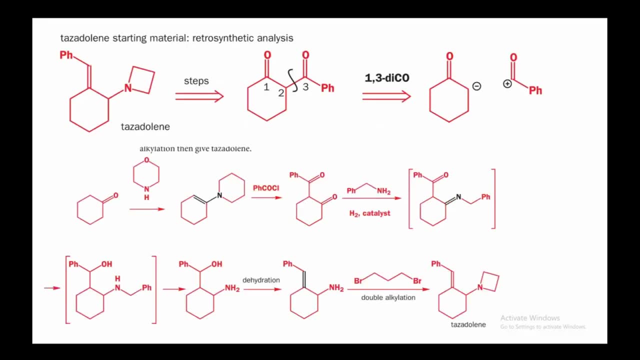 compounds are preparing the starting materials and then constructing the synthesis towards the big target compound. okay, let's move on. if you are given this kind of a strategy, if you look at this example again, this is a 1: 3 dicarbonyl compound relationship. so you disconnect between 2 & 3, the one 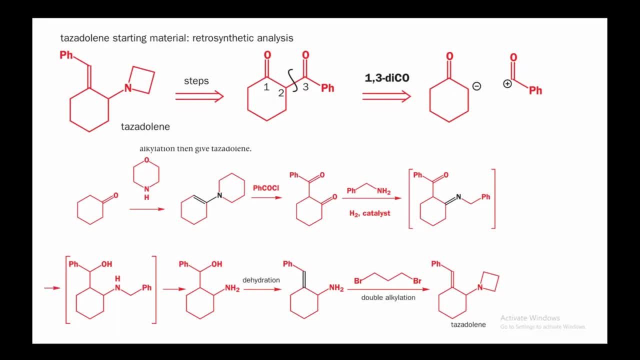 side gets a negative charge and the other side gets the positive charge. so what you can do is you can apply in amine synthetic strategy for these sort of compounds and then you can use this strategy to generate the base to give you compounds, that is, 1, 3 dicarbonyl compounds. so you first react with this. 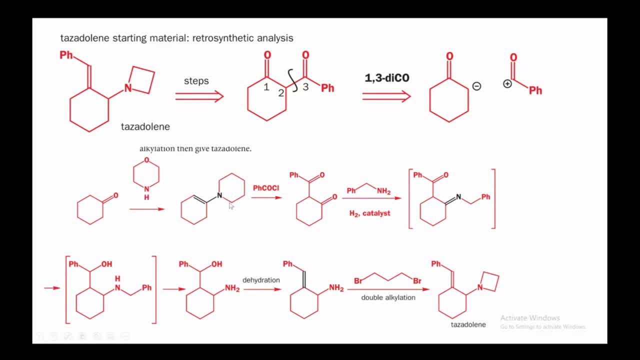 ketone with any amine- secondary amine, to generate an in amine, and then you react this with acid chloride to generate this compound and in the next step, you react this with primary amine, which will react with this ketone, and then you can use. 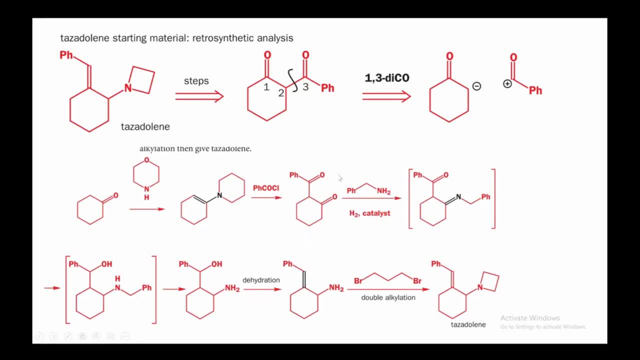 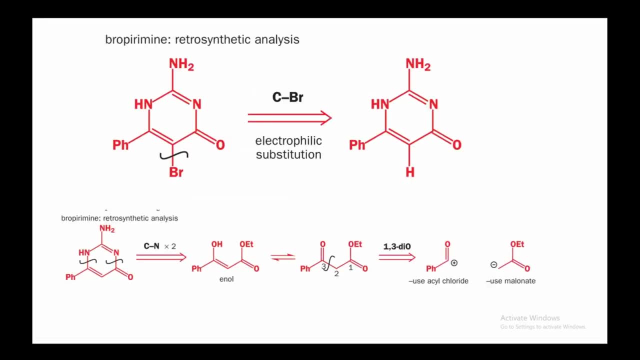 H2 catalyst to reduce this compound, to generate the, this product. that's called the in amine strategy for 1: 3 dicarbonyl compounds. if you look at this example, you can delete this bromine- that's a CBR electrophilic substitution reaction- and then you can disconnect these 2. 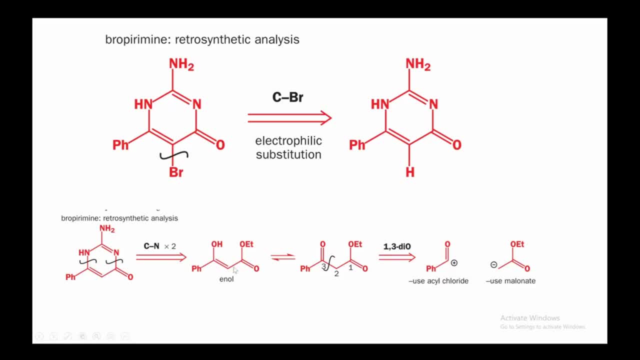 cyanide, carbon-autogen bonds, you generate a enol and then you have 1, 3 dicarbonyl compounds. you can disconnect it and you have these synthones and which are equivalent to this one's. so if you have this situation where you have 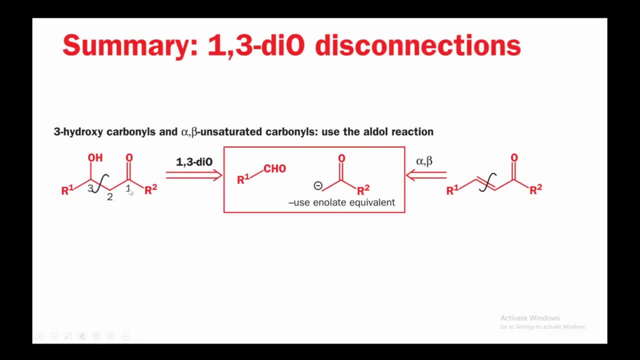 alcohol on position 3 and carbonyl on 1. you disconnect from position 2 and 3 in the opposite direction, two and three, you will generate these sort of synthetic equivalents which is exactly similar to alpha beta unsaturated. if you disconnect this position, you will have these symptoms easy. so you try to remember this summary. 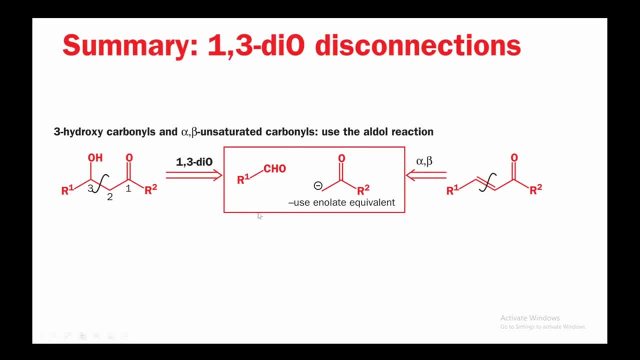 in your mind and the relationship of the functional groups though, so that you can apply this concept for this sort of compounds. this is a manic reaction strategy. if you have a relationship between one and three and you have a nucleophile at position three, you can disconnect from two and three and you 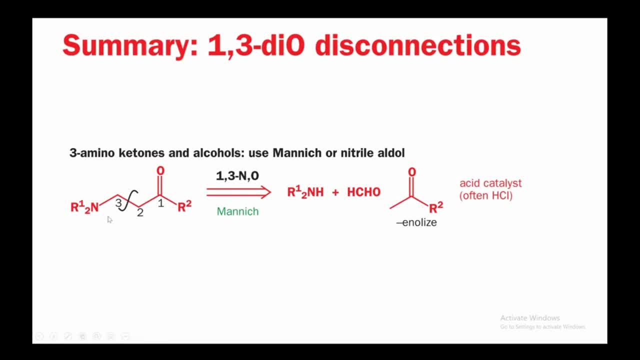 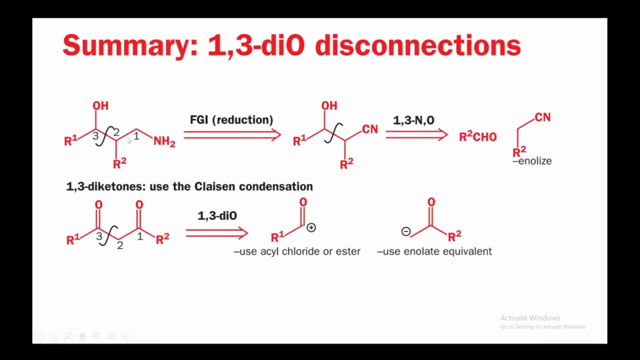 have a simply starting materials and you combine them, you will get this region. another reaction was one relationship between amines and alcohols. amines and alcohols. you do FGI, you convert NH2 into cyanide and then you disconnect between the cyanide and alcohol into these simple molecules and then you have one. 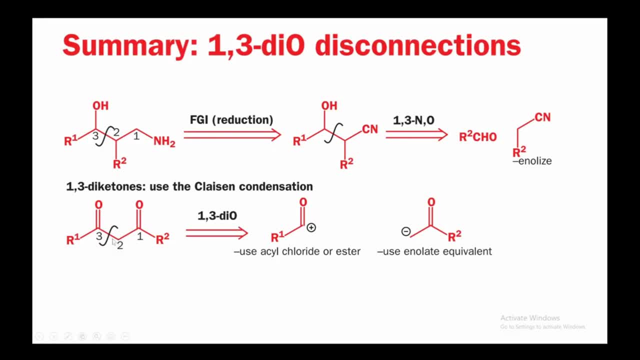 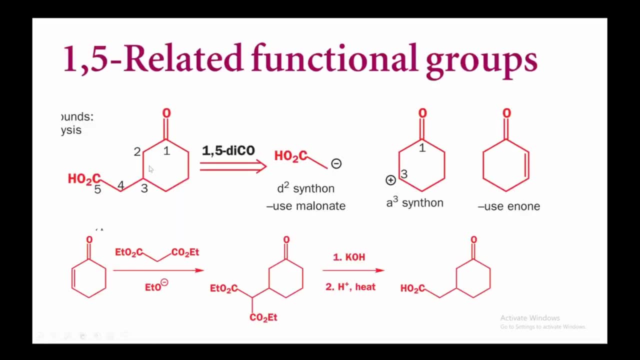 three diketones. use the glation condensation you disconnect between two and three to generate these phenols, centons. how about one five disconnections? so in one? in case of one five disconnection, you can disconnect it from position three and four and you will get a positive charge on three which will be equivalent to this. 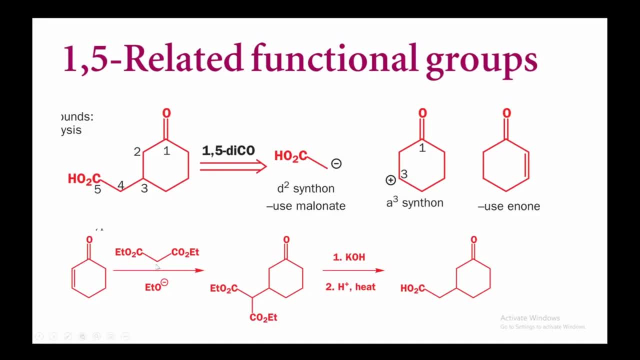 centon. now you are reacting this enone with this active methylene compound in the presence of base to get this, and then, in the next step, you are converting, hydrolyzing one of the ester into acid, and then you are removing the ester using acid and heat to generate the positive target compounds. 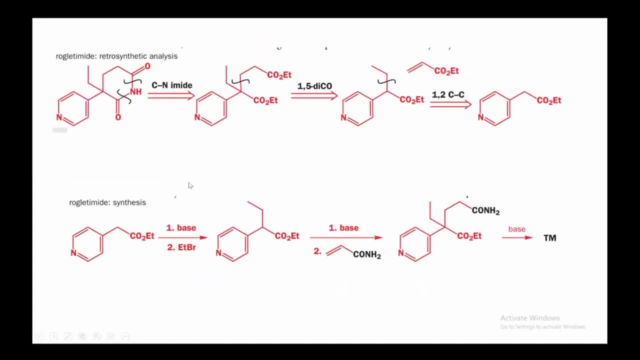 this is a one five di functional compound that you can prepare this away. next is this: is see an amide bond disconnection because the cyclic amide, so you disconnect it and then you generate a one five di carbon compounds. then it's an alkylation one five disconnection. you can disconnect it from this position. the 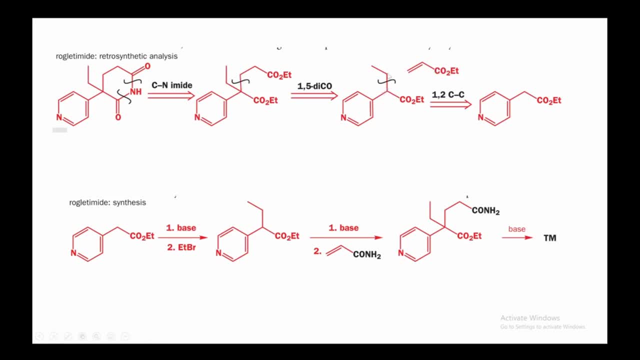 one becomes a Michael acceptor and this is alkyl group. we disconnect it and you can start from the simple historic material. what happens is you have alpha position of this ester, which base picks proton from this position and attacks on the ethyl bromide and you generate this compound and, in the next step, the base. 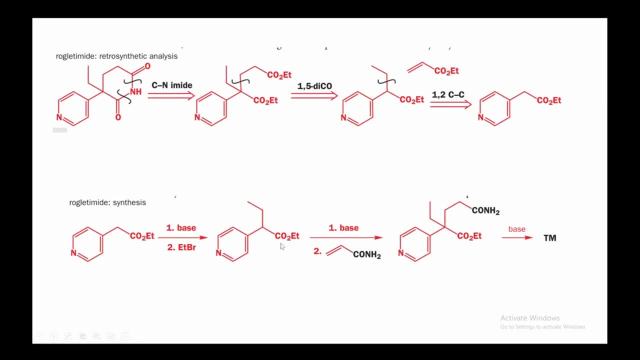 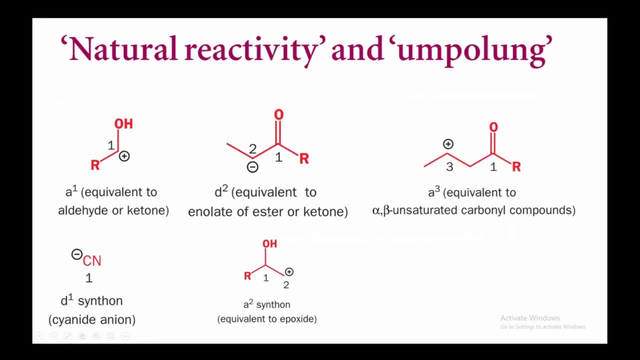 reacts with this compound, generate a negative charge and this attacks on this compound. to give you this, and in the presence of base, you get the target molecule. this was the natural reactivity and I'm pulling is the reversal of polarity. so you generate positive charge. in the appalling, you convert this. 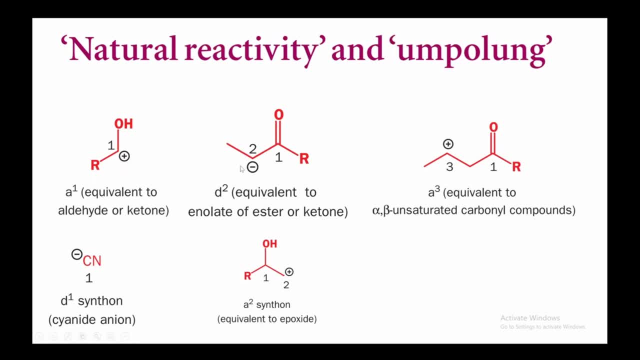 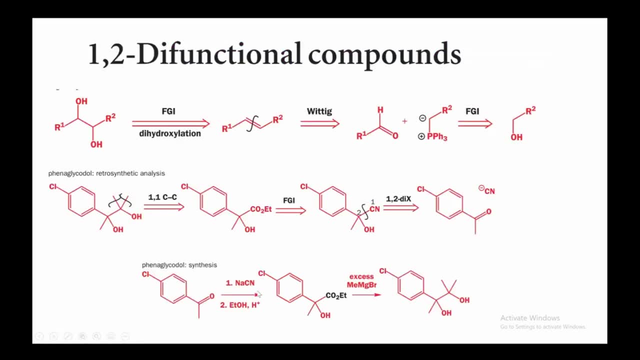 positive charge into negative charge. so the a1 centon, this is a2, sorry, d2, and this is a3 and this is d1 and this is a a2 centons. so one, two di functional compounds, so this is diols. so do fgi dihydroxylation: you convert diols into 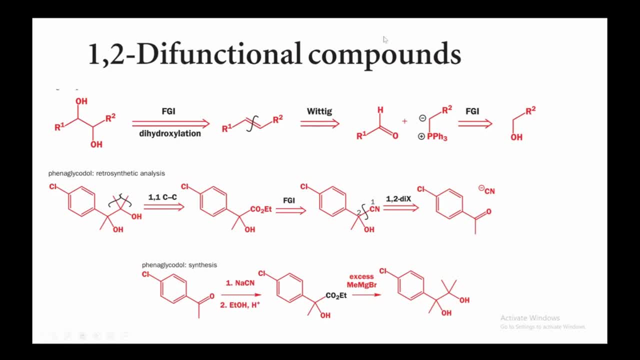 alkenes, then do wittig reaction and you have a elid and aldehyde and then do fgi. that you gave you the alcohol. now this is alcohol. so you disconnect from two methyl groups. you generate aspr here. remember this is a tertiary alcohol and two 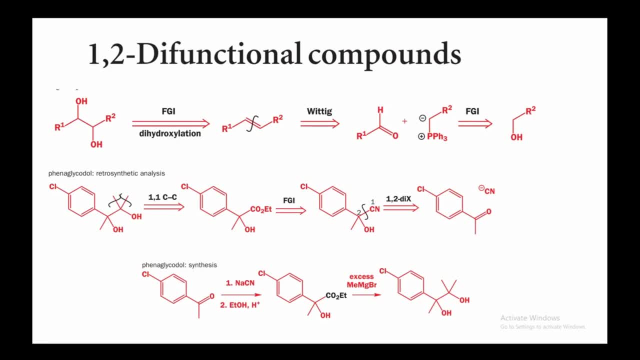 metals are symmetrical, so there's a relationship of a sterile connected. here we are, naszych q, approval, sizin one, two, and then you can work, asking the cyanide, then the disconnect, cyanide, character, identity or not, where it decides to keep on and in the presence. 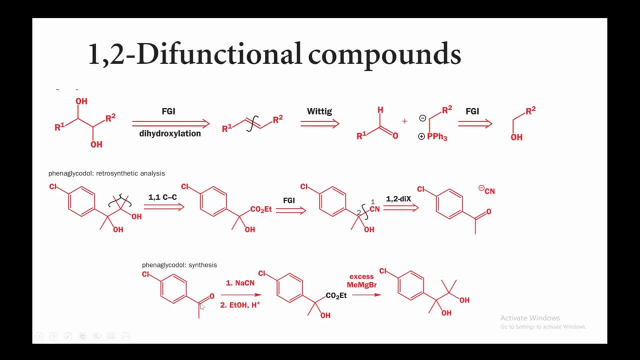 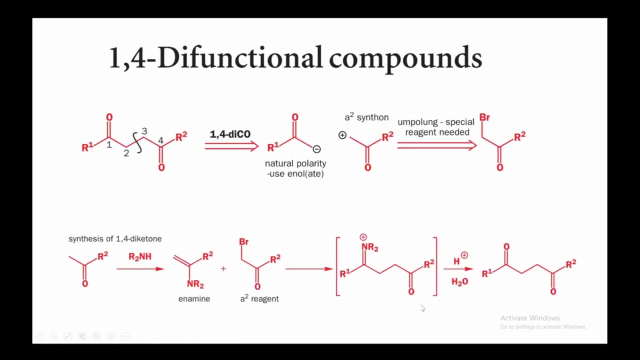 of ethanol, so he forget the alcohol and cyanide. and then cyanide is the high into acid which is then reacting with ethanol to give you the ester. then you react this ester with excess methylmagnesium bromide to give you the diols. that is for 1,2-diefunctional compounds. this is a 1,4-diefunctional. 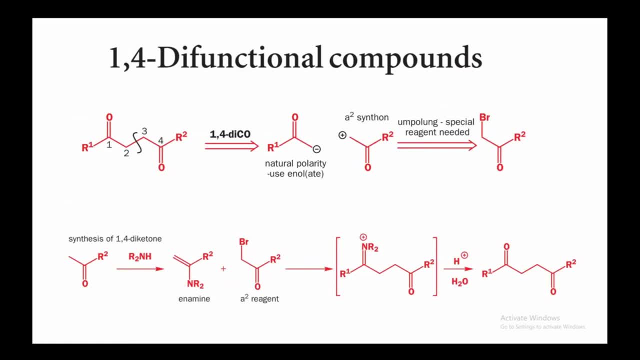 compounds. it's a very tricky reaction. so you disconnect from position two and three. you generate a negative charge and a positive charge, both on the alpha carbon. so you put the bromine where the positive charge is and you use the end-amine strategy for the negative charge to make it a more nucleophilic. 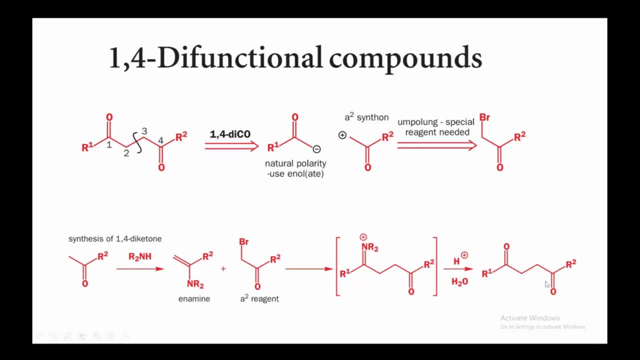 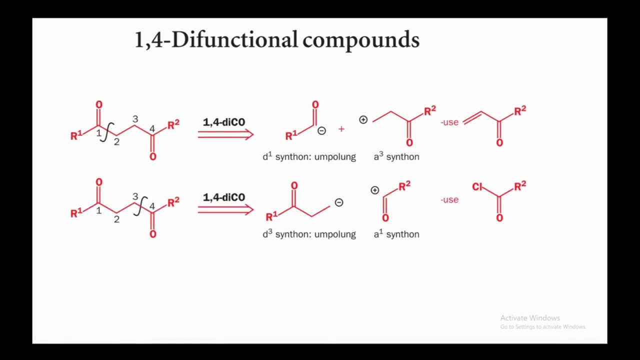 and in this way you can generate the 1,4-diefunctional compounds. but here is a summary for 1,4-diefunctional compounds. you in this previous example you disconnected from two and three position. here you can disconnect from one and two. in that case you get a. 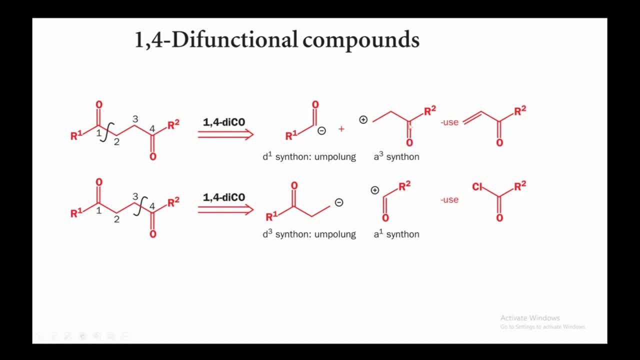 negative charge of this carbon and the positive charge and the synthetic equivalent for this positive splined. its also my好的 pulsating the star. it's very difficult to follow this path. so you select lessiс settings and slightly positive charge is the Michael acceptor and also you can disconnect from position three and four. 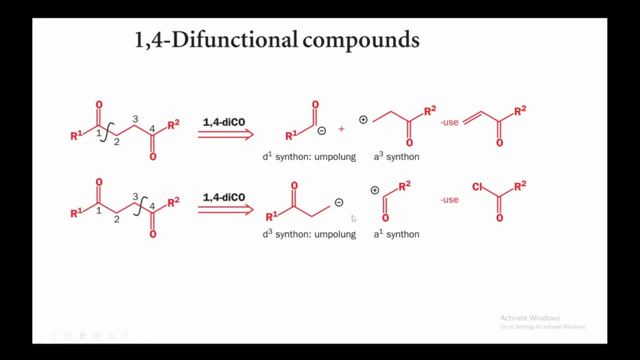 for one four dicharbonic compounds and you get a negative charge on this carbon and a positive charge on this, and for this positive charge you can use this acid chloride as a synthetic equivalent of which is reagent. so let's apply this study to this real example. so now you are. 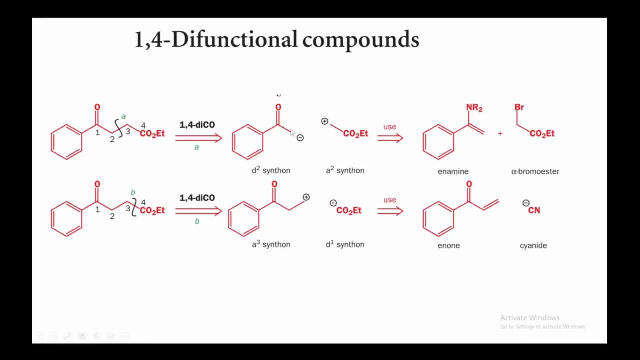 disconnecting from two and three, you are generating a negative charge on this alpha position and a positive charge on this carbon, so you can use the in amine route. and here you are disconnecting from three and four. you are generating a positive charge and negative charge here, so you can. 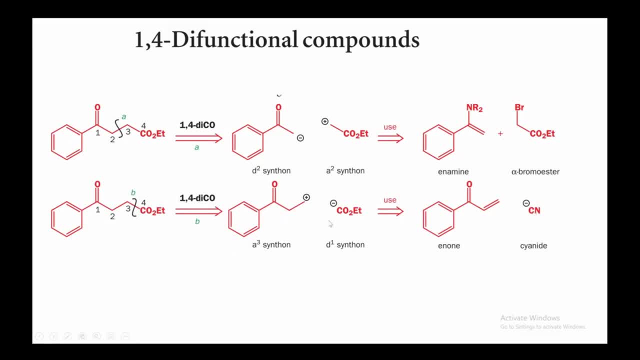 generate in a d1 synthone, which is cyanide, and the positive charge here that is Michael acceptor enone. this is again a one four disconnection and you can directly use the Friedel-Croft acylation. but you need to do first fgi- convert ester into acid- and then you 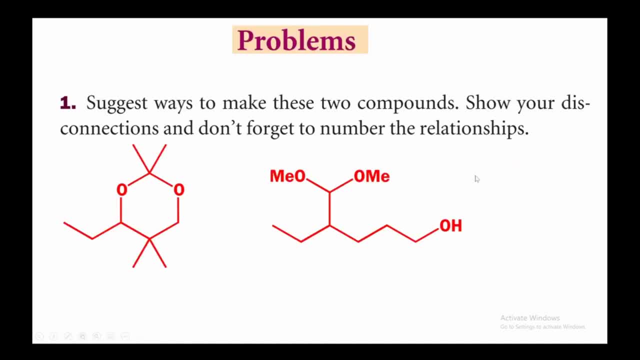 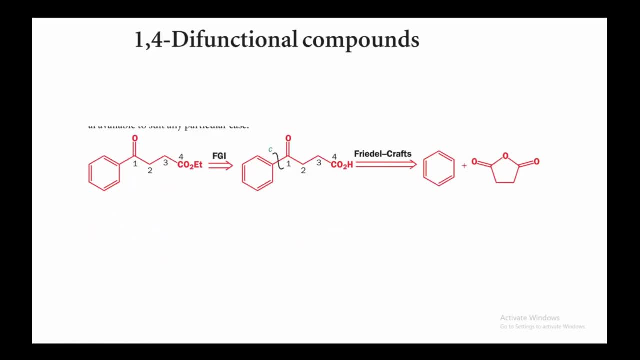 disconnect from two and four and you can generate a positive charge on this carbon. this connected in this intramolecular reaction. this was the chapter of cladding that I described in this long video. sorry for making a long video, but someone asked me to make a very big video about right to synthesis. I will make two more big videos to lectures on. 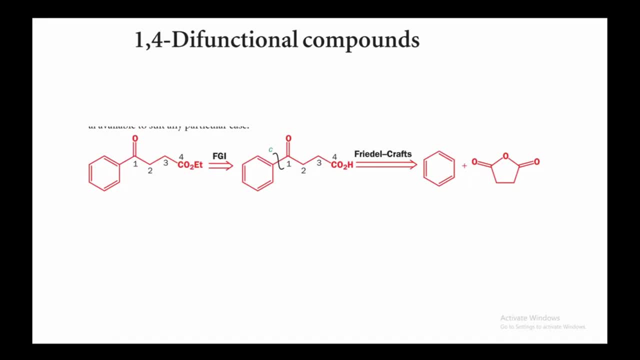 retrosynthesis from two different books and, after those two videos, that will be the end of the rate of synthesis and you will be master if you clearly listen. what I have mentioned in this video- and I will make more videos about this- and this was. this video was taken from the Pleiadian organic chemistry book, chapter 30, and I 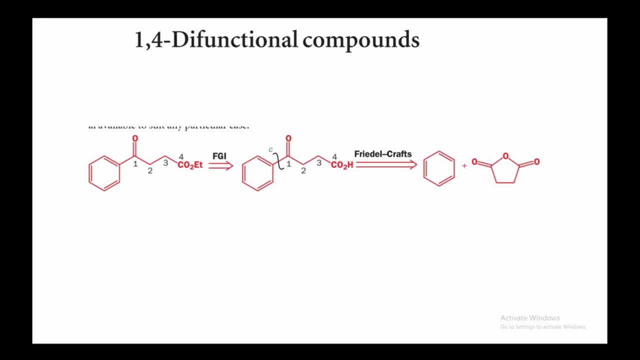 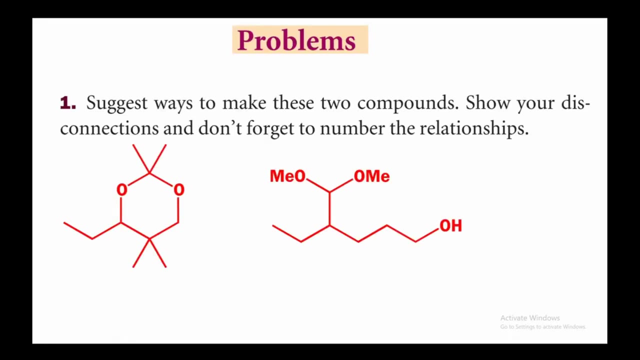 made this video. if you don't understand any molecule retrosynthesis from this video lecture, please drop your questions in the comments of this video on the YouTube. I will try to answer and I am NOT solving the exercise. I am leaving this to you to solve this exercise of Pleiadian. this is a problem number one. 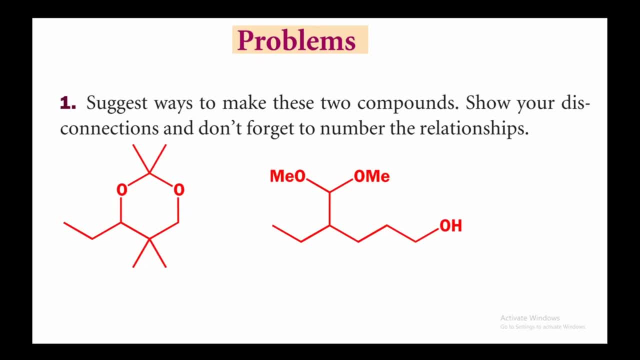 but if you are unable to solve the exercise, please ask me in the comments of the YouTube. then I will try to make another video where I will solve these problems for you. but I hope that if you have understood the video about the retrosynthesis whole chapter, you should be able to solve these problems by